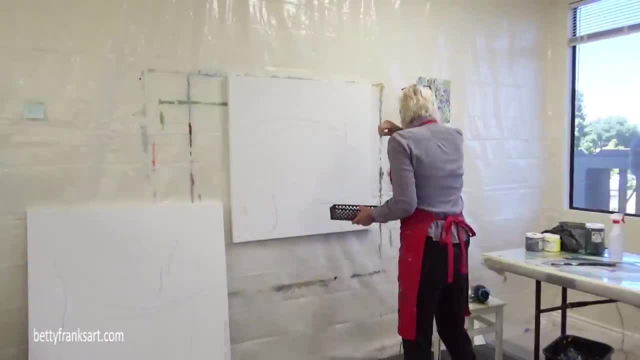 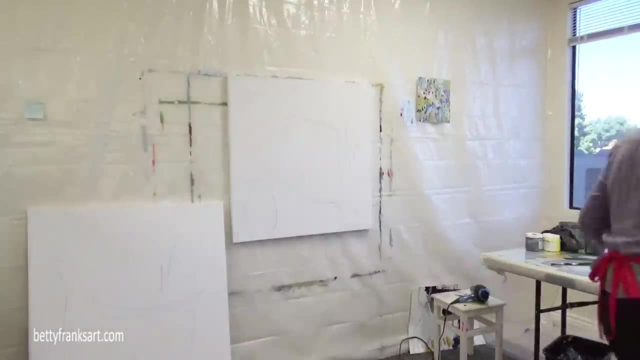 And that's because I don't have enough screws going across my wall and I need to fix that so that I can put two of them up at once, Kind of like I used to do in my old studio. I had quite a few screws going all the way across. Now, in my old studio there were studs in the 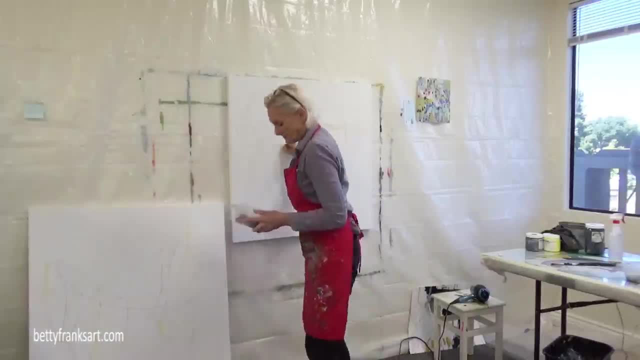 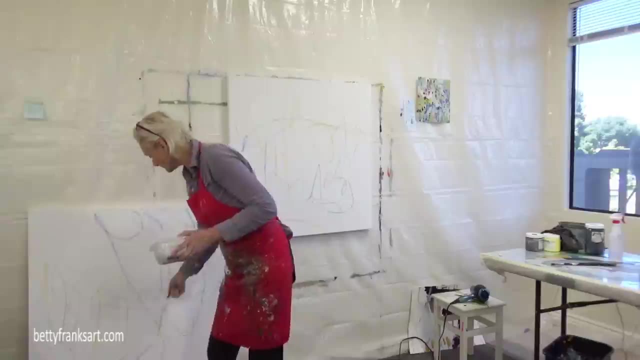 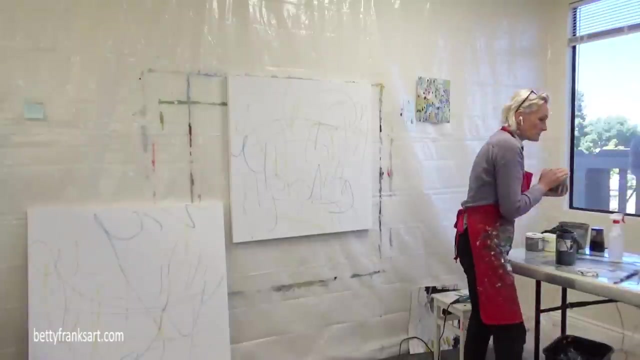 walls, So actual wood studs in the walls. What's interesting in this building? this is a really old building and for some reason there are no studs in the walls. There's metal studs, So I'm still trying to figure out the best way to get screws in there. The maintenance: 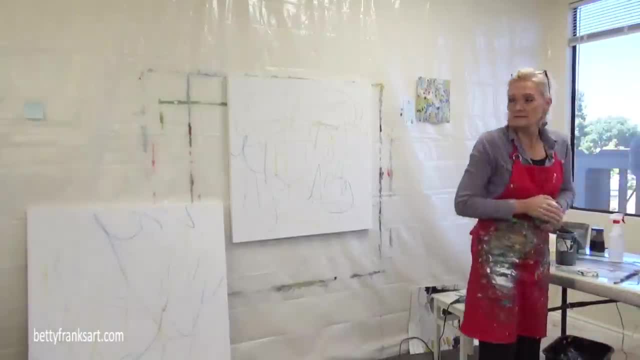 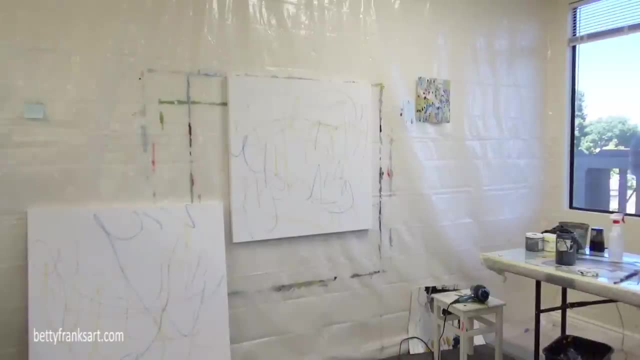 company that runs the place put these screws in the wall for me, but they're not sturdy. They're already falling downward. So I'm kind of annoyed with that right now. So I purchased. let's see, where did I purchase? Oh man, I can't remember the name of them, But anyway, it's something where. 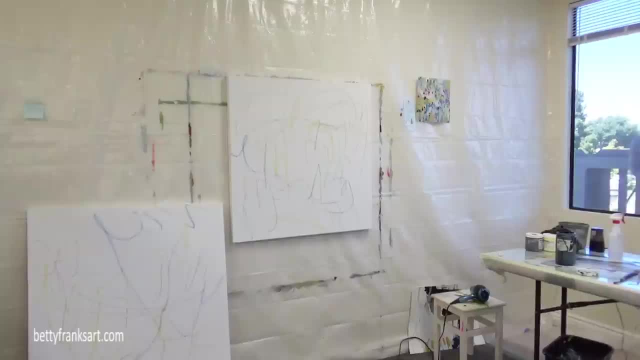 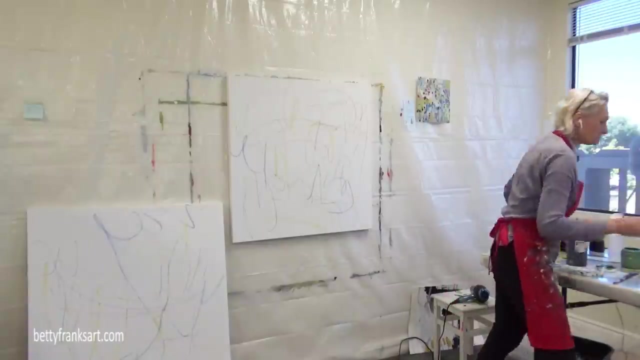 when you can't put a screw in the wall because you don't have a stud. so it's something that will help secure that screw so it stays in place- An anchor, That's it. I think it's an anchor, And I was being a little annoyed over there because I was looking for that one tool. 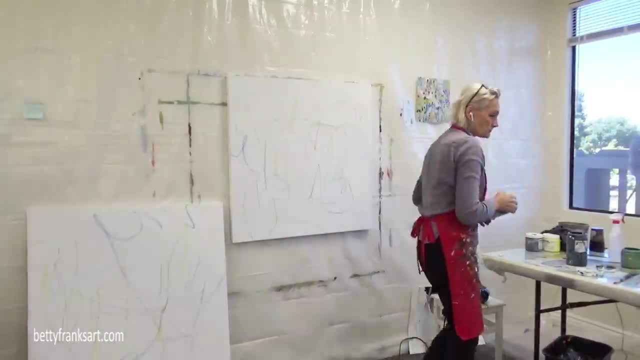 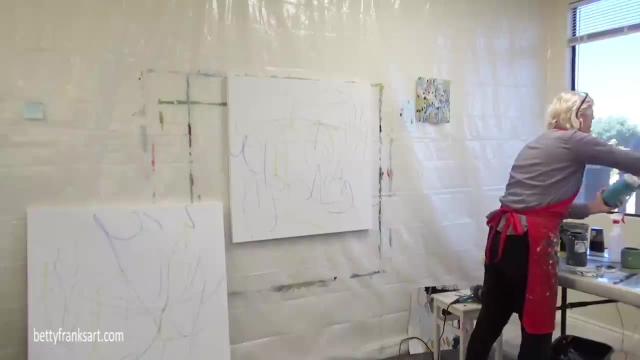 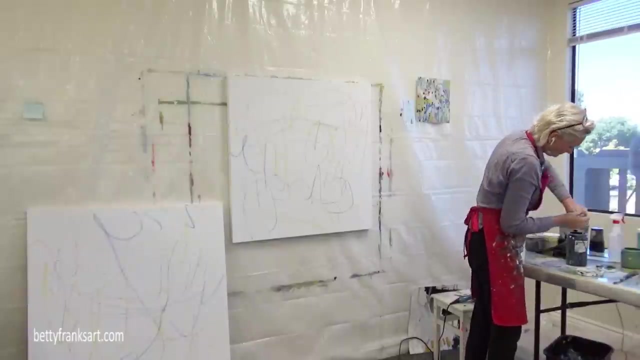 that I have to whack the side of my jars so that I can get them open. This video was taken shortly after I moved into my new studio. As you could tell, there's only a couple of outlines of previous canvases up on the wall, And what I'm doing right now is I have a jar with some black in it, And what? 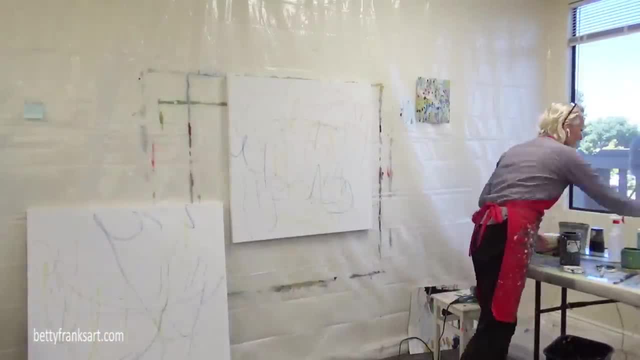 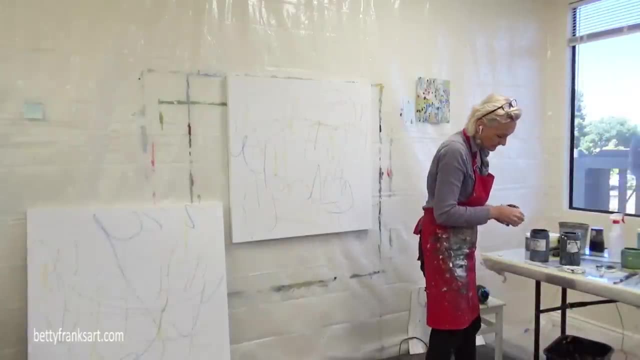 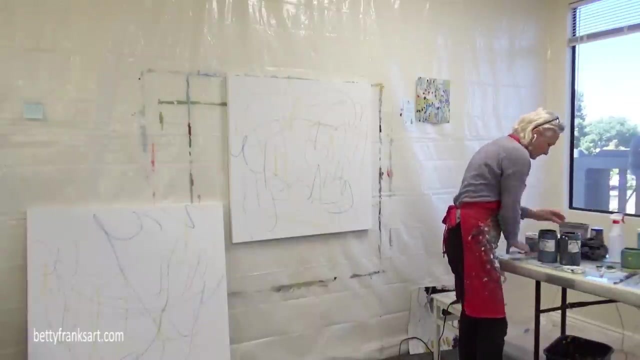 I like doing is I like adding other colors to it to really deepen that black and not just a pure black out of the jar, but a more complex black. And the way I do that is I just add a variety of different colors to the black and I just mix all that up. So that's what I'm doing here And I'm 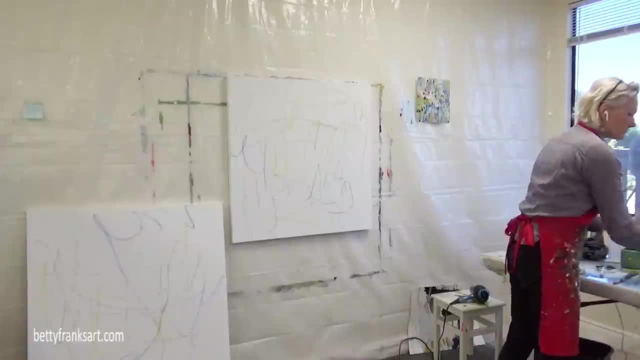 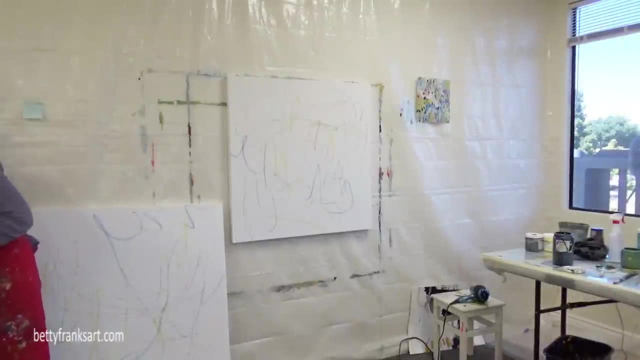 just searching. I've got a shelf over off to the left side of the screen there with a number of different jars And I'm trying to grab a few to bring over And I'm trying to use up some of my, my jars of paint that. 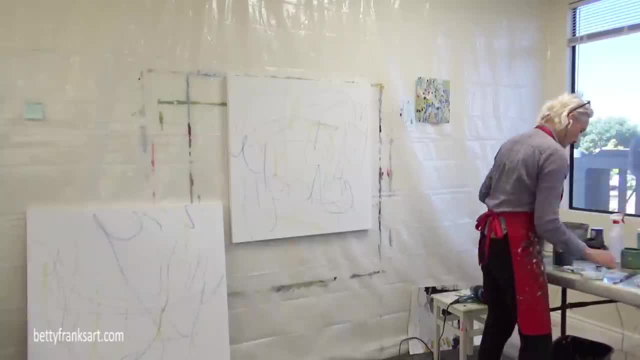 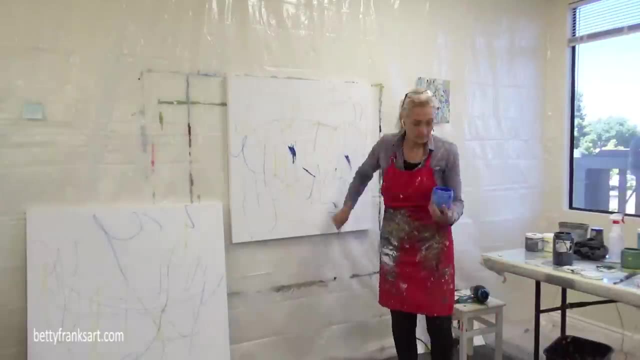 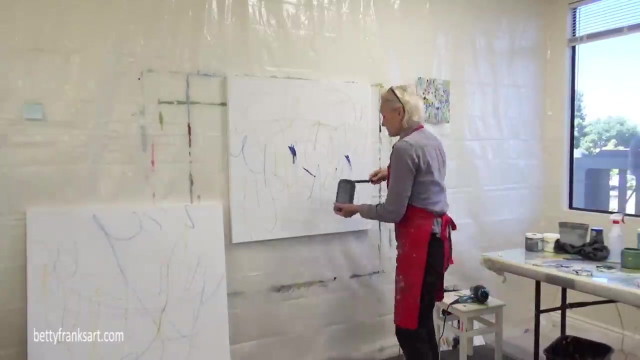 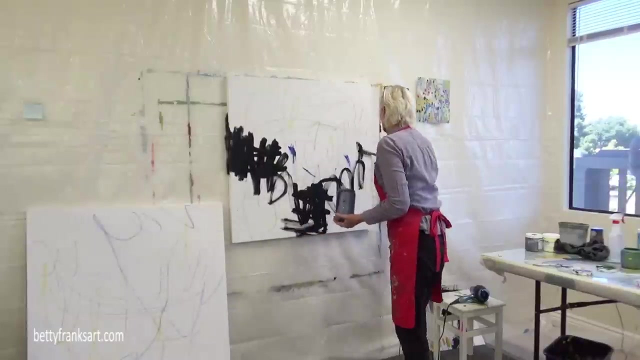 are starting to get old. I think the most tragic thing is to have jars of paint that have dried up as opposed to using it up In some way, such as getting it up on a canvas. There we go. So from here you can't tell that it's a more complex black, but up close you know I can. 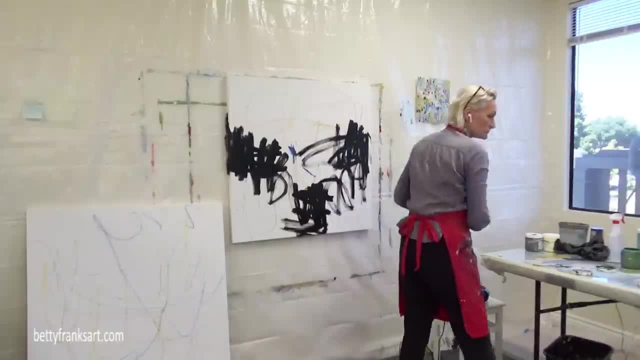 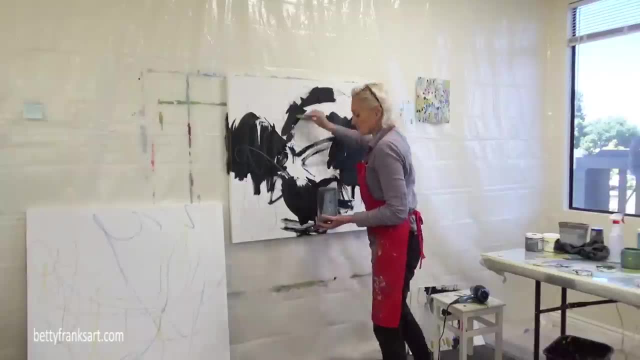 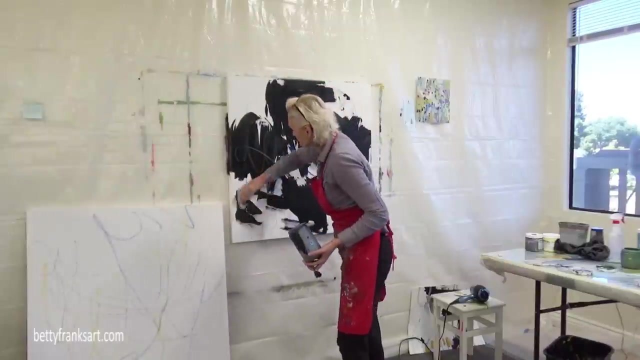 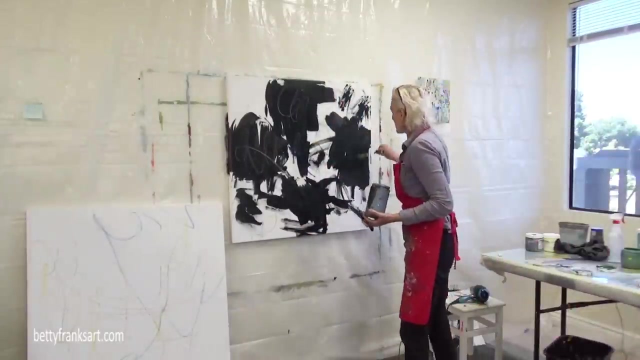 definitely tell. Now I'm using a scraper here just to move that paint around, more so than I usually do with with my paint brush, Doing something a little bit different. You know, normally I would just use a paintbrush at this point, But I decided to do something a little bit different And I'm scratching right into that. 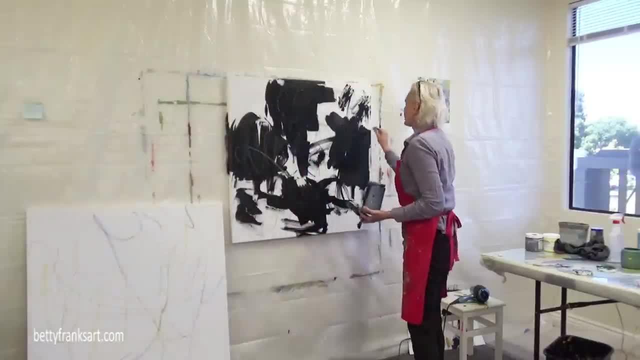 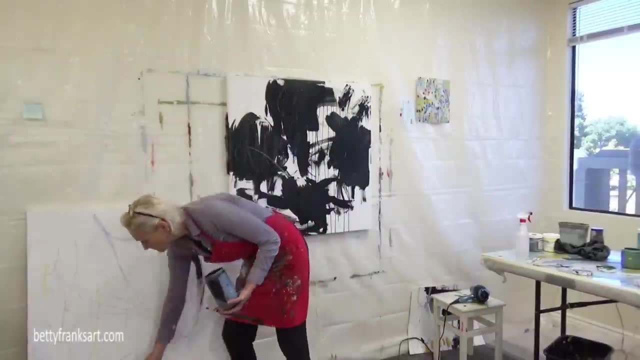 black to start adding some texture to the painting. I'm going great for drips as well. OK, that frees up some time for me to work on the other one, And we can't quite see the bottom of it, But I think you'll get the gist of it later on. One of these I continue to work on and the other one I set aside, But I do have a video. I do have a video now and I have all the shows I have in there. There's a lot of resources- Even One of these I continue to work on and the other one I set aside, But I do have a video now. There'sBA still a lot of questions about how to work with either one, but I overwrite them, but sometimes I speed up, stir it up. 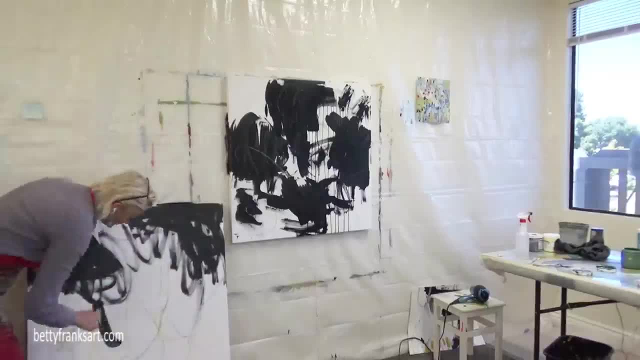 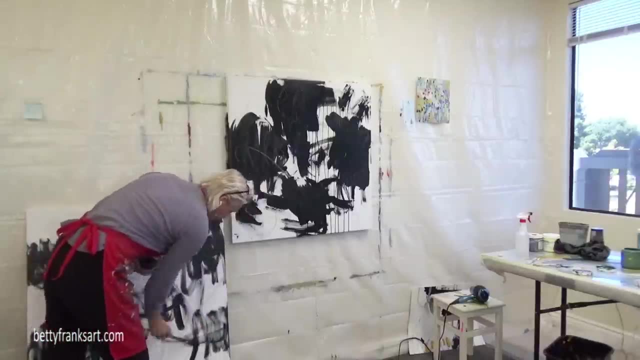 But my almost favorite stuff to try on right now is pink, but my favorite is video of that one as well, Or I should say I will have a video of that one. I haven't put it together yet, but I do have it prepped and ready for me to do a voiceover on it. 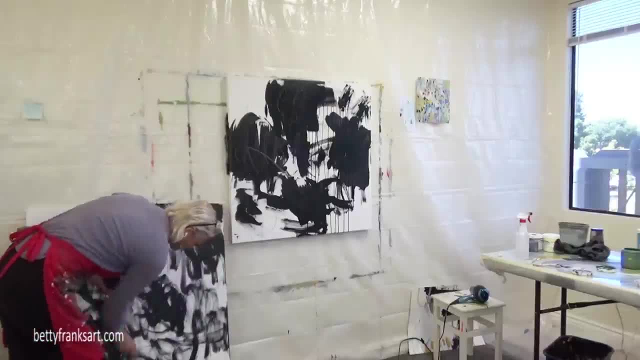 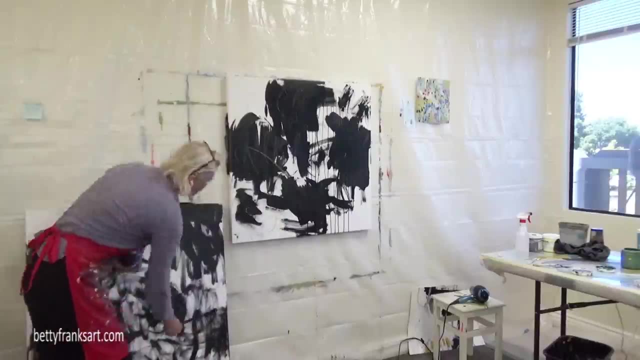 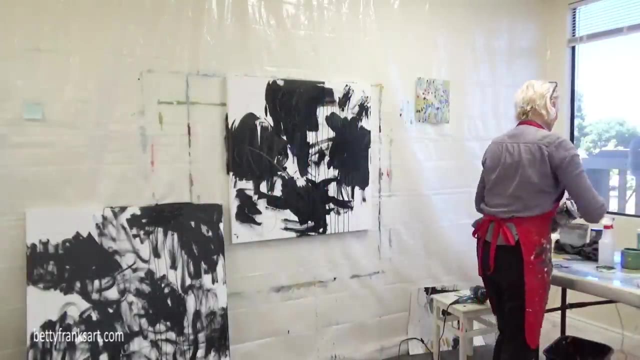 Again, I want to say welcome If you've been following me for a while, thank you, thank you, thank you. I so appreciate you being here for another video And if you are new to my channel, welcome. Happy to have you here And I think you'll discover a lot of other videos on my. 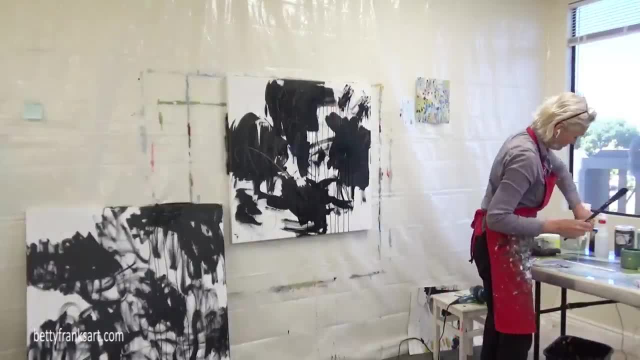 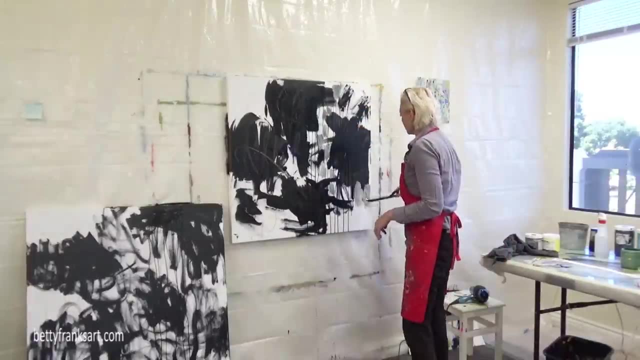 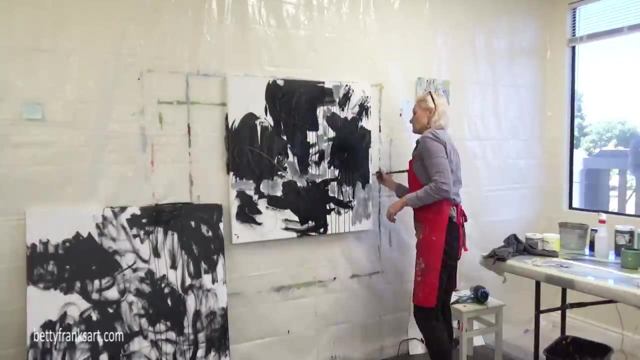 YouTube channel. If you haven't explored yet, just click on my home page for Betty Frank's art And I've got everything categorized. I like to keep things a bit organized, unlike my studio space, And the way I have them organized is I've got them separated by large art, small art. 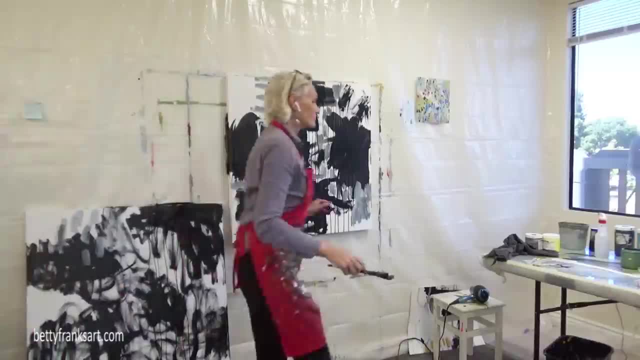 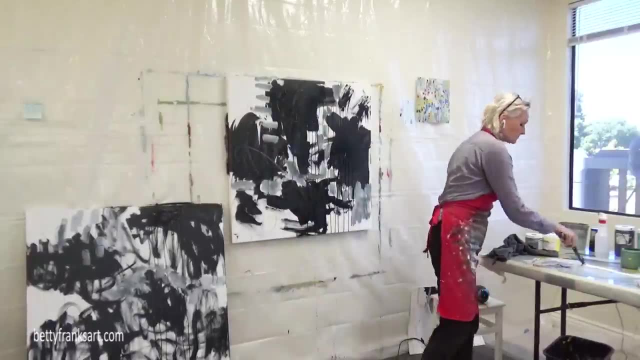 and let's see non-painting stuff, which is more like business stuff. Oh, actually I do have an art business section And something new that I started, which is vlog, So V-L-O-G video and log So vlog. 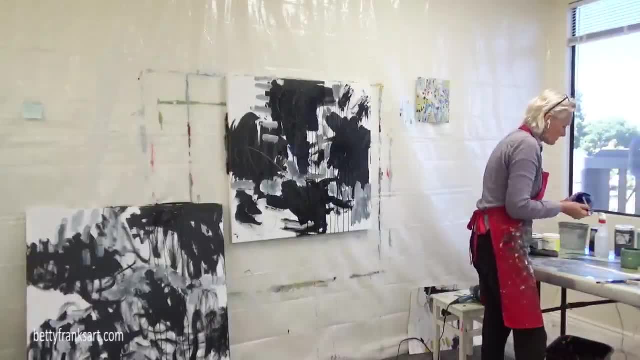 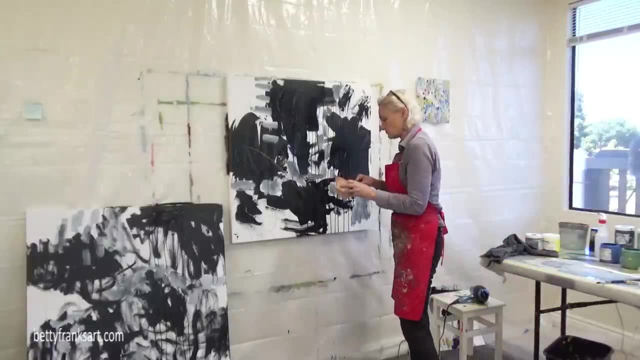 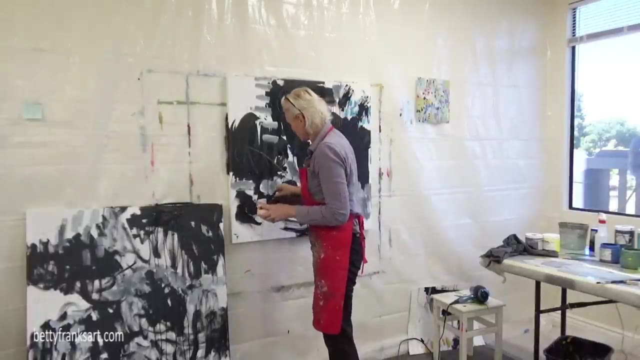 And, for those of you who are not familiar with that, a vlog is basically just a video of things that are going on, whether it's a one-day vlog or a week-long vlog or things that are happening, And so I like sharing that And I've found, you know, just something other than always sharing. 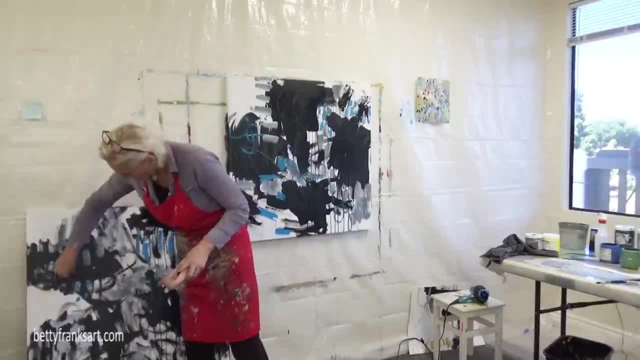 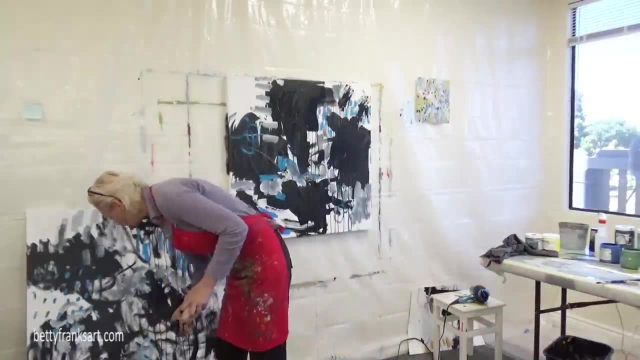 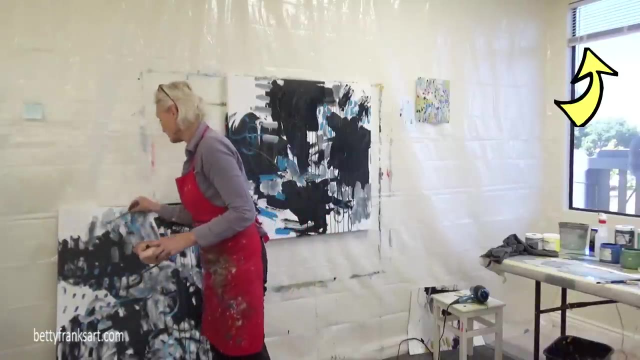 my paintings with you. I wanted to kind of give you more of a behind-the-scenes look at what goes on in my studio. So if you want to check those out, I'm going to put a link here And you can watch. I've only got two of them up so far, So the first one. 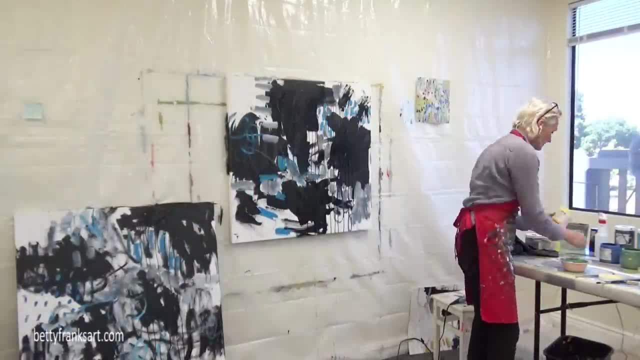 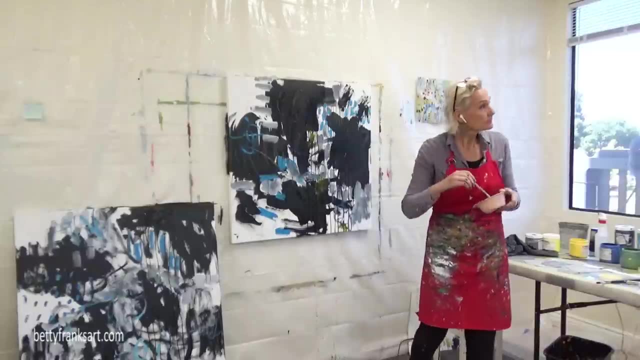 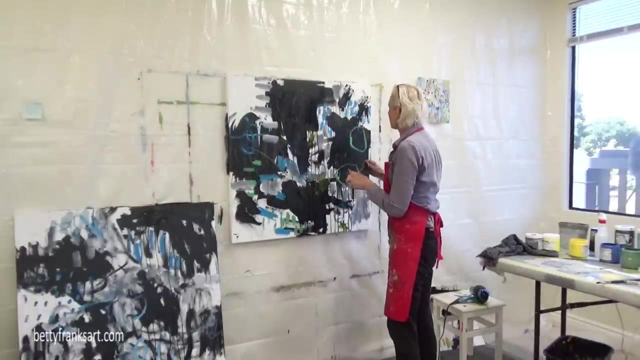 a day in the studio. some of the things that I was doing- and also creating a piece And the other one that I just uploaded last week- is it takes place over a period of time, so over a week, maybe a week and a couple of days, And it's all about me preparing for an art show. 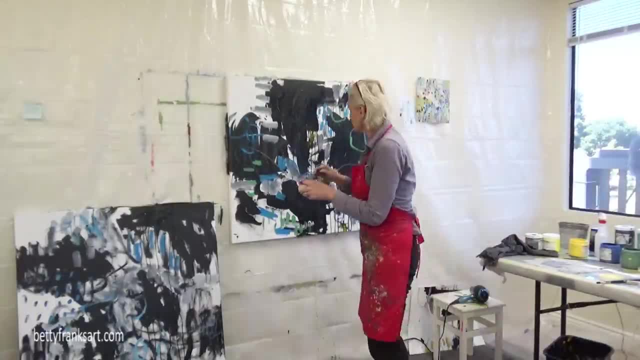 So I'll show you how I do my photography, how I do my varnishing wiring and I show you some other things somewhere in there as well. So I'll show you how I do my varnishing wiring and I show you some other things somewhere in there as well. 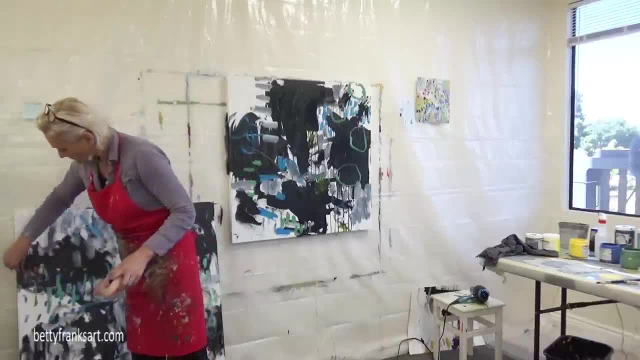 So I'll show you how I do my varnishing wiring and I show you some other things somewhere in there as well. So if you'd like to check those out again, we've got the link here and I'll also put a link down below in the show notes. 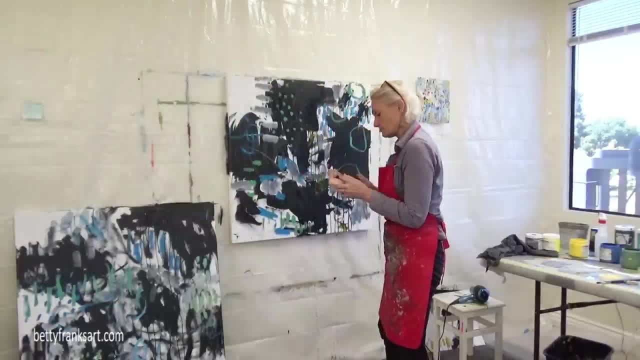 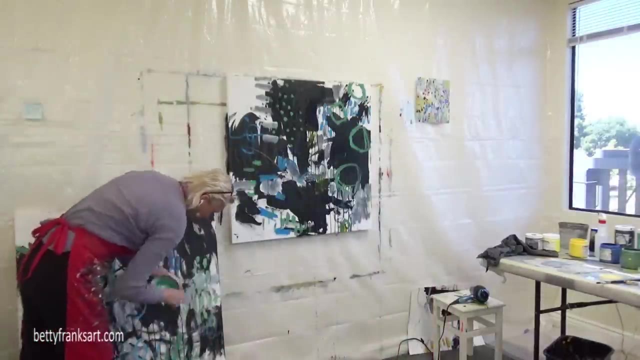 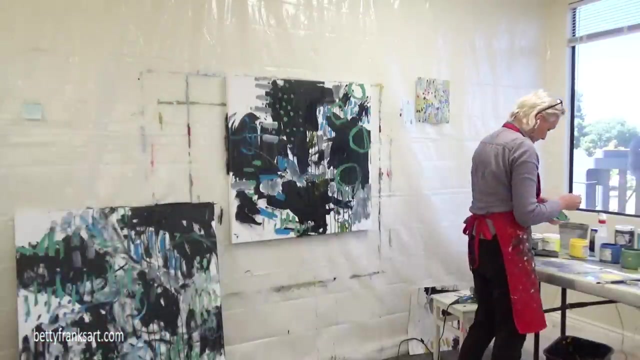 So I am working between the two of them here, just kind of going back and forth, And instead of using my palette over there, sometimes I like to grab these plastic containers and mix my colors inside of those. I often like to start after I do my black and I add some gray in there, which is just wiping off my brush and going into some white paint. 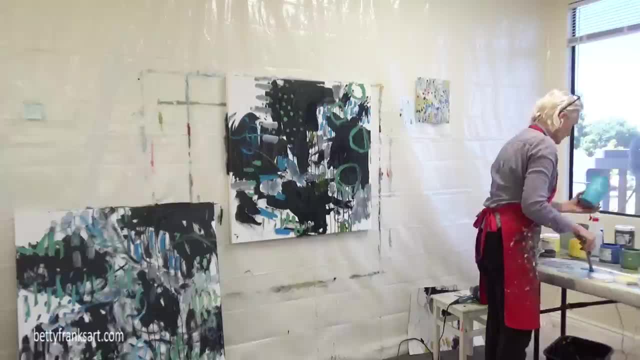 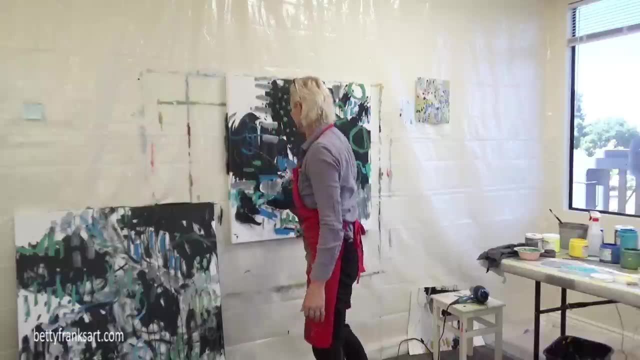 Then I like to either decide on: am I going to start with warm colors or cool colors? And the reason I like to do this is because if I mix my warm colors and my cool colors, as you probably know, you're going to get mud. 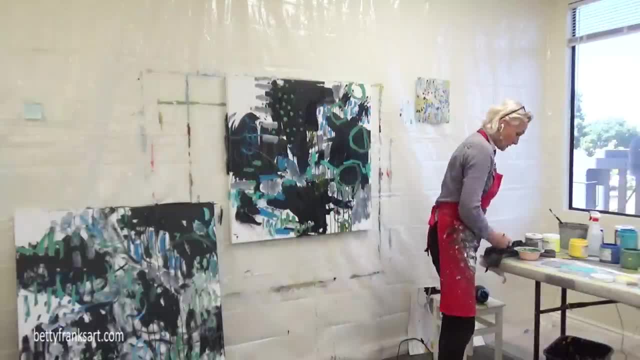 So, although I love it, I don't want to mix my colors. but I do want to mix my colors. So I'm going to do that. So I'm going to take some color. I'm going to take some color mud, but not always. I do like neutral colors, but when I am, especially these. 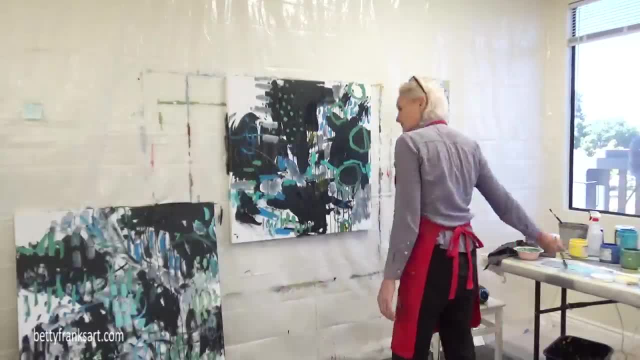 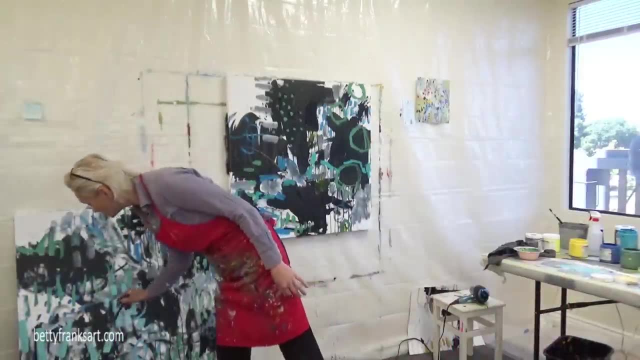 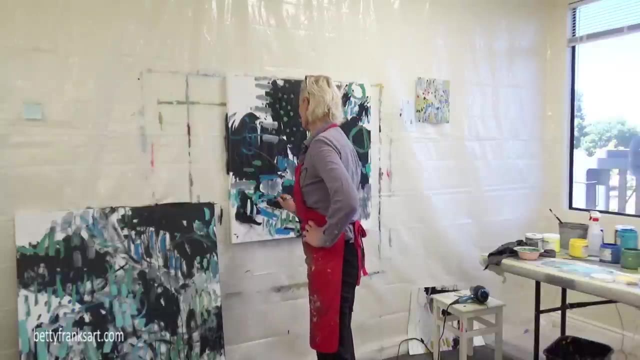 earlier stages. I like to keep my colors fresh and bright and clean, and by by keeping just either warm colors or cool colors I can achieve that. And I should say, as long as I don't dip into the black that's still drying. I'm trying to avoid it. in some areas It looks like that particular canvas is. 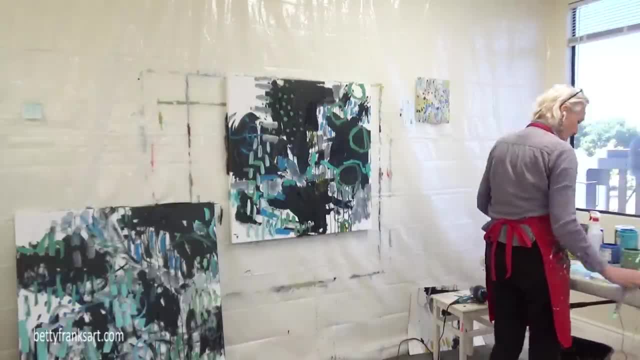 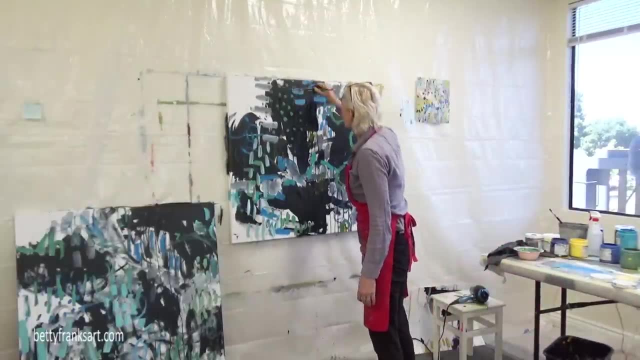 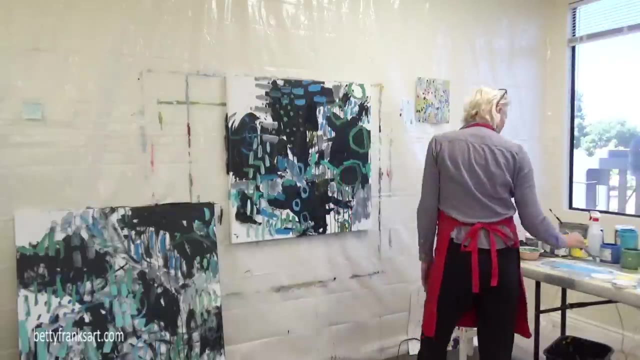 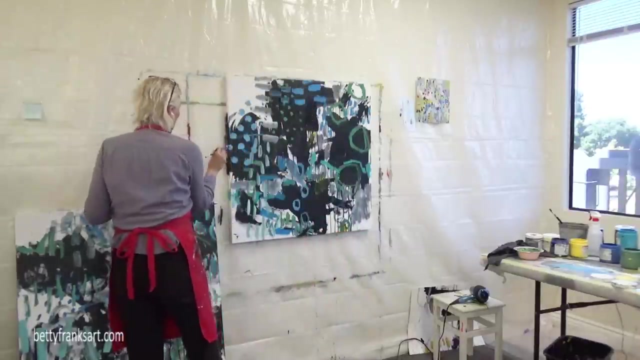 already dry and I believe that I started creating these, I want to say back in April either, maybe late April, somewhere in that timeline. so springtime, Not too hot yet in in California. I'm in the San Francisco Bay Area. I like making those circles. It's just taking my brush and pressing down and 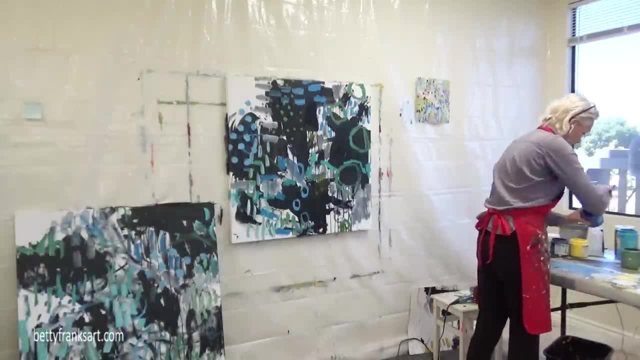 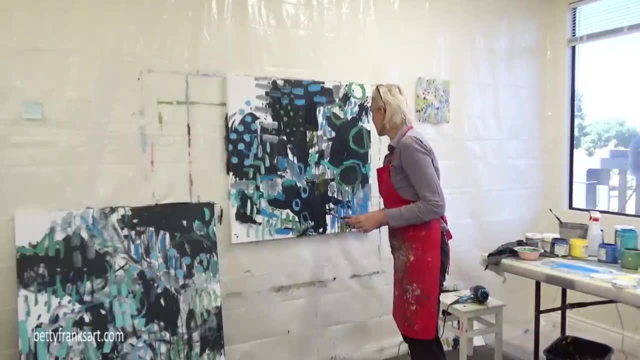 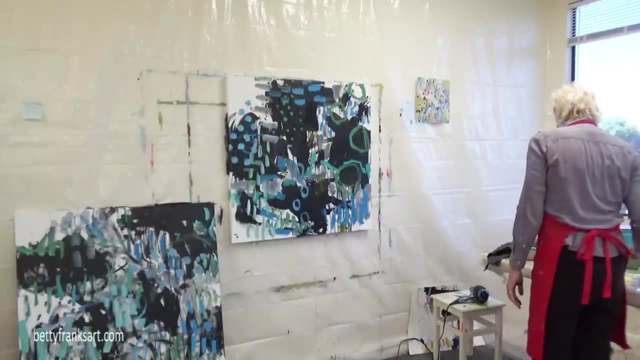 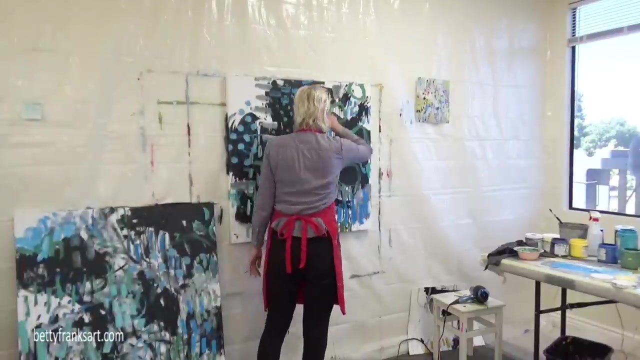 turning it Now. the colors that I like to use, or I should say the paints I like to use, are Nova color paints and I absolutely love them. I've been using them for a while and I have partnered up with them. I actually have what we call Betty's. 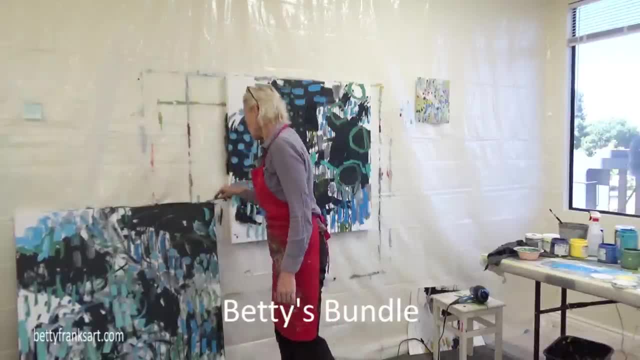 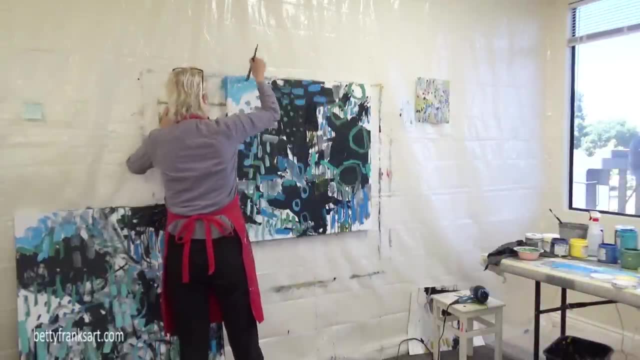 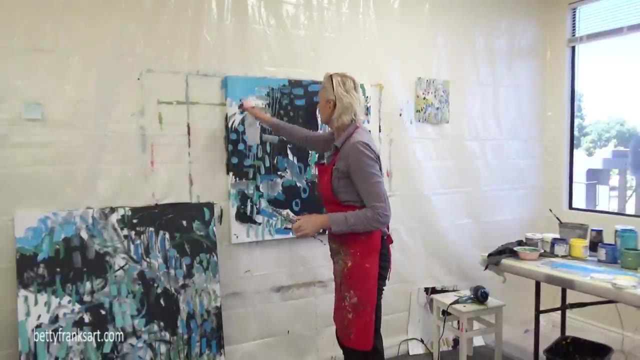 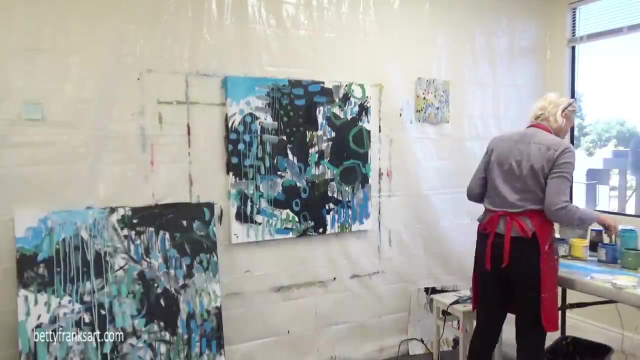 bundle, so 15 of my go-to colors that I like to use, And you can get them either in the four ounce jars, which are great if you want to just sample the colors, or the larger ones, like you can see on my table over there. Those are the quart size and the pint, And I've got the Betty's bundle. 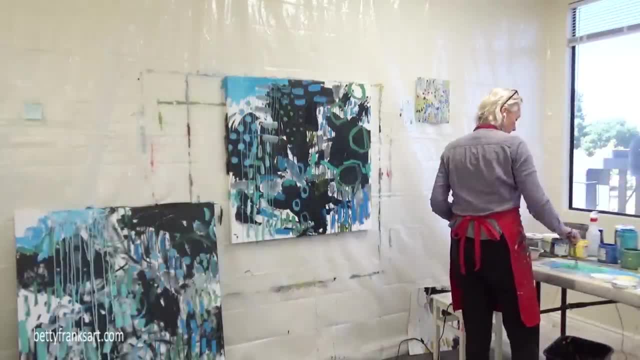 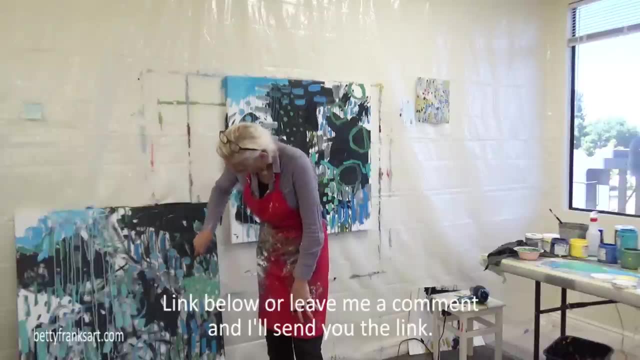 available, I should say in the four ounce and in the pint, And so if you want to check that out, I'm gonna put down in the show notes a link to them or a link to my bundle, I should say. and if you can't find the, 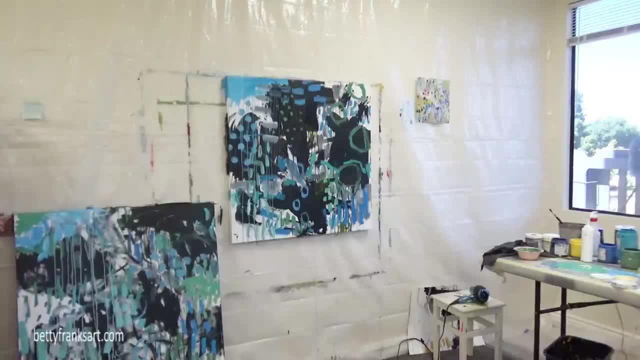 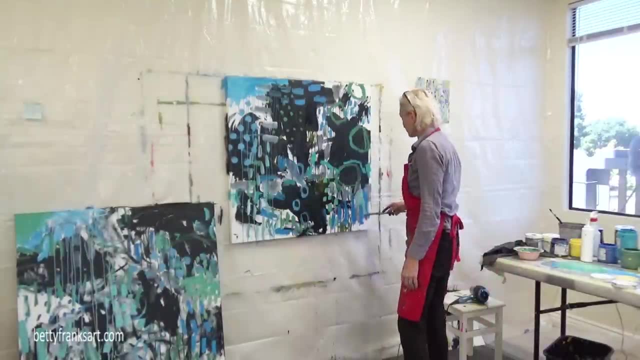 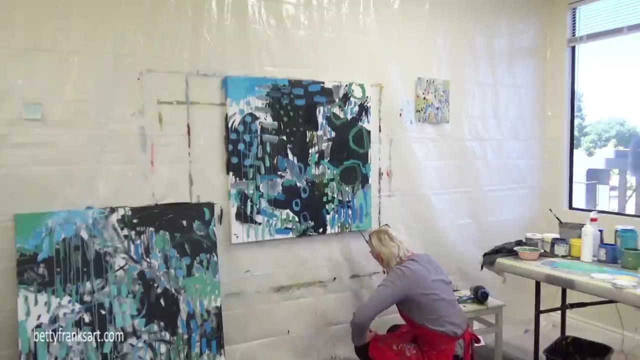 show notes. no worries, just leave me a comment down below and I'm happy to send you that link. I'm moving pretty quickly through this process, even though I did speed up the video just so we can keep it under an hour. But this part of the process is all about putting down marks and getting color on. 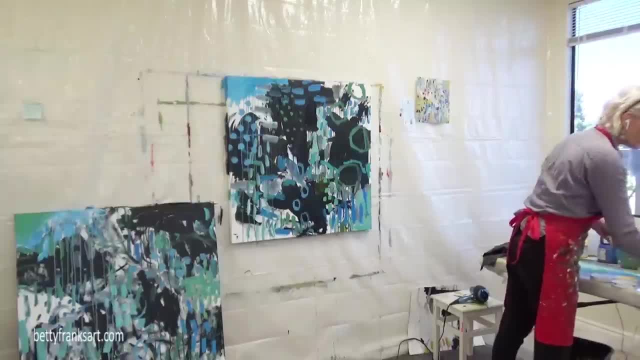 there. So I'm moving pretty quickly through this process, even though I did speed up the video just so we can keep it under an hour. but this part of the process is all about putting down marks and getting color on there on there in one way or another, but also starting to semi-think about composition. 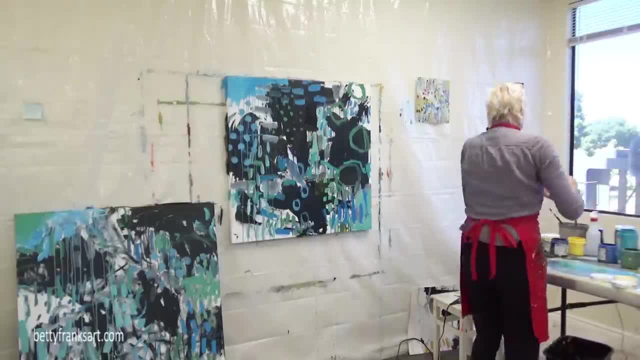 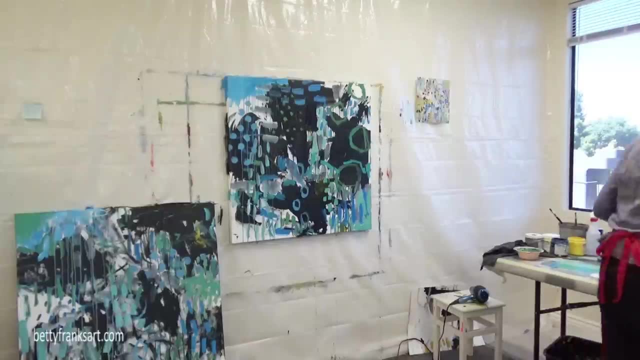 a little bit. and I say just a little bit because I do think about, you know, getting some larger elements on there and some smaller, different types of marks, different shapes and sizes, and the more I do that at this stage, the easier it is for me in the following layers that I put, down. I went looking for my rigger and because I had only been in the studio for about a month, month and a half or so, I still didn't know where all my stuff was. It was unpacked, but in new places. that was new to me, so it took me a while to kind of get used to that. 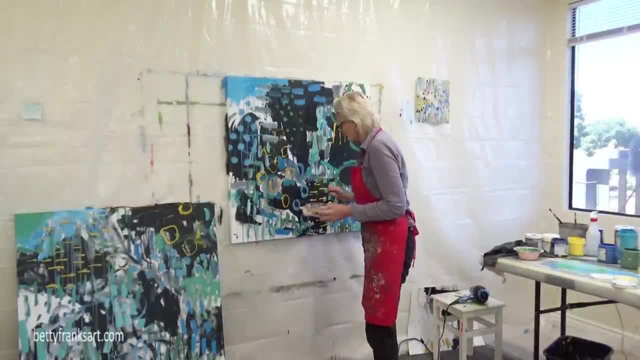 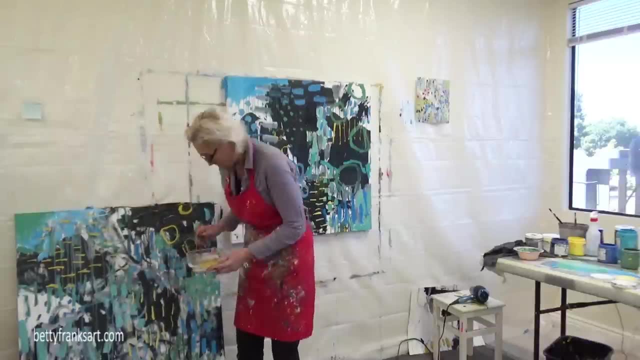 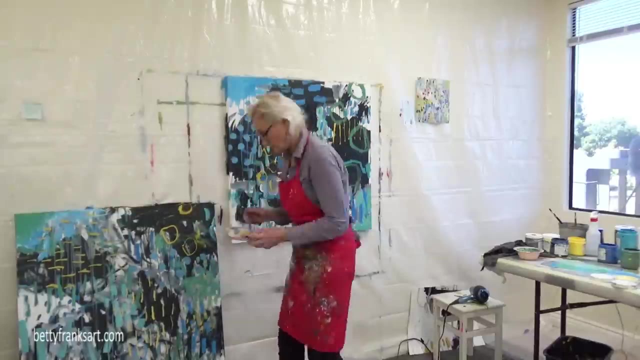 I love the rigger. It's a small brush with very long bristles and I use it either when I'm working on small art or even large art like this. It makes these wonderful little thin lines, and I like to do that. I like to have a lot of variety in my paintings. 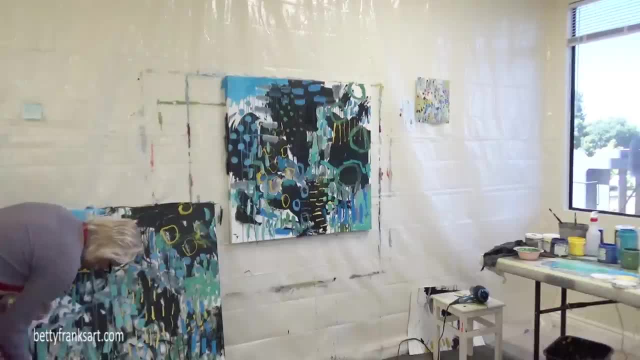 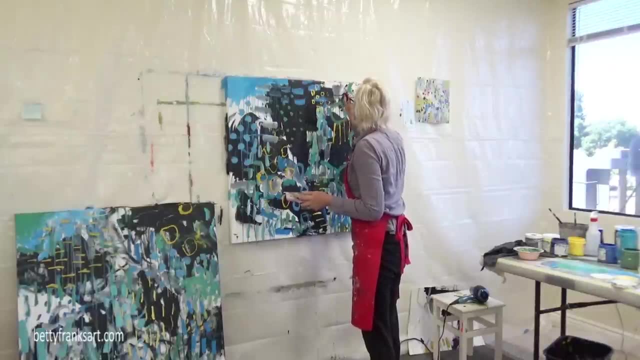 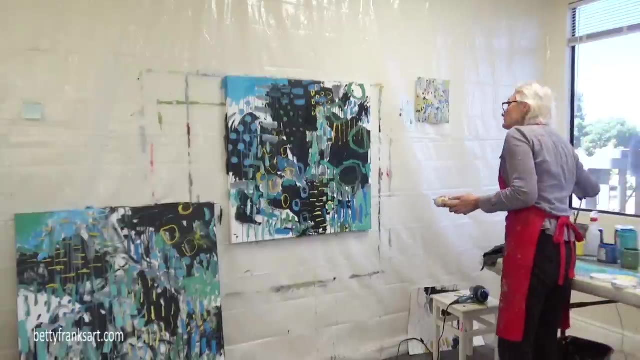 you know, whether you know, I use a larger brush sometimes and middle-sized brushes and small brushes, so that helps add a lot of variety to the piece. Now, if you're new to my channel, let me tell you where my inspiration comes from. It comes from my love. for fields of flowers, And the story behind that is when I went to Croatia in 2018, the spring of 2018, that's where my parents lived. That's where they were born. We grew up in San Jose, California. 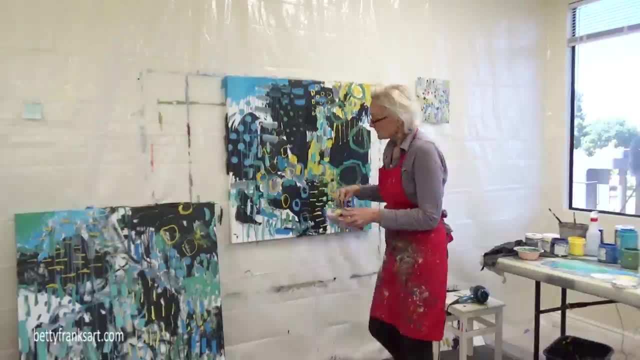 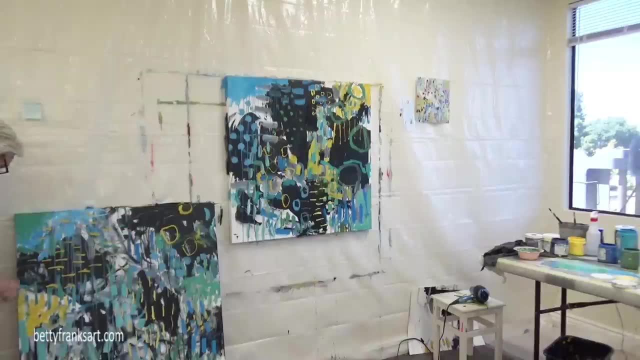 but when they retired they went back to Croatia. They built their home there. They're both from the same village and it's just wonderful. It's on the Adriatic, looking out towards the mainland. They're on an island, And so when I went to go visit my mom and I would go for walks. 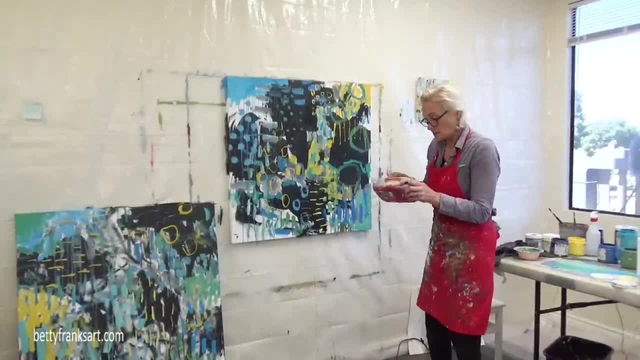 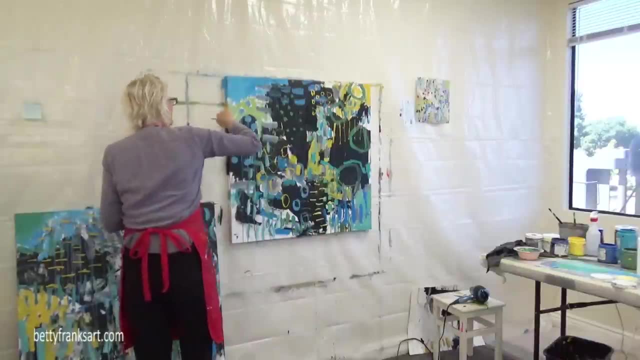 and during that time of year all of the wildflowers are in bloom, And so we would be out walking and we would pick all these flowers and make these little bouquets of flowers that we would bring home and have. you know, all over the house We had all these little. 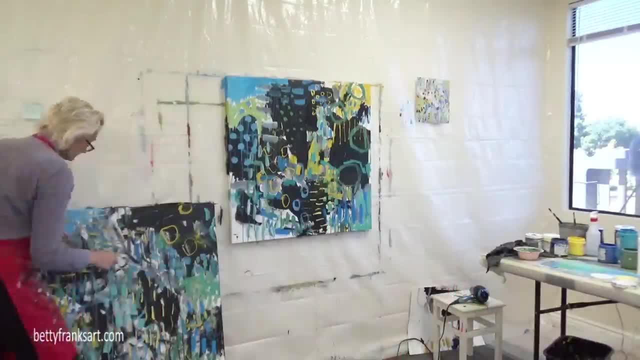 tiny bouquets of flowers. Absolutely loved them And I realized, you know, I brought my paint supplies with me and paper to work on, And I still remember to this day telling myself: okay, Betty, you're on vacation, just relax and just do whatever you want to do, Because, at that, 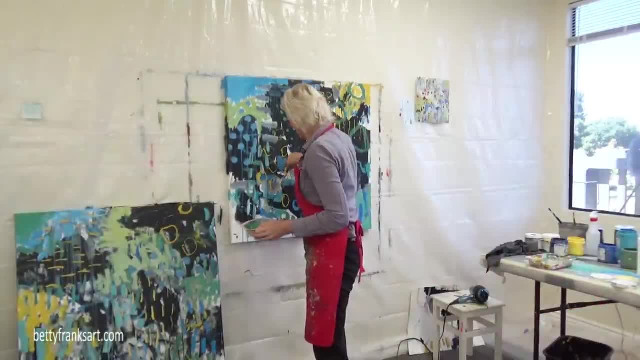 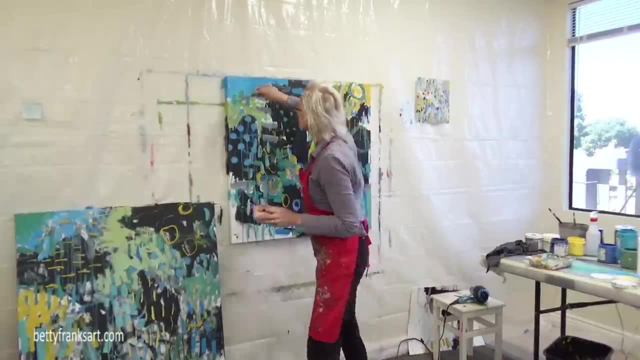 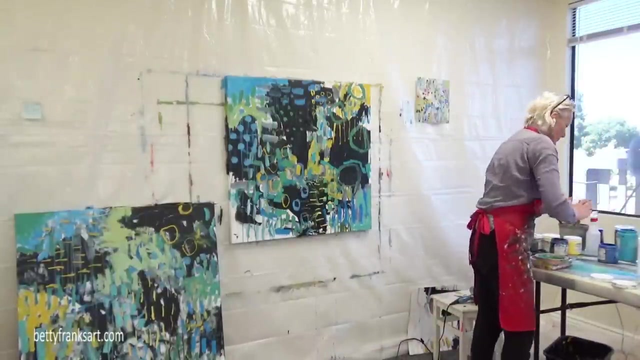 point. I truly didn't have a style yet, but I was already inching towards this style, but I didn't know it at the time, And so when I was creating, I realized later that I was creating these, these flowers that we were seeing in our walks, And I was 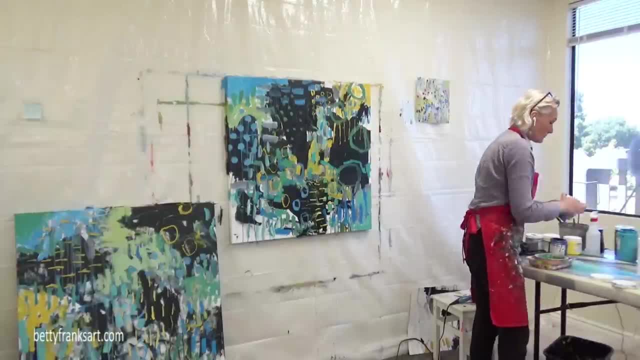 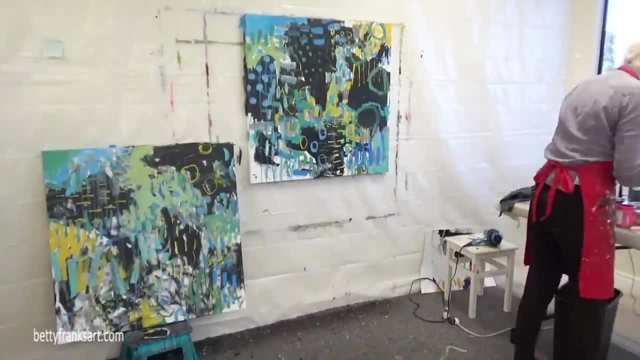 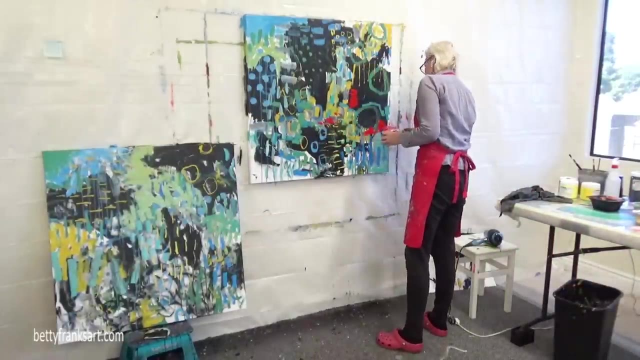 creating, you know, recreating these flowers that were all over the house and the joy that they brought me and the happiness that I felt seeing these flowers, And so that's when I discovered my style And it- and, like I said, I didn't didn't discover it right away, It took me. 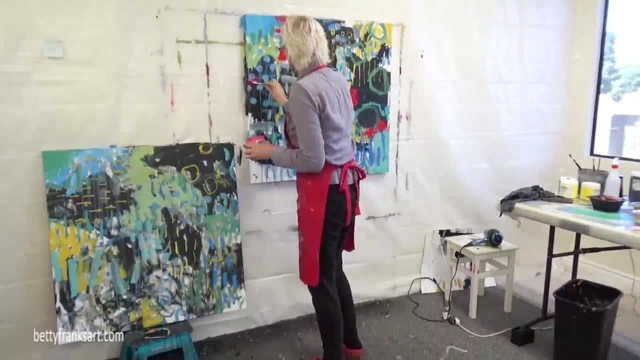 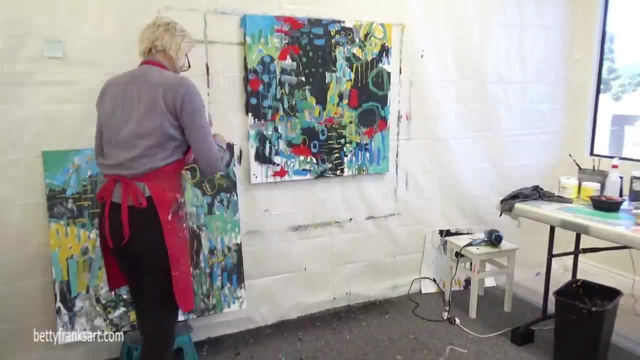 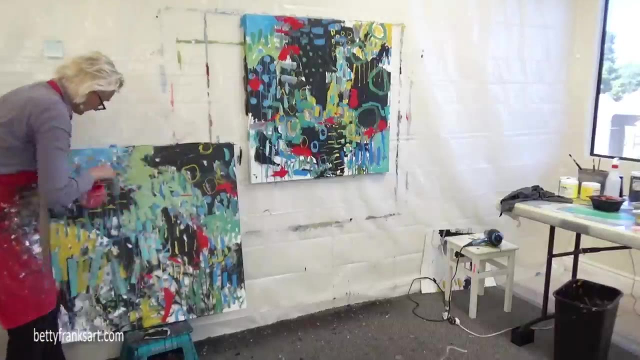 a little while to figure out that that's what I was painting, And so I credit my mom. I thank my mom for her love of flowers and making these little bouquets of flowers And for me, you know, reconnecting with my love for flowers in in kind of a special 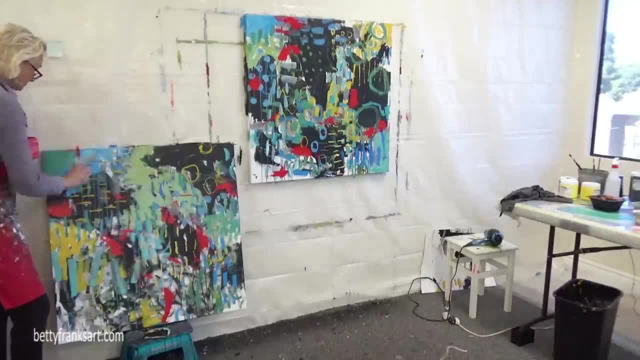 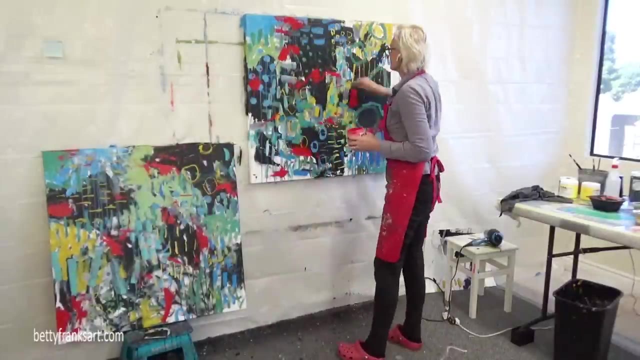 way And also in. I'm just so thankful that I was there that spring and that I finally discovered- you know what it was- that was trying to come out of me And so- and it took, it took me years. If you're on that journey, then you know what it's like. 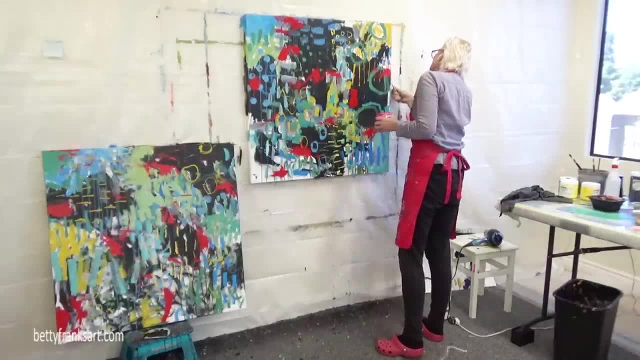 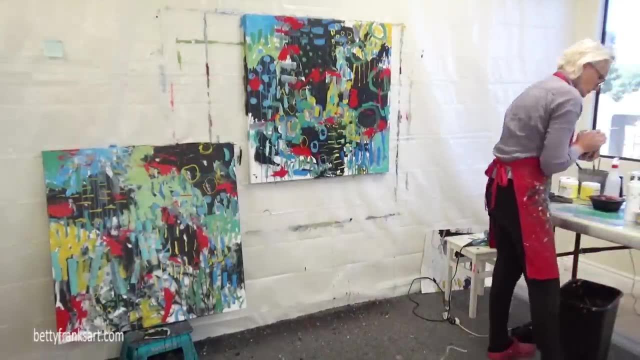 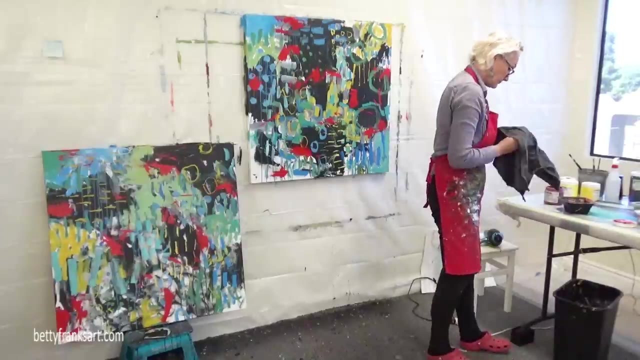 It's not something that happens overnight, Although you know for some people it might. I don't know. I can tell you for me. it took me years to figure it out, because I started creating abstract art in August of 2015.. That was when I decided I wanted to be an abstract artist. 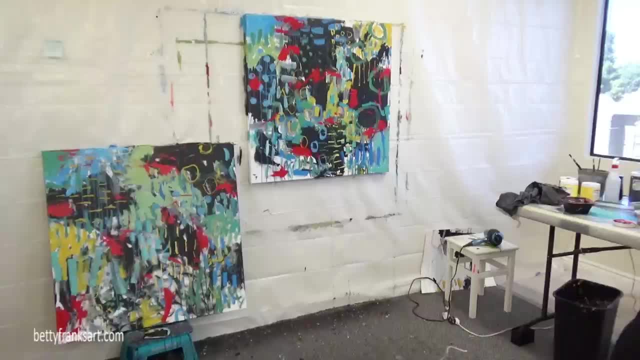 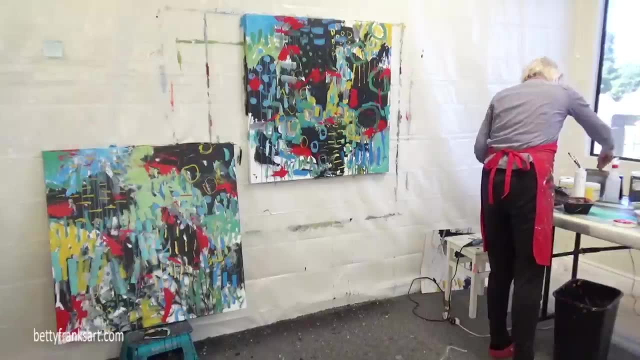 but had no clue. Well, what does that mean? What kind of art am I going to create? What is it? What is it going to look like? What is it that I'm trying to say in my artwork? So, from 2015 to 2018, it took me- what is that? About two and a half years, almost three years. It took me a while to to figure it out, And every step that I took during that journey was important. It brought me to where I am today And I am, you know, grateful for all of that, even those very frustrating times and annoying times, And 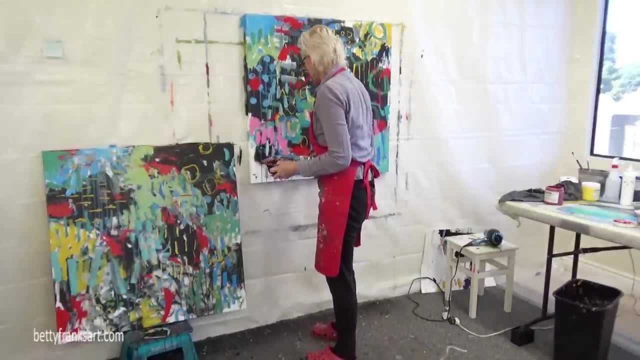 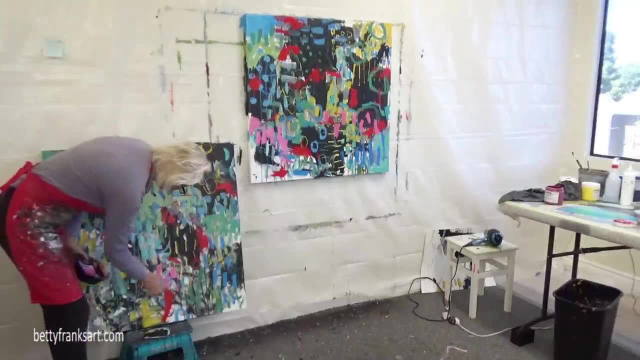 you know, I have no clue what I'm doing times. All of it was for a purpose, a greater purpose. I'm having an issue with that brush. It keeps falling apart, but I still keep using it. So anyway, going back to you know, hang in there If you're still trying to figure it out. 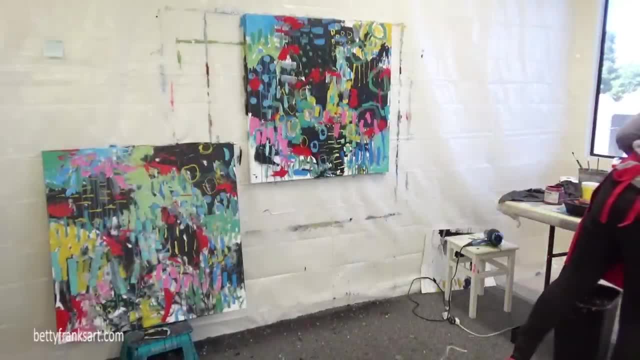 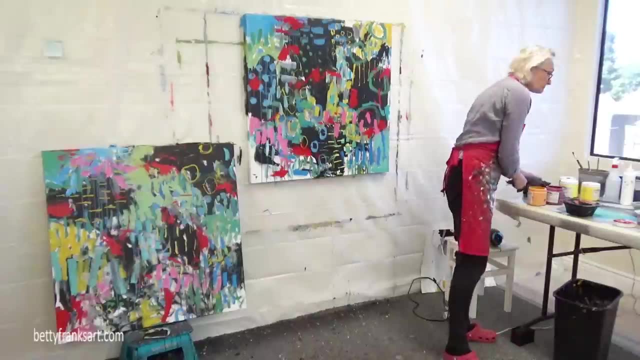 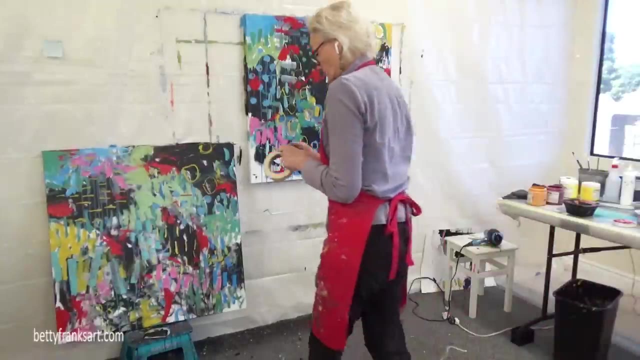 hang in there, just keep creating. It is going to come to you. It is going to find you, as I like to say, especially when you are at least looking for it. When you kind of stop looking for it, it will end up finding you. So, anyway, hang in there. I've got the tape out. 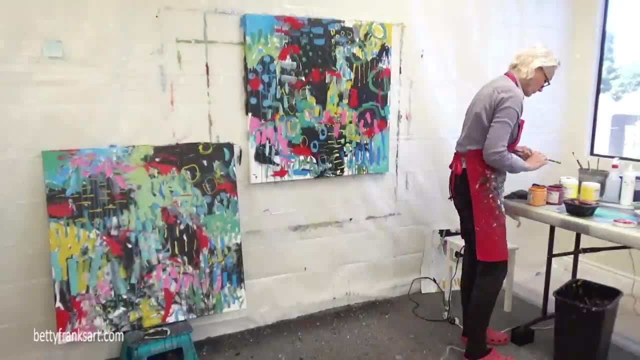 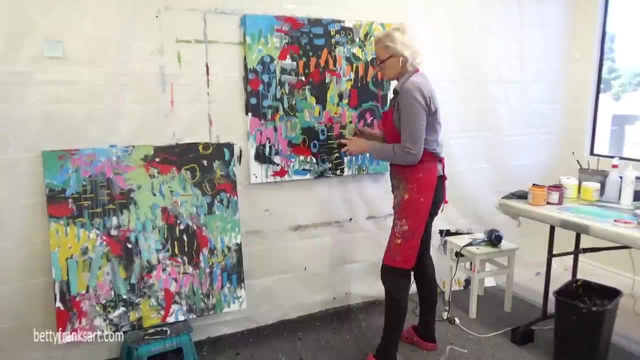 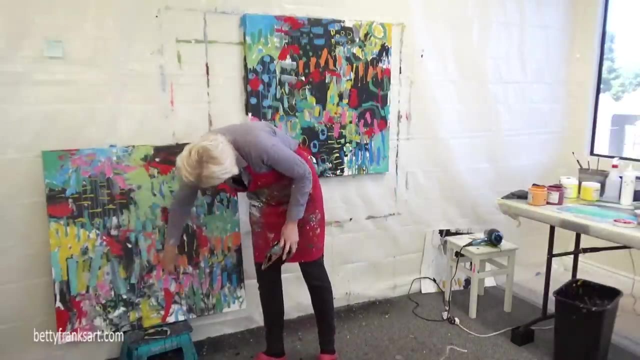 and decided to tape that up. for whatever reason. I really liked that brush, All right. When we came back, I came back in with warm colors, as you can tell. So adding warm colors right over the some of those cool colors, but keeping some of those cool colors. 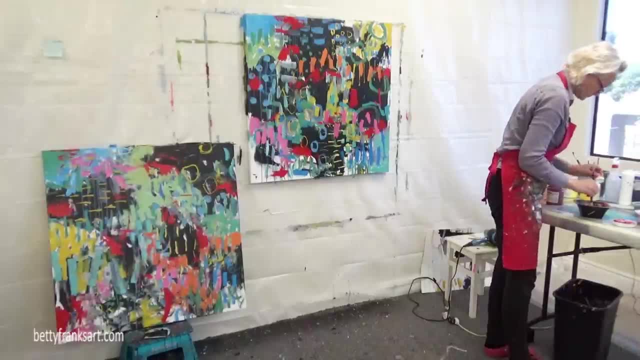 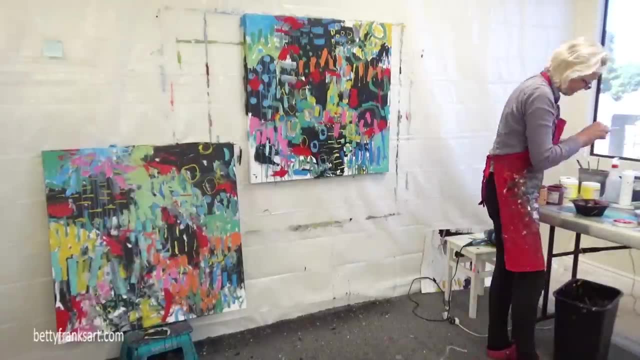 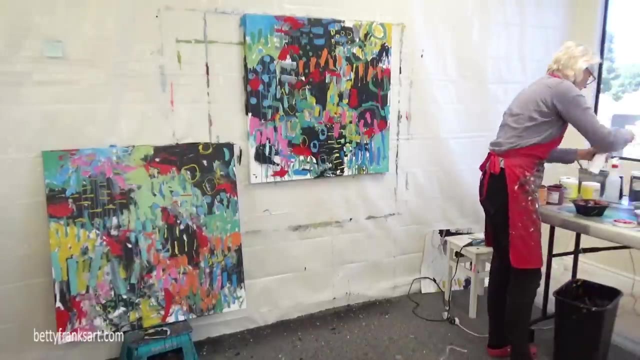 too, And from there we are going to start with сбus flop. Meanwhile I was blanking on the kind of frames that I wanted to add and I found a place where I found the white. I've got white over there. that was in a smaller jar that I no longer use. It was kind of like 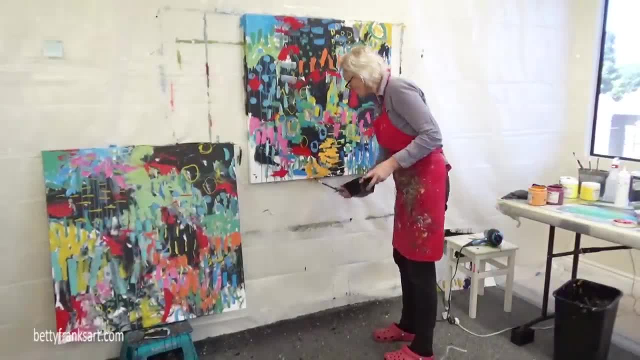 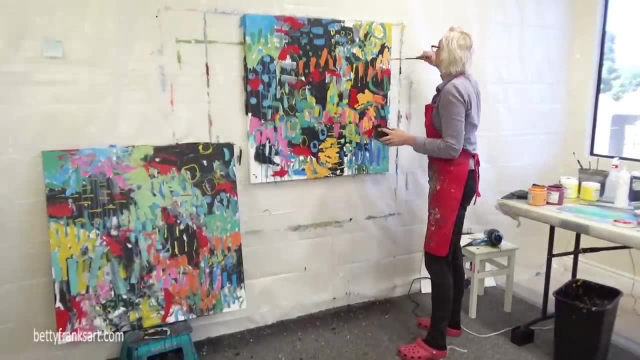 ketchup bottle size type of bottle for paint, and it just dried out too fast. I don't like putting lids on stuff, Joy, And so it really doesn't work For me. now use Nova Color Gesso that I absolutely love, but I saved my old Liquitex Gesso bottles and I 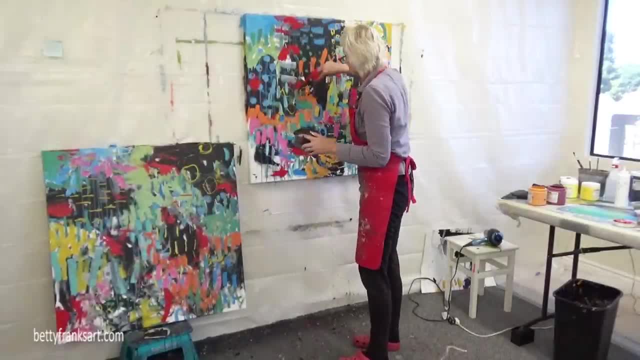 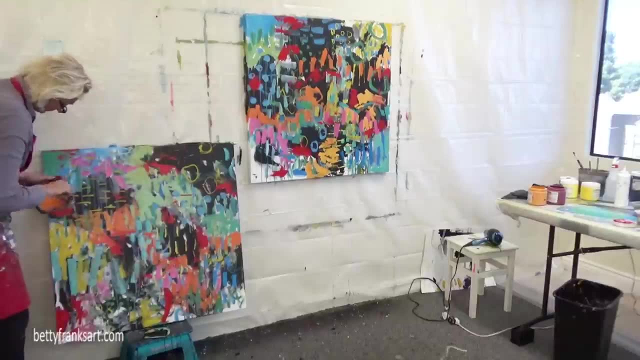 just refill those all the time now because if it dries up then it's very easy for me to just pop off that dried up paint or gesso and continue using it. So I'm moving right along here and even on this layer, not thinking too much. I just want to get. 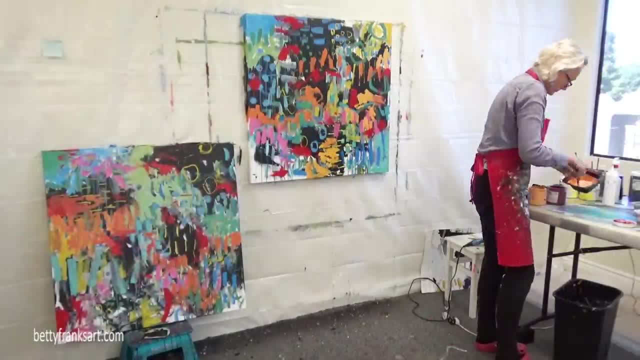 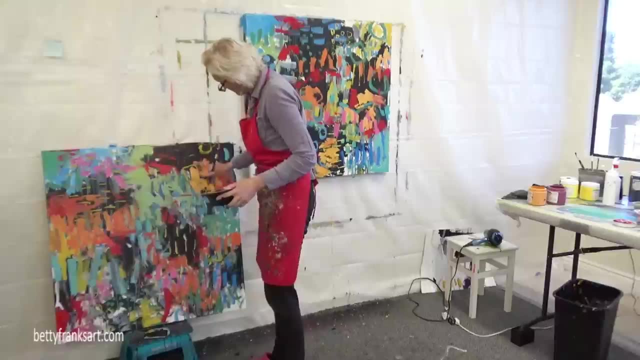 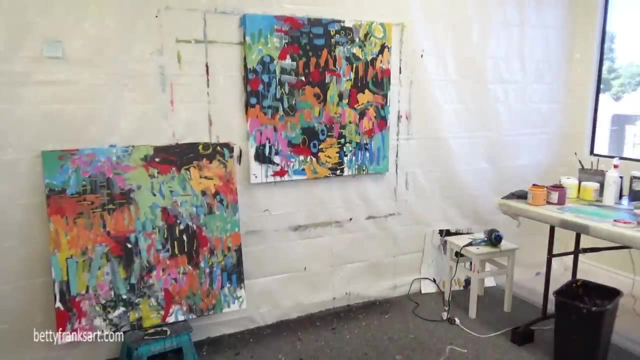 some paint down. I want to get these colors down and you'll see later- oh, I guess much later, after I do my second recording, but the one that I'm working on right now, I think is, is the one that I used for my second recording. it looks completely different from from where it is now, so that's the 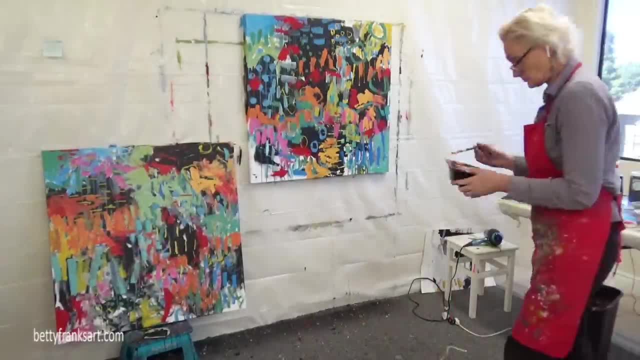 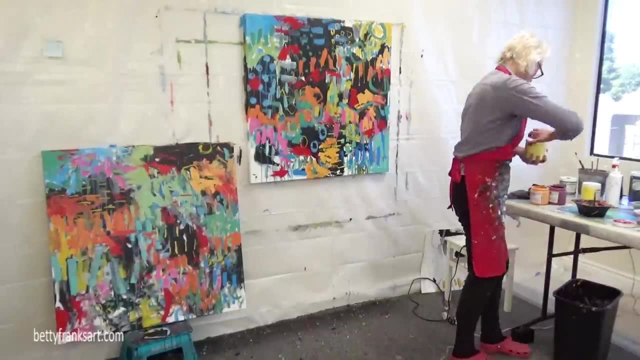 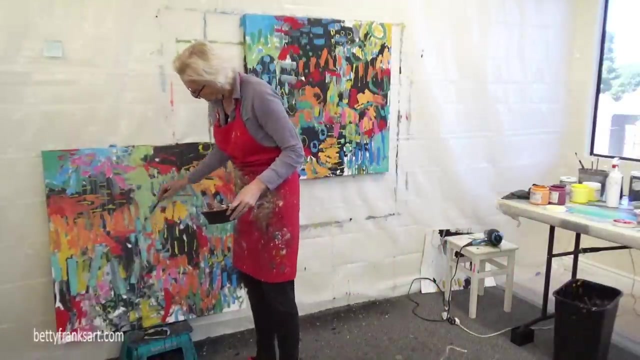 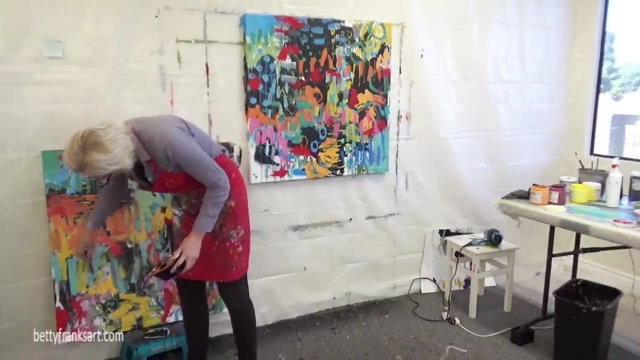 importance of me just trying to get some layers down so that I can figure out what I want to do later, And I was just looking at the picture of the final piece and I have a feeling that the one that I'm working on- the lower one, I think- is the one actually that I end up finishing during this. 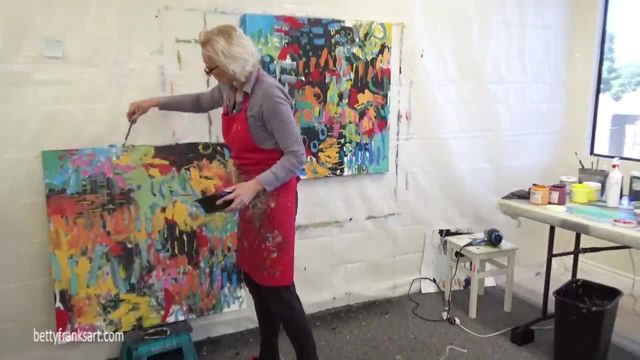 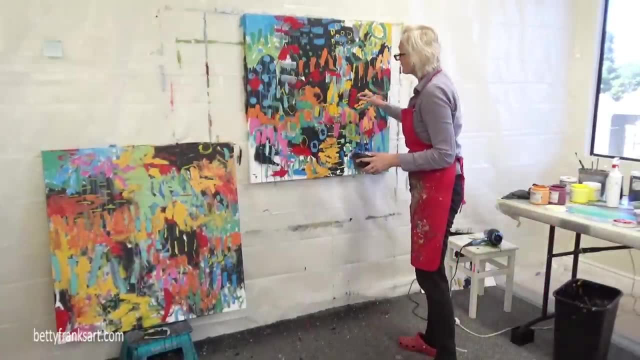 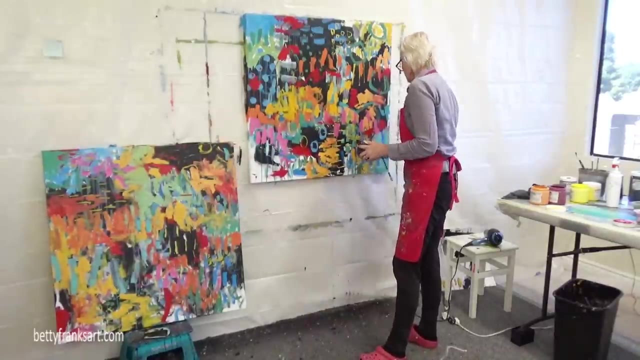 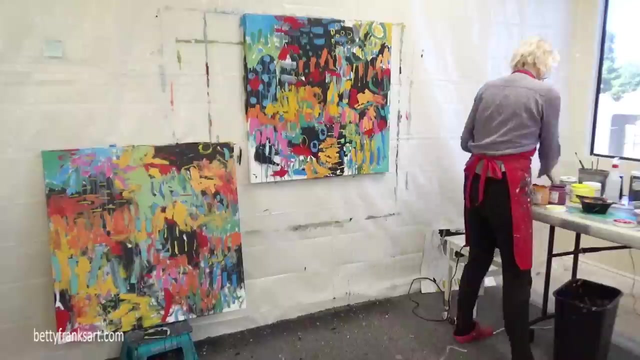 particular videotaping, and I guess it's the the upper one that's on the wall that I end up working on later. It's kind of fun watching them come together. it's been, you know, months. right now we are at the beginning of August, so it's August 9th 2022 when I am doing this voiceover for you. so it's been. 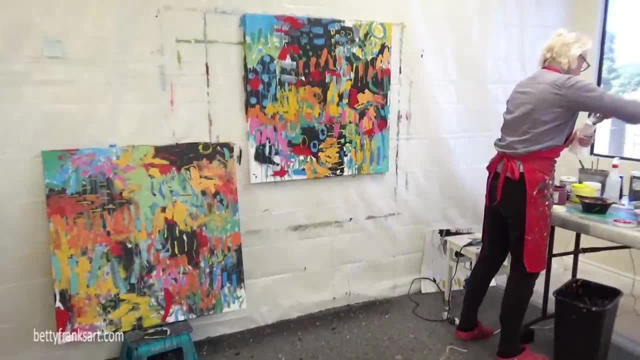 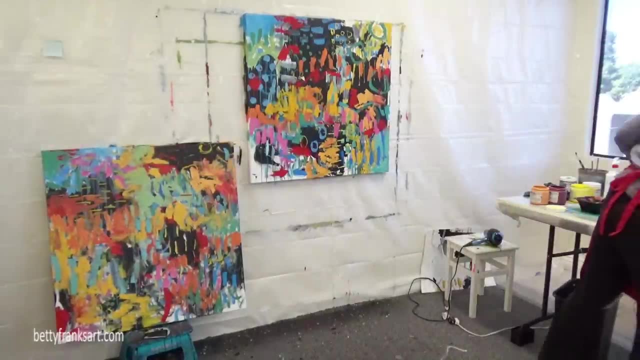 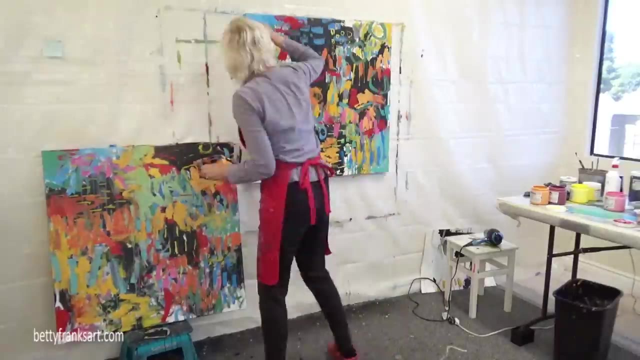 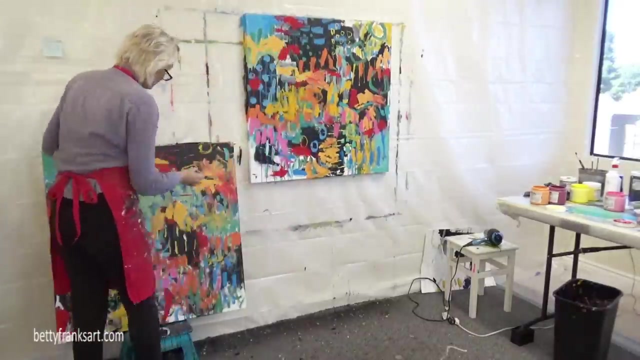 many months since I created these, so for me it's very fun to look back and see how they came together. I had a gentleman by the name of Brian. he's an artist. he creates these absolutely gorgeous flowers, and he was telling me that his granddaughters watch my videos and create. 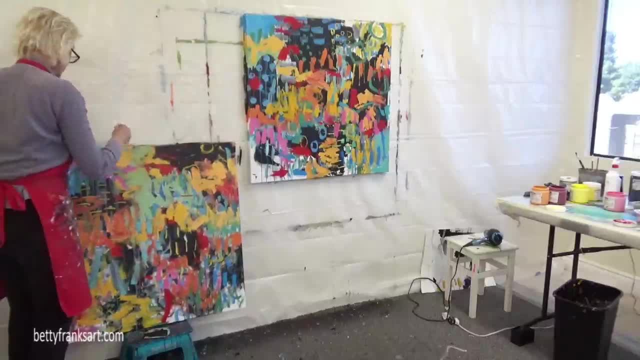 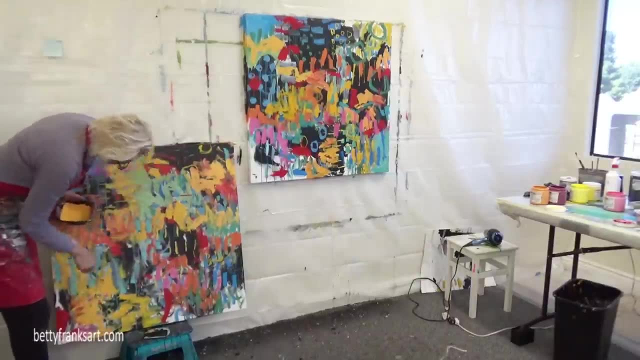 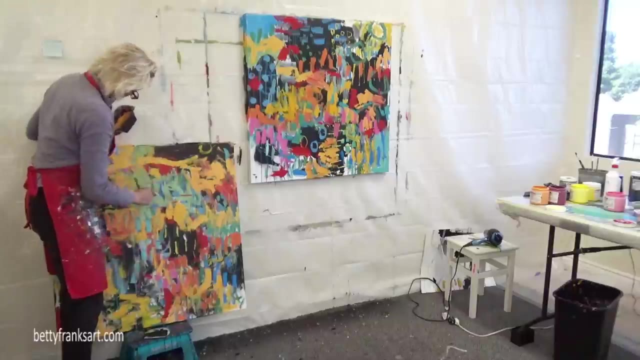 abstract art while they are watching me, and so I was just. it just made my heart so happy knowing that I'm also reaching a young generation of artists, so I want to do a huge shout out to Maddie and Val and keep on creating, ladies, thank you so much for watching my videos. 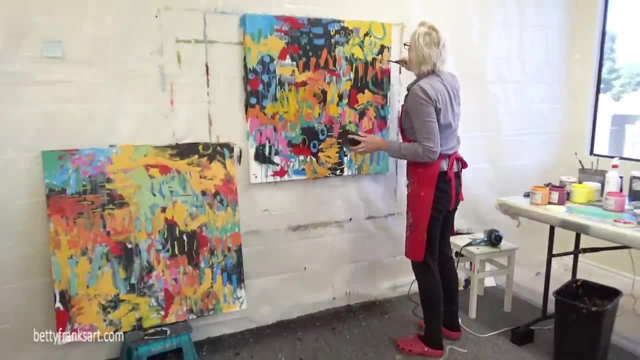 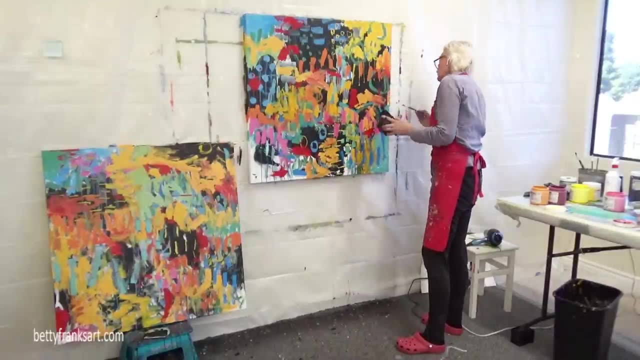 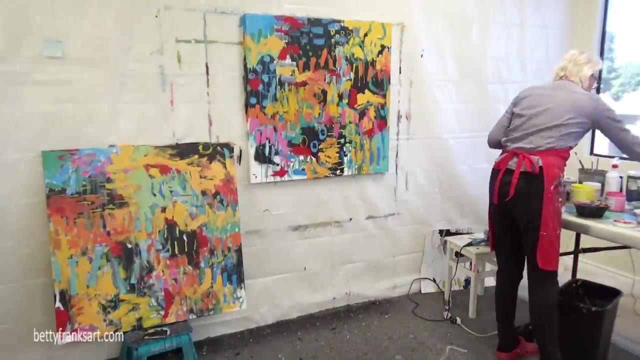 Coming in here with a lot of yellow. I love cadmium medium yellow, or I should say I use it a lot, but straight out of the jar I really don't love, and so I tend to mix it with other yellows. I think I had a Hanza yellow and I've got. 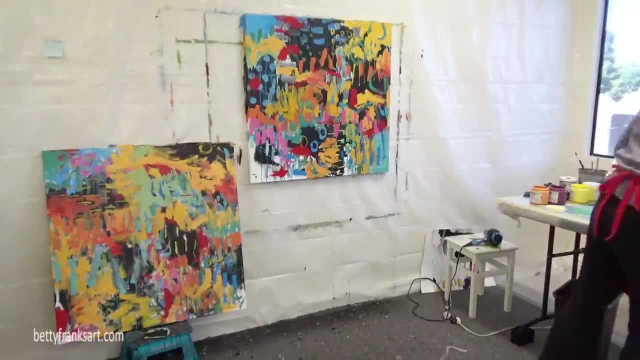 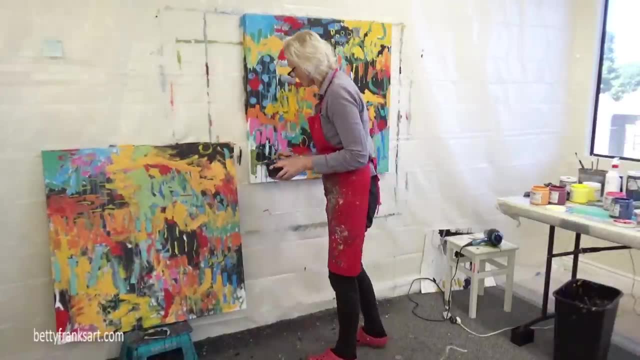 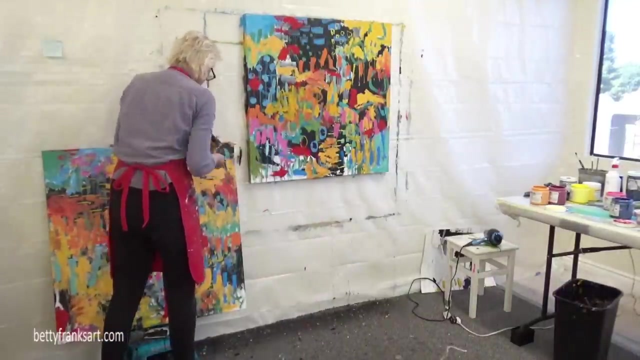 um, oh, let's see Indian yellow on my table, and so I like mixing those yellows together so that I can create a, a yellow that I'm much more happier with, and I think I added some black to that yellow and that's why I've got that green going on, so I didn't switch to my cool colors, I just um. 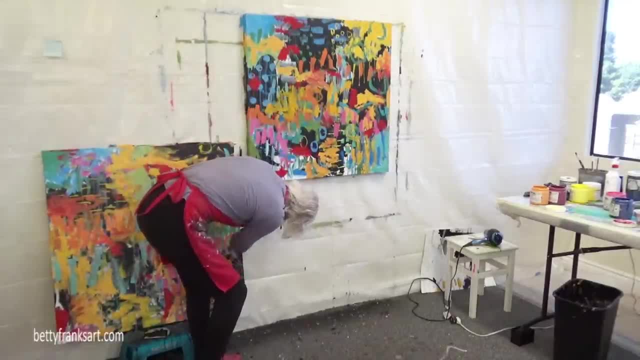 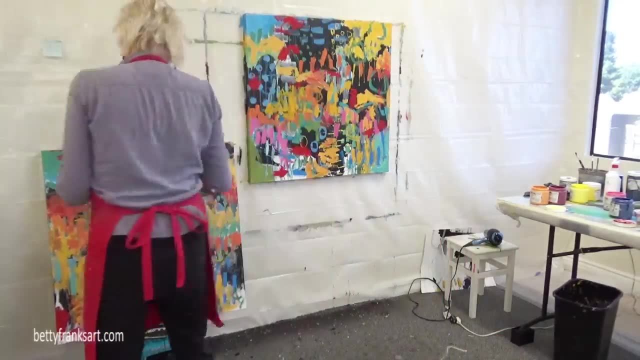 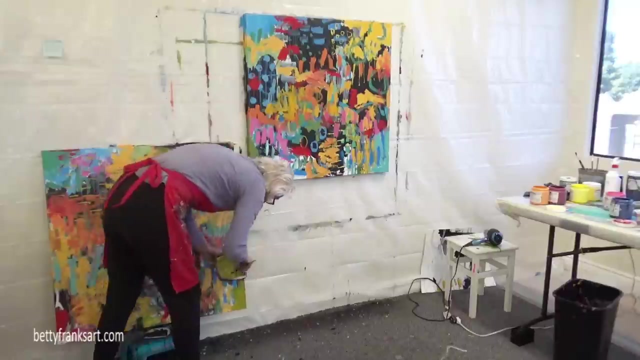 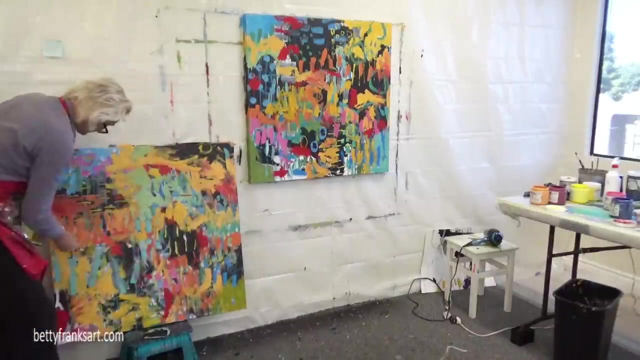 probably was using up whatever I had over there again, but that is where they come from and so, um, it's don't feel like anything at all, so I can't really bring them up here personally, but it's an endless process coming close to being done with these first few layers and then I'll be able to. 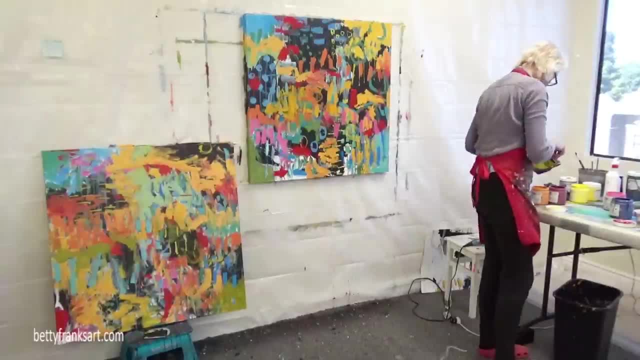 just grab one of them and continue working on them. If you are enjoying this so far, it would mean so much to me if you would give me a thumbs up and also effect notes. Click the rejected videos. don't forget to put them down and I have openв. 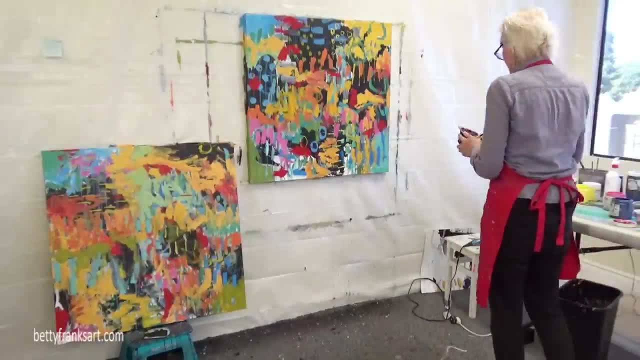 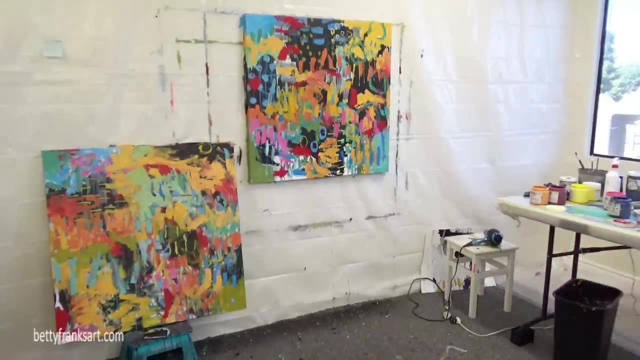 of videos for me and some other time. NextQu? andacio. thanks a lotackerscom. Also, if you haven't already, if you can subscribe to my channel, I would so appreciate it. It really helps me out so much And it's something that's really inexpensive for you to do, which is, you know, hitting. 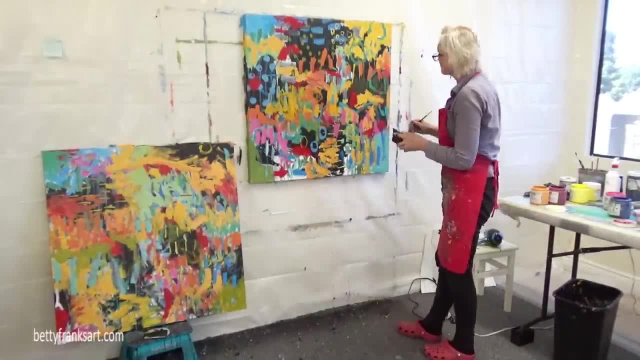 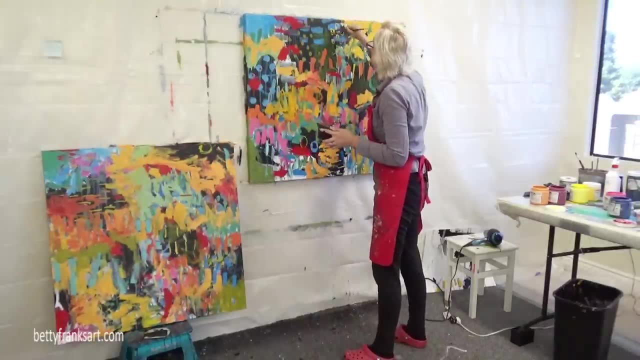 that thumbs up and subscribing- hitting that bell so that you know when I've got some more videos- It tells the YouTube algorithm that you're liking the content that I'm putting out there, And then they say: oh OK, people are liking this. 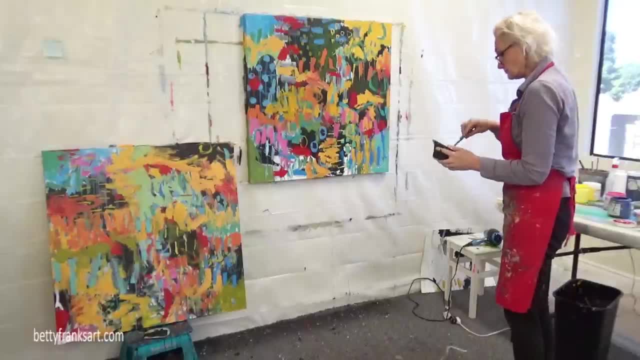 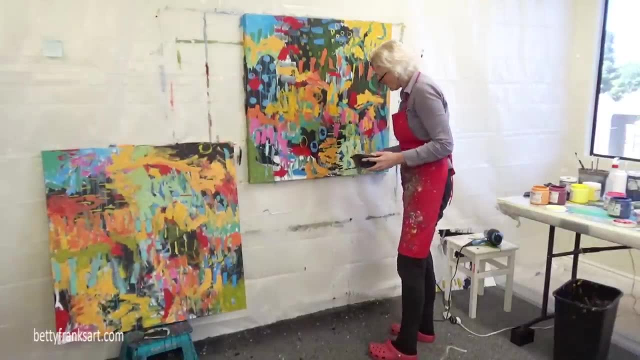 So let's show it to more people. So you are helping other folks who maybe are looking for this style of art and haven't found me yet because this video hasn't been served up to them yet. So I so appreciate you helping me out in that regard. 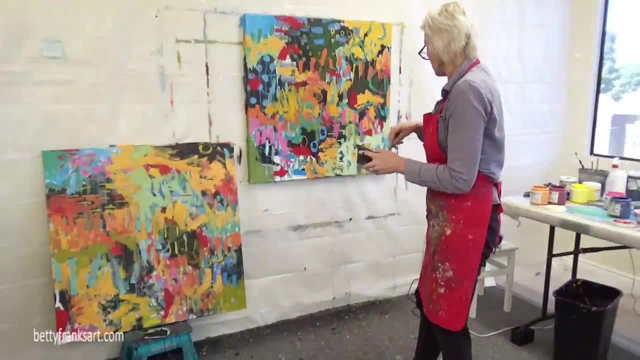 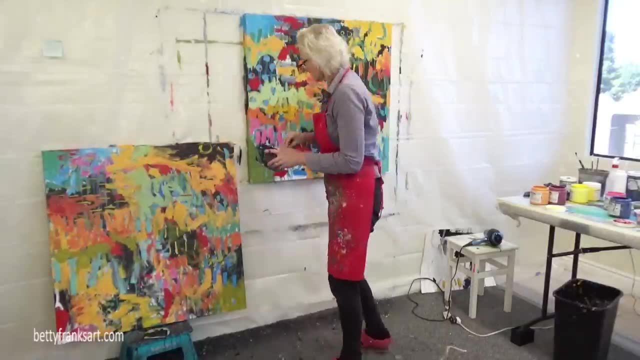 And then, if you have a few minutes, watch some of the ads that come up, because I get a few pennies for everybody who watches one of those ads And you know a few pennies doesn't sound like much but it does add up over time. 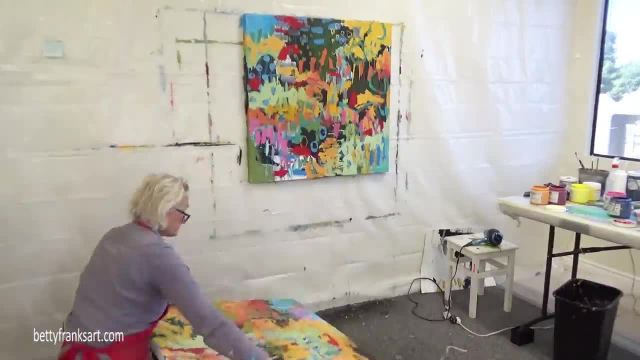 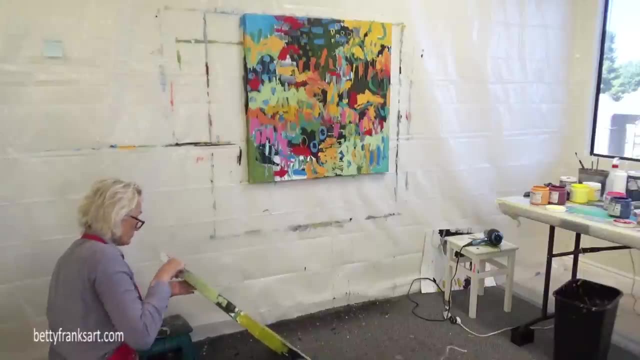 And that helps me out. It helps me with having the ability to create these types of videos for you and to just invest my time in whether it's a video camera or I'm also working on trying to get a clip on microphone so that when I'm doing my vlogs you can hear me, because if I turn away from 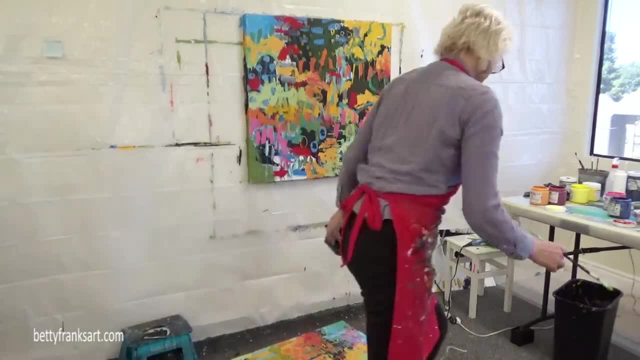 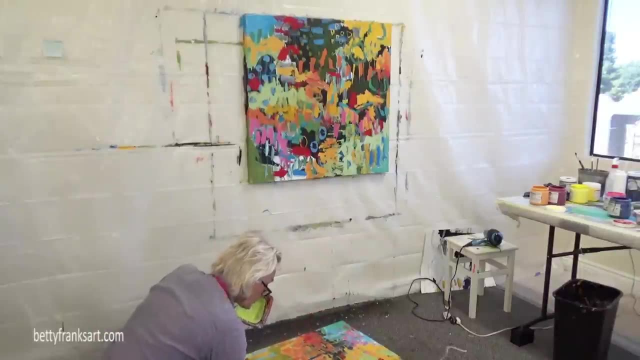 the camera. you can't hear me, So it helps me. It helps me with buying supplies, in that, in that regard, not just painting supplies, but supplies for being able to put together videos- I'm working down on the floor for whatever reason. 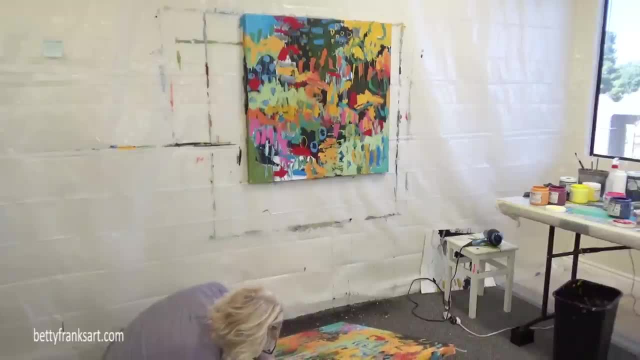 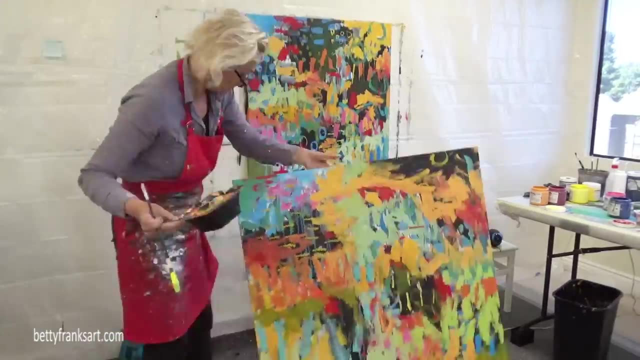 I don't remember, So we can't quite see what I'm doing down there. But oh, I was working on that one edge because it was sitting on top of that little stool that I have. I was trying to get some color going down there. 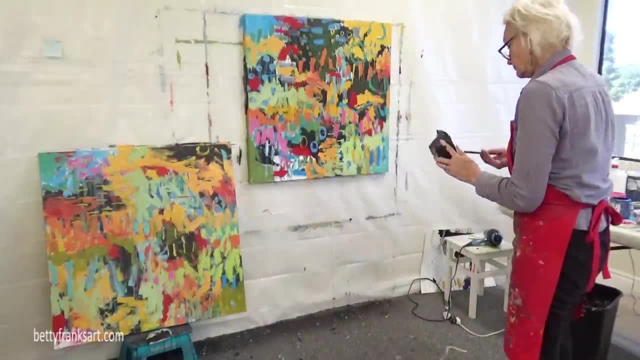 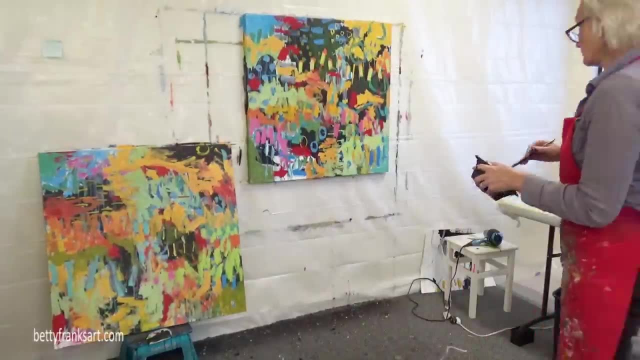 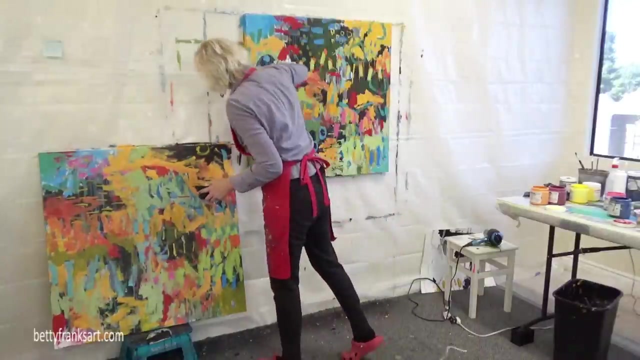 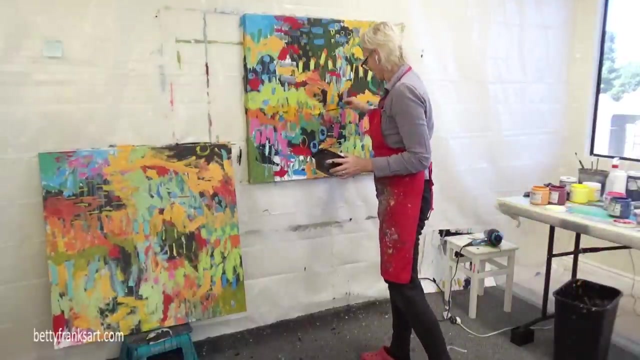 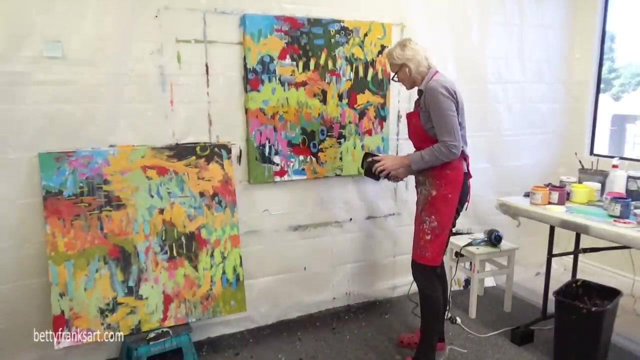 All right, moving right along, It looks like I'm already starting to put color over color. There was already kind of a different tone of green there, and I see I came in with some more green right over It, and that's something that I like to do to build up my layers. 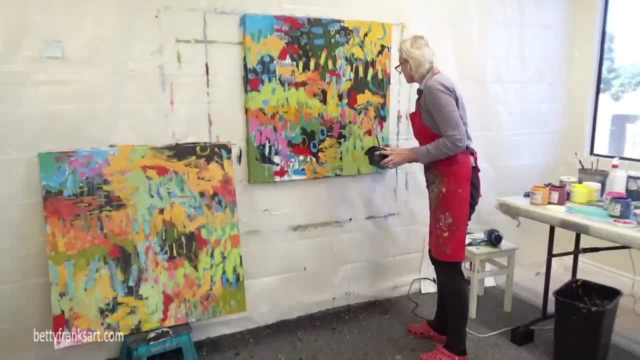 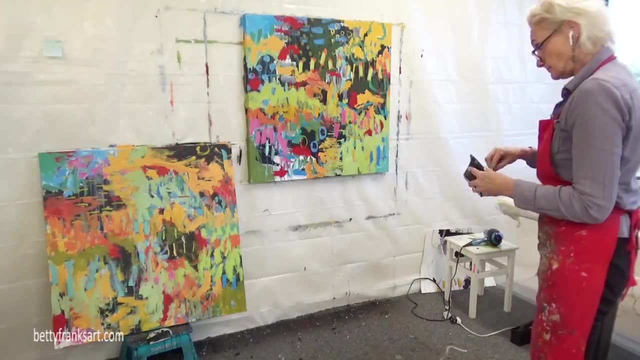 And sometimes I'll do that with you know, a similar color right over a previous color, or it might be opposite. Maybe I'll cover pink with some greens or something like that, And all those things help me, help build depth in my paintings. 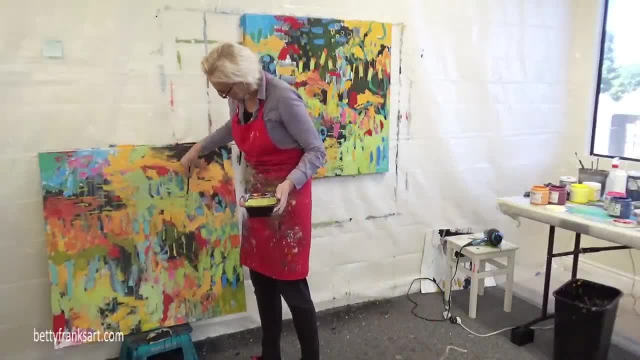 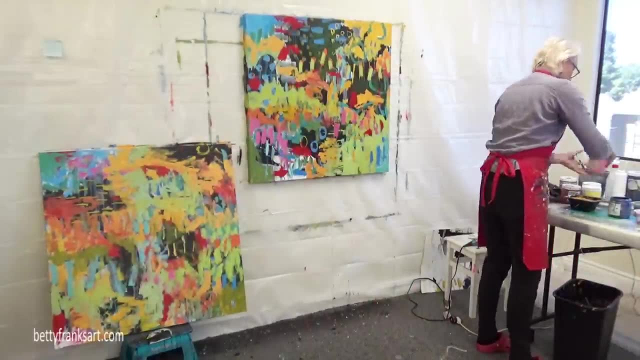 I would love to be able to do an example of a painting That's just one layer without mixing colors, And then to be able to show that side by side with a painting where I add a lot of layers and I mix my colors as I go. 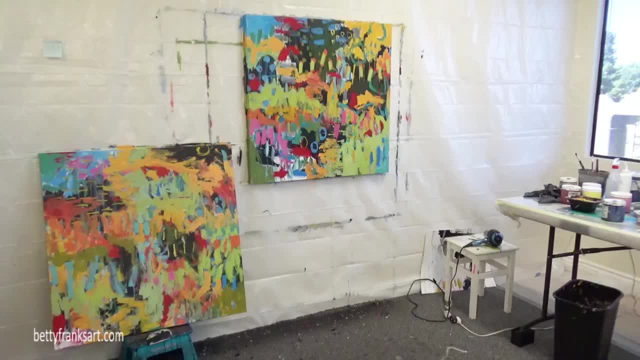 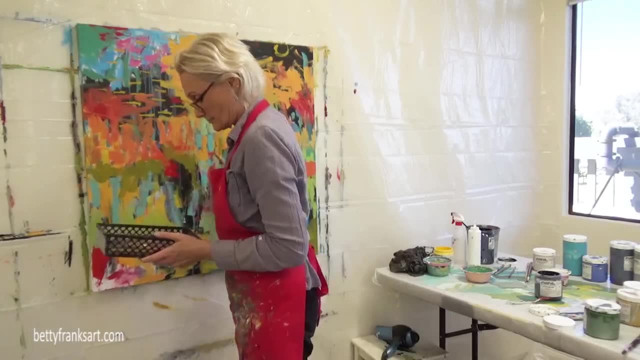 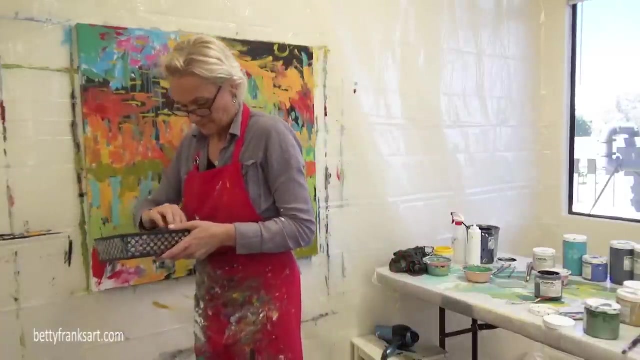 And I know I'm going to have difficulty with that, because I naturally gravitate towards mixing my colors immediately. Okay, so that one that was down below is the one that I ended up continuing on for this particular painting. I'm coming in here with my marks again, just like I did at the very beginning. 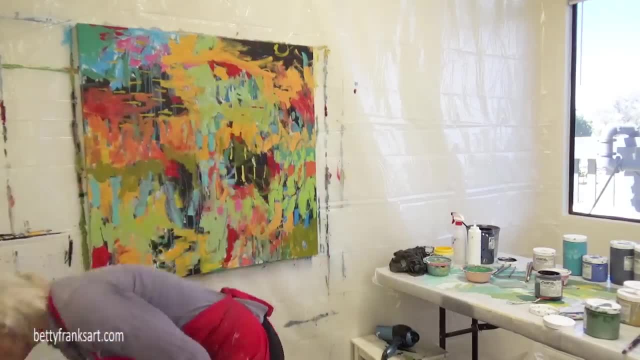 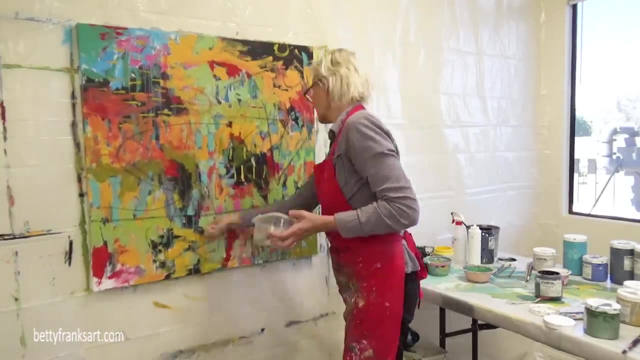 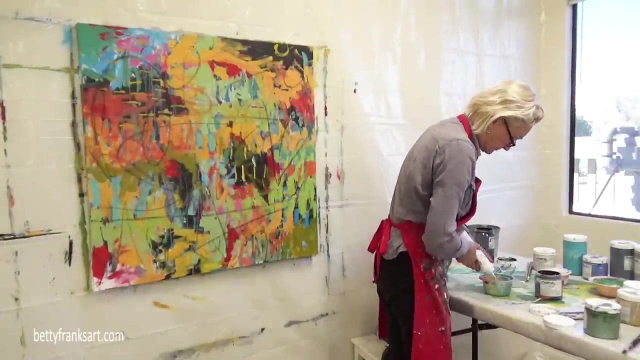 And the reason I do that is because a lot of those marks from the very beginning have already disappeared. And this is also my way of kind of reconnecting with this canvas. Coming in with that black, you can really see that right, Creating a lot more chaos. before I calm it all down, 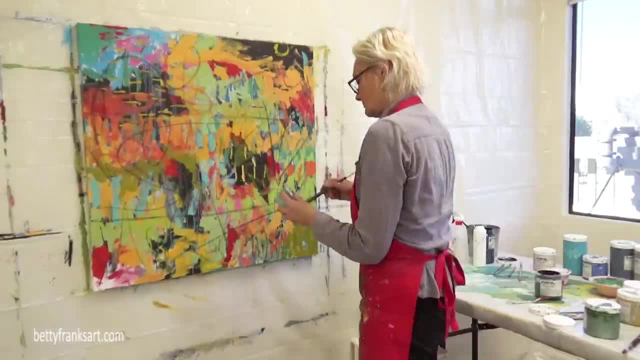 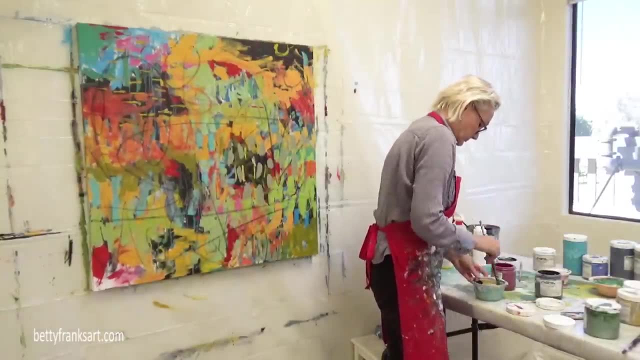 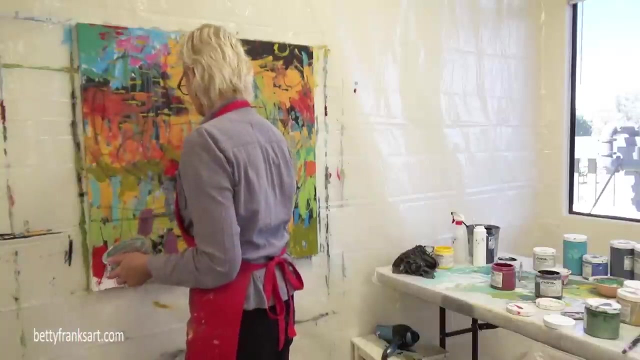 Now- I'm not sure if this is a different day- I tend to wear a different shirt underneath, but the same gray one when I'm in the studio, And I think I've got my black sweatpants on there too. So sometimes I have to check my earrings. often I have different earrings on, and that. 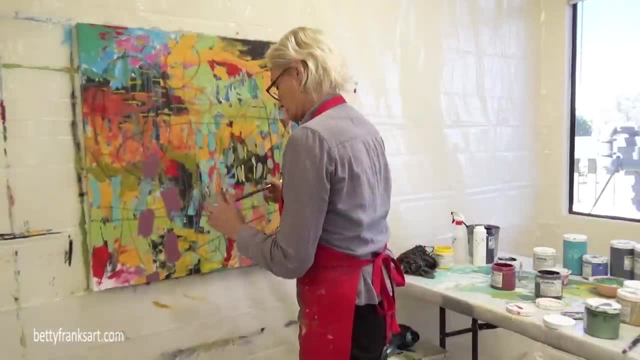 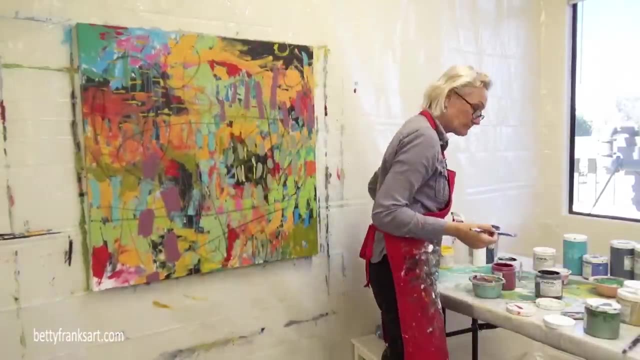 tells me it's a different day, or if it's the same day, Okay, I'm coming in with quinacridone red, But I don't know what I added. I added to it and I don't really like that color. 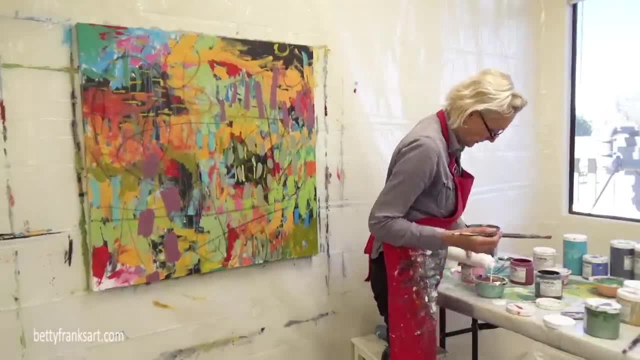 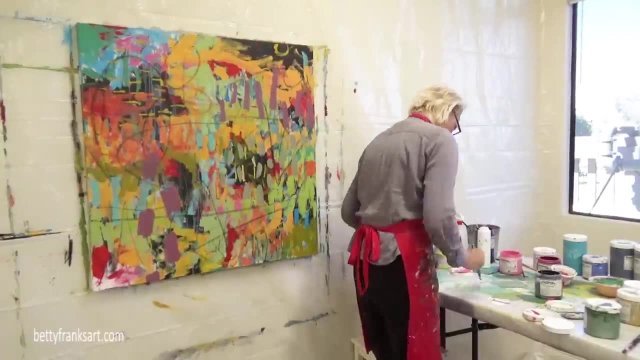 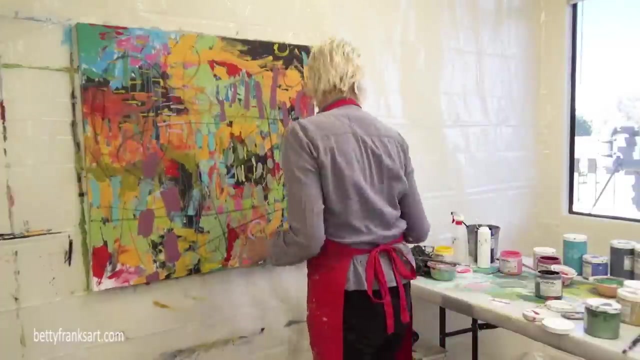 I think I was trying to change it a bit, but it's kind of dull for me And in the end this painting ends up being a very bright, happy painting And that color just wasn't going in the direction that I wanted. 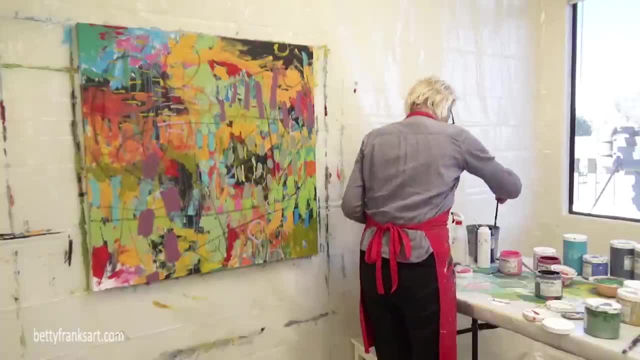 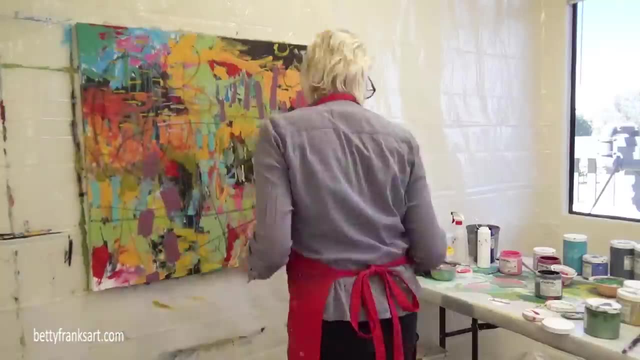 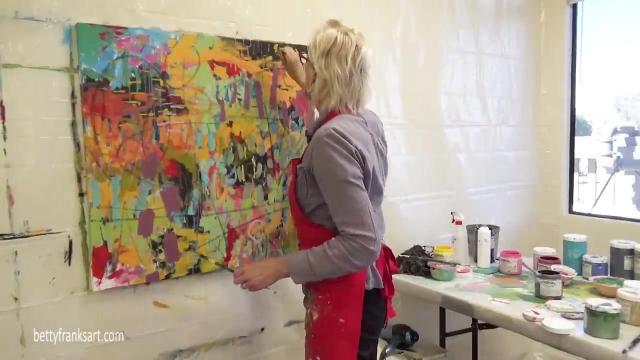 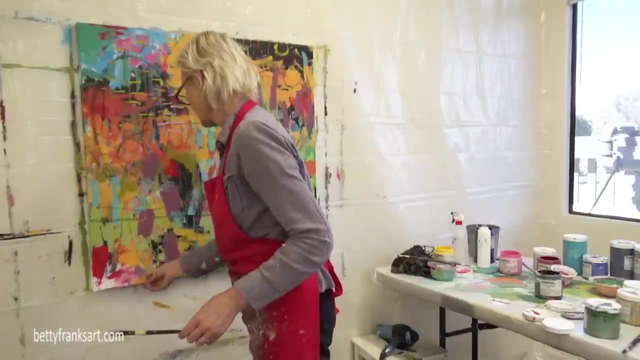 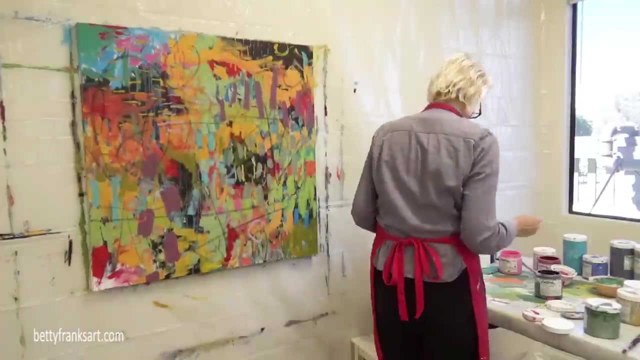 Coming in here with some pink And I believe I'm using my rigger again. I love making those finer lines with it. If you would like to learn from me and the way that I like to approach paintings, create paintings, how I loosen up. 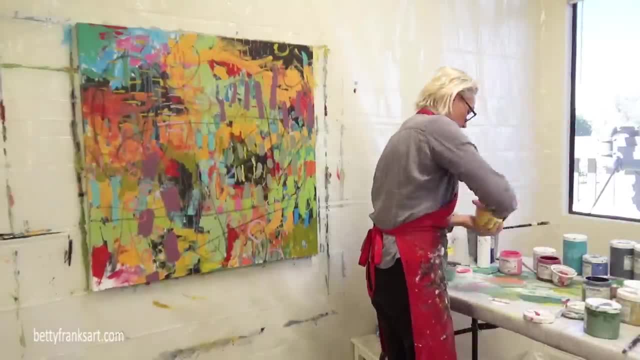 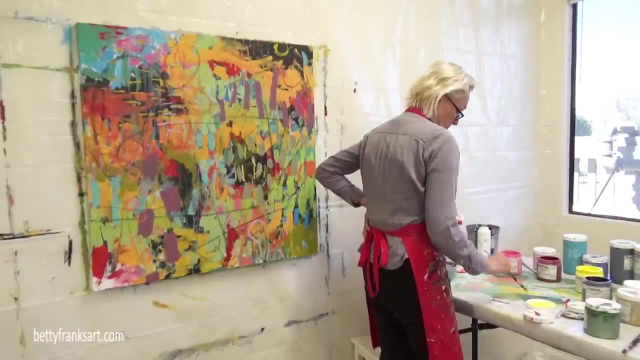 I've got exercises on that, Or how I make my paintings. I'm going to show you how I do that. I mix my colors. I've got an online course that is from an online workshop I did a couple of years ago. that is over two hours long and it's from a live show. 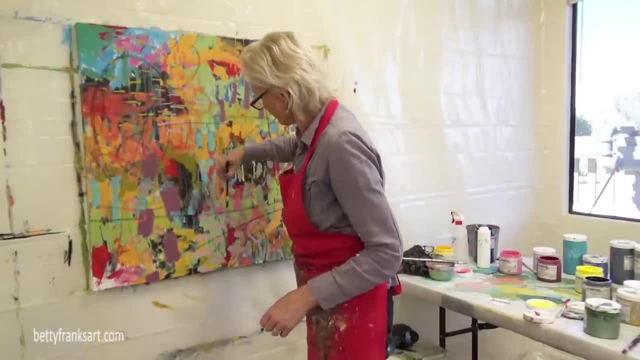 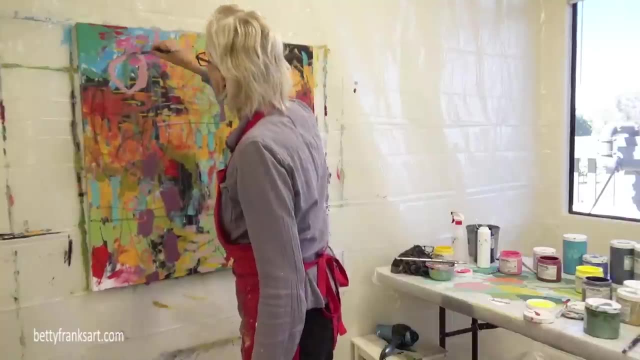 So you'll hear me actually answering questions from the students live and they're creating with me. Most of them are. Some of them are just watching it and then they're rewatching it later, but it's a two hour session and it's available. 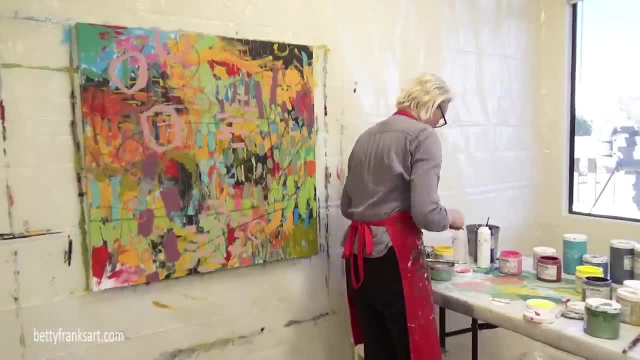 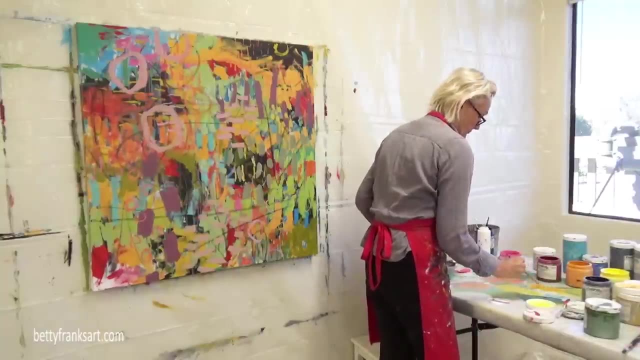 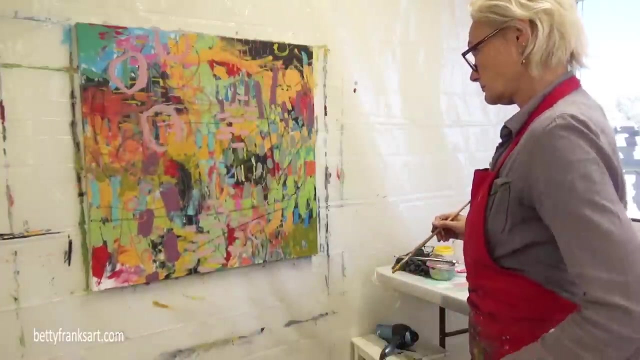 For immediate download, or I should say immediate access, which is actually on YouTube. So super easy. If you're watching this, you can also sign up to paint with me and watch it on YouTube, And the great thing about that is that YouTube allows you to change the language. 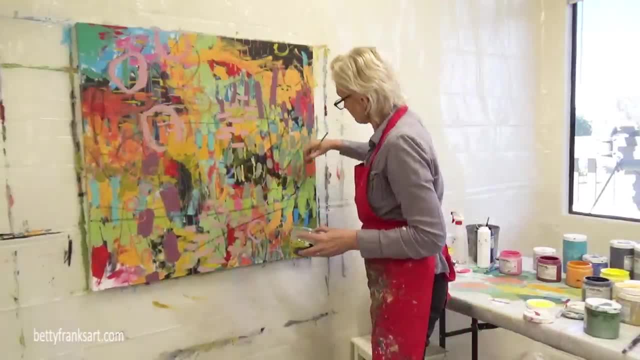 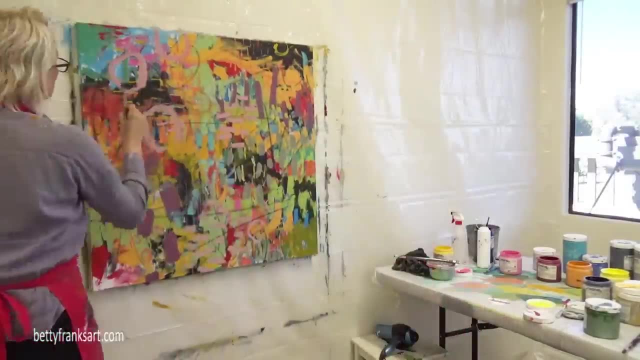 So if you're watching this from a part of the world where you don't speak English as your first language, you can change that in the There's a, There's a, There's a gear icon down below the video, and if you click on that, you've got some. 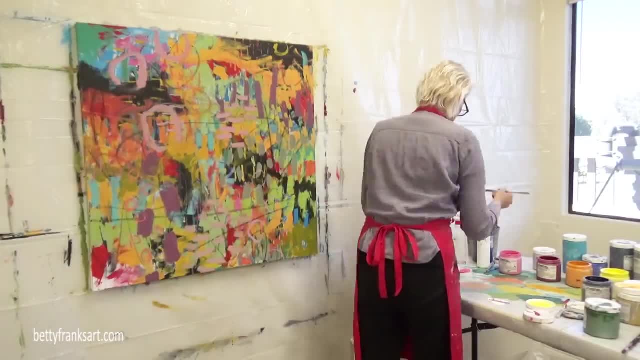 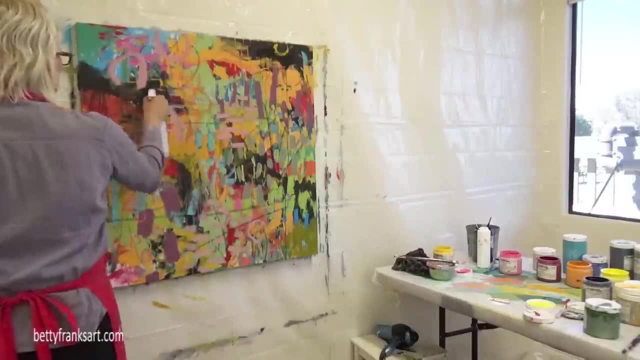 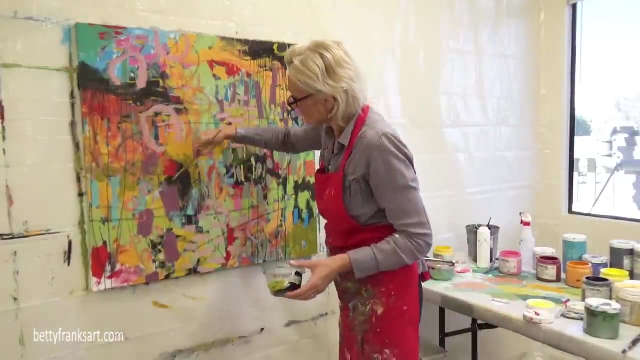 options and you can select the language option, and it should be able to Have a choice of choosing one that that you would like. So that works also for my online course. I'm going to put a link down below for you or, if you're not able to find that link, just. 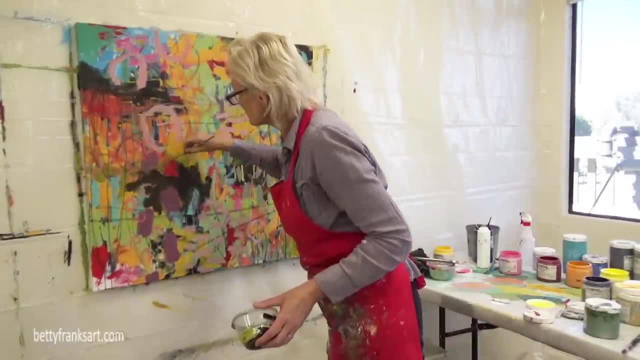 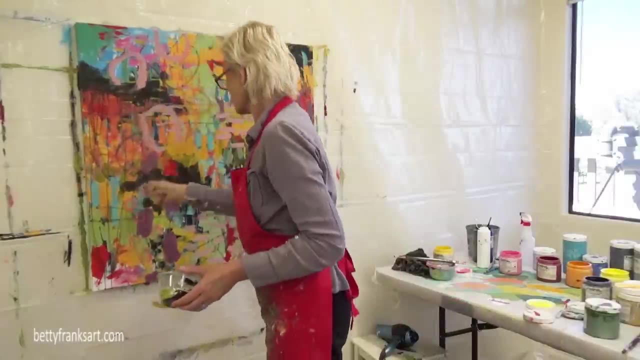 message me. Happy to Send that. Send that to you Now. I was hesitating there a bit because I'm coming in with black and I normally don't do that, Or I don't like to do a whole lot of that after my initial layers of black. but I covered. 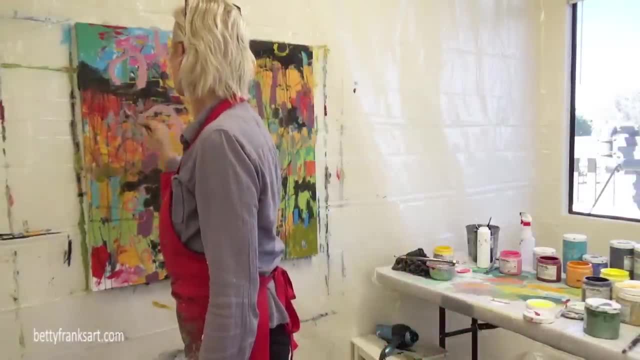 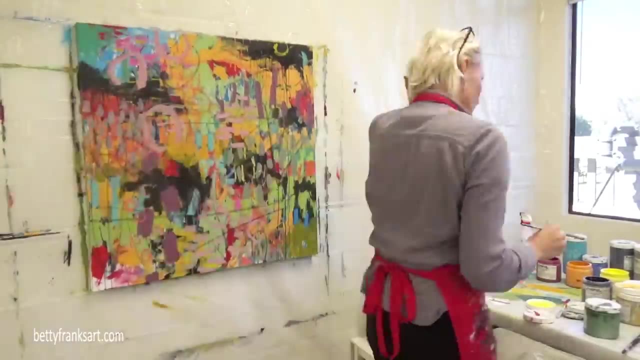 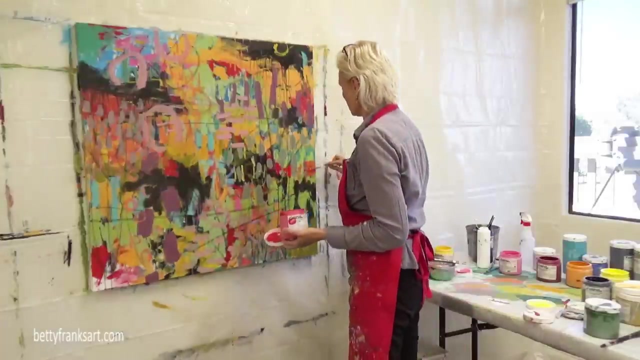 up so much of it that I wanted to bring it back in, And the reason I love the black is I think it just adds so much depth to the painting. Now, a lot of this will get covered up. I know I know a lot right now, but it will get covered up. 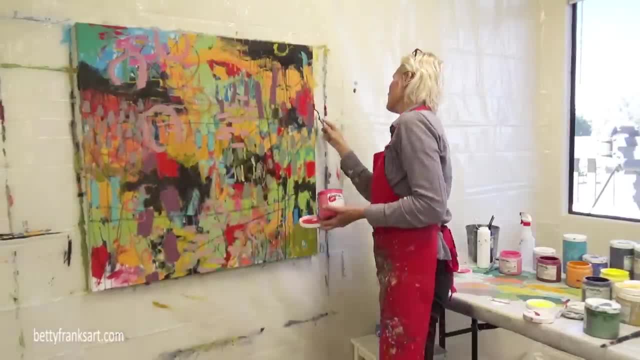 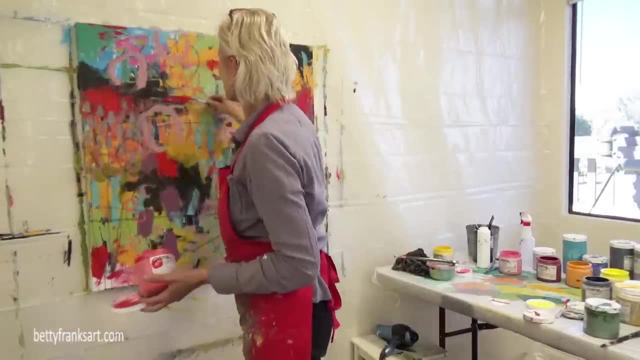 I'm looking at one on my I'm looking at the final piece on my phone and you know what A lot of it, almost all of it, gets covered up. but I bring it back with like more of a darker gray because the black was just not working with the overall piece, but the gray 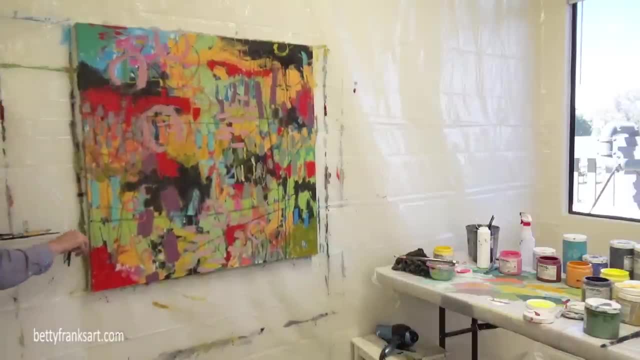 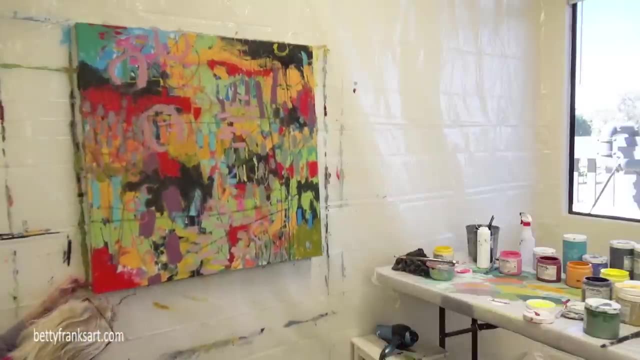 worked much better. Now, here I think I've got a palette knife. Yes, I do. So I've got a palette knife in my hand applying the paint a little bit differently, Just like in the beginning I was using that scraper, and here I'm using a palette knife. 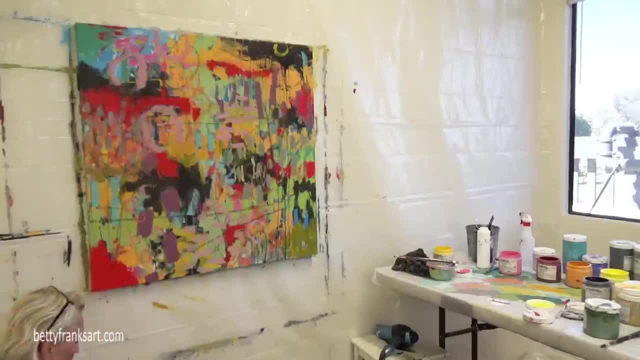 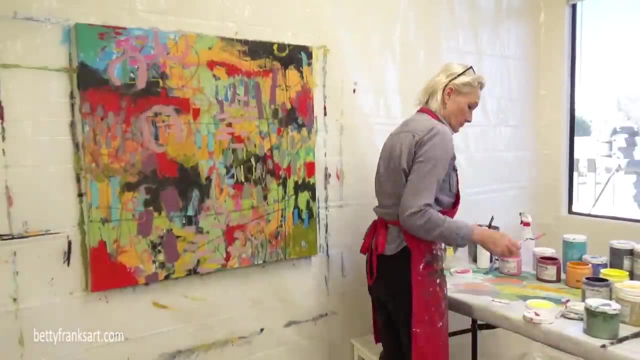 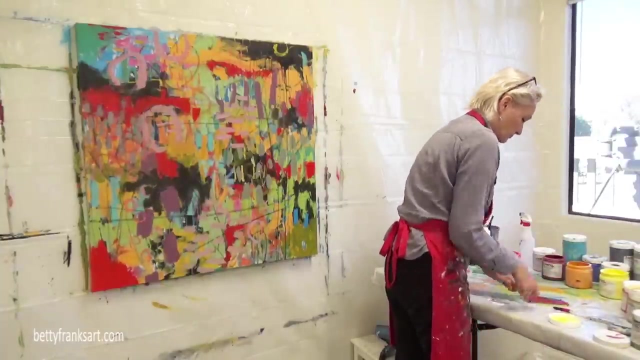 to apply the paint so that they're not always brush strokes. I like to bury it a little bit. The great thing about a palette knife is you don't have a whole lot of control of how it goes on, And that's something that I like. 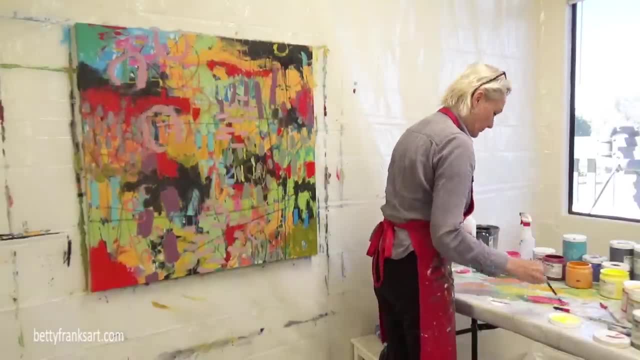 I like having elements of color. I don't have a whole lot of control of how it goes on. I like having elements in my painting that I don't have full control over. you know, kind of like the drips. I love those because there's not a whole lot of control. 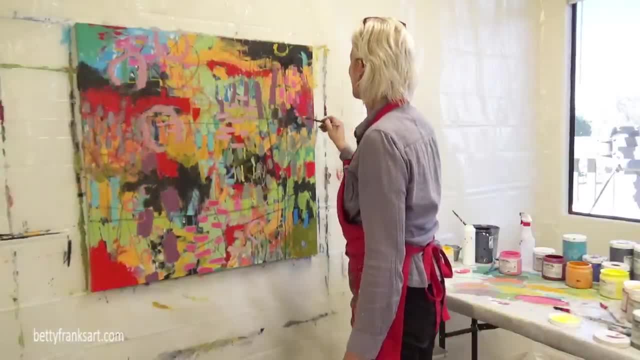 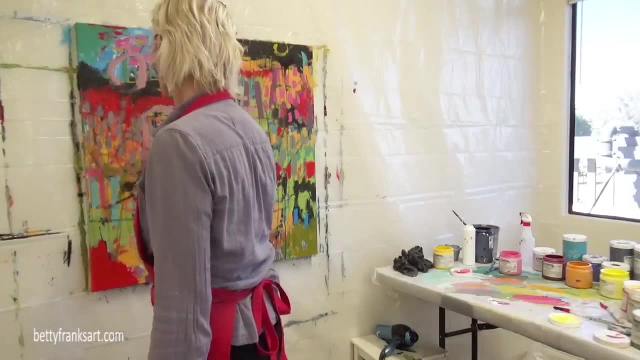 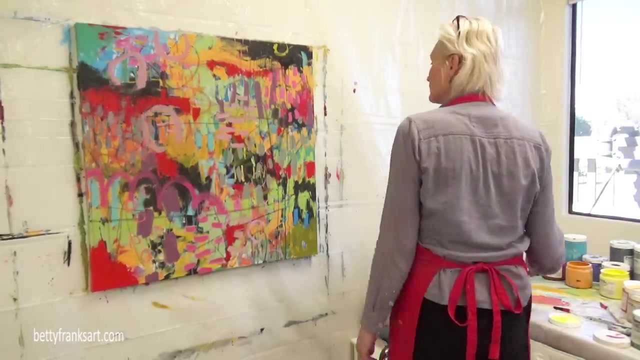 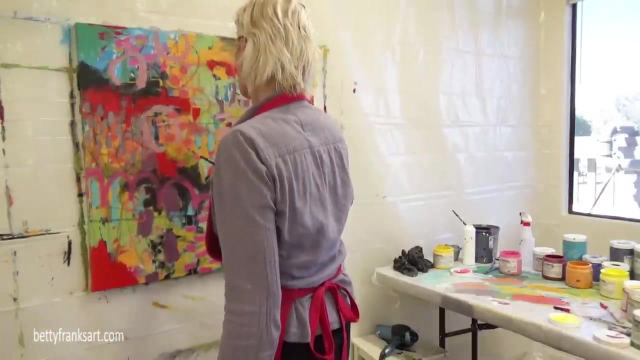 I love all the scribbles because they're not intentional. They're not. you know something that I clearly said: oh, I want a line to go here. I don't know, I don't want to go there, I just do what I want. 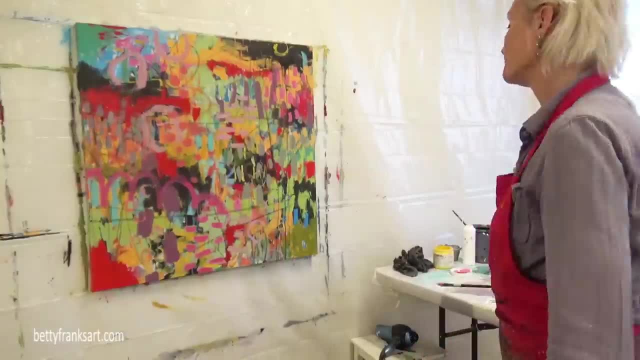 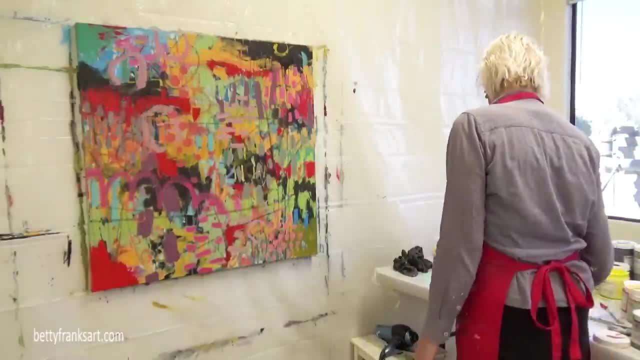 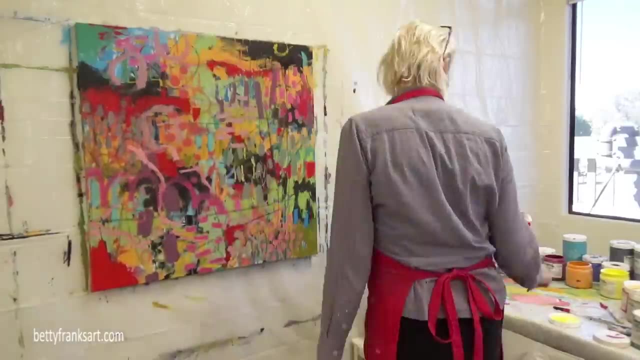 I don't know, But I do like the idea of having a little bit of color to go with the painting. This painting ends up being, I want to say, a warm color, but actually it's a combination. It's got a lot of greens in it, a little bit of teal and then definitely pinks in it. 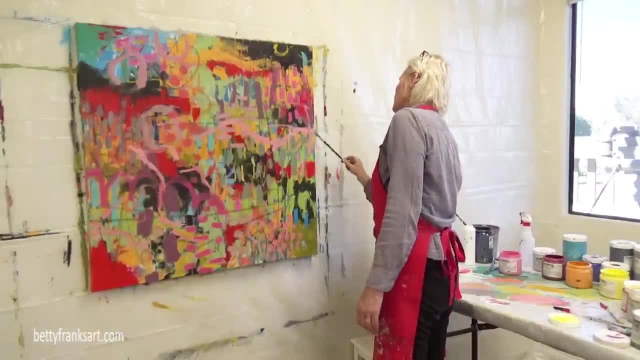 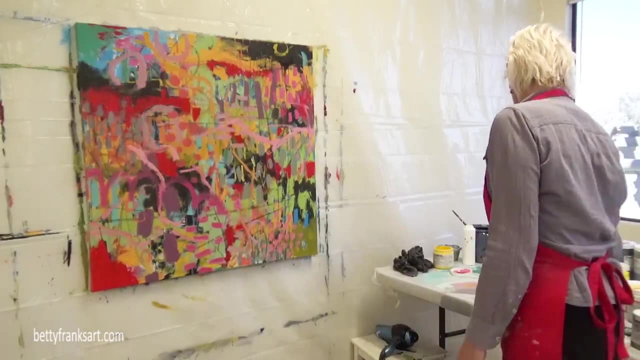 And here what I'm doing is again some marks that are not perfect circles or lines. I'm just trying to be realistic. I'm just trying to be realistic horizontal, vertical lines. I'd like to come in and just kind of throw down some. 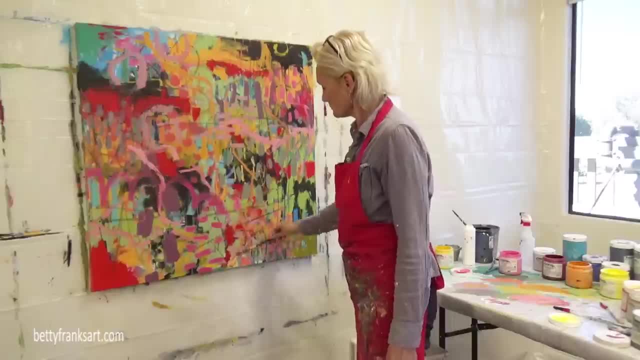 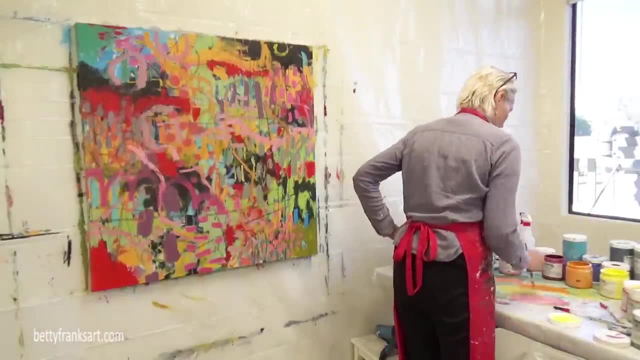 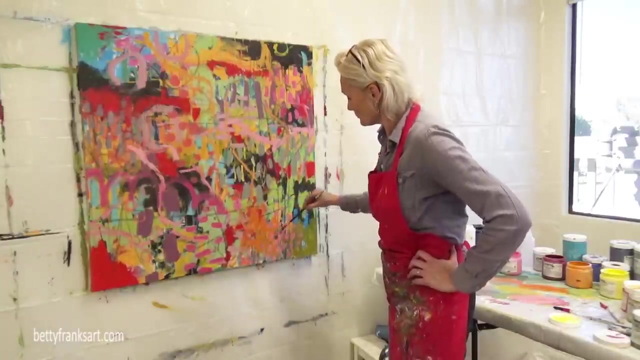 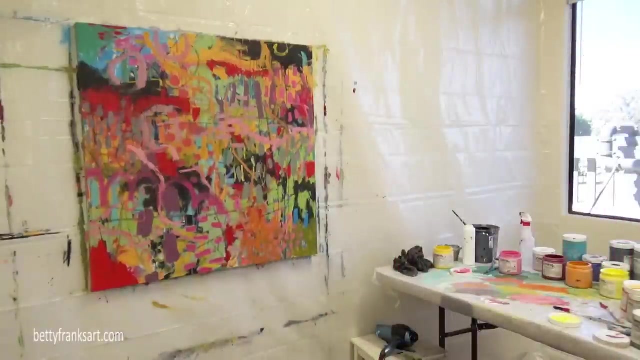 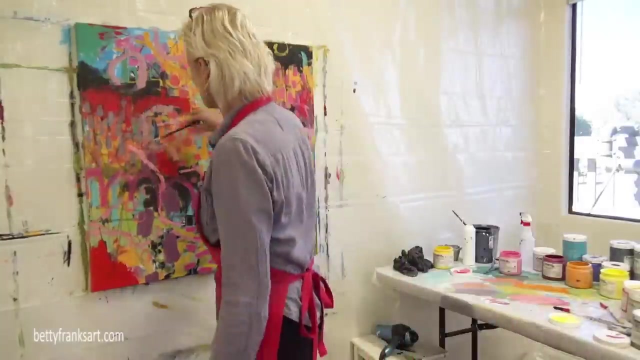 color haphazardly, I guess, is what I'm trying to look for, Making it feel more organic that way. So here I'm filling in and I'm saving some of the, some of the things, that some of the dots, or I can see something down towards the bottom of that, Not covering up everything. 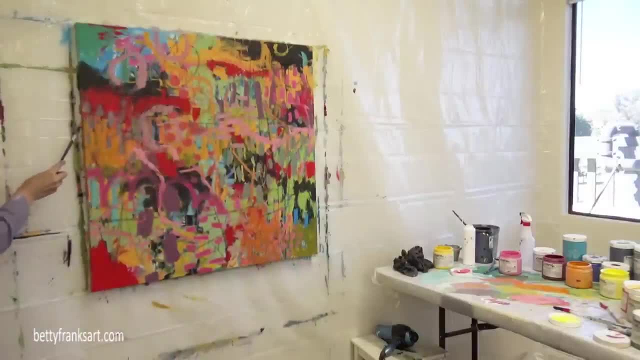 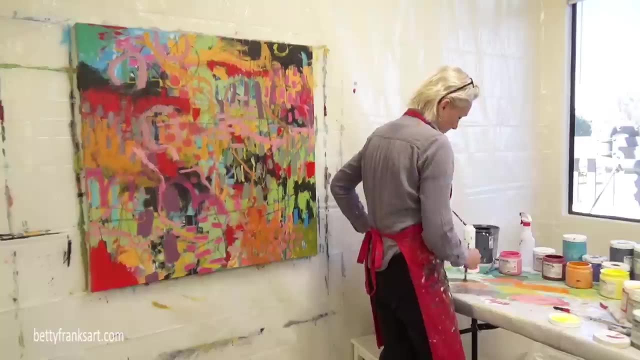 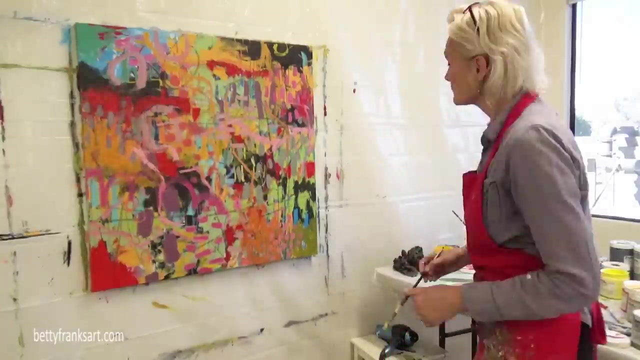 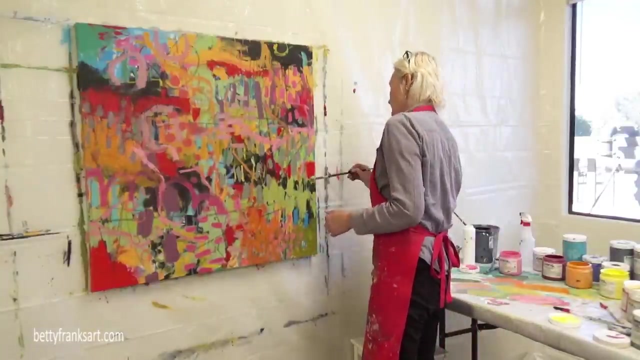 Saving some parts. For me, each painting is such a journey. It's, you know, going from those early stages of total chaos and craziness. even right now it's still a lot of craziness happening And it goes on this journey of quieting down and some areas you know still stay still. 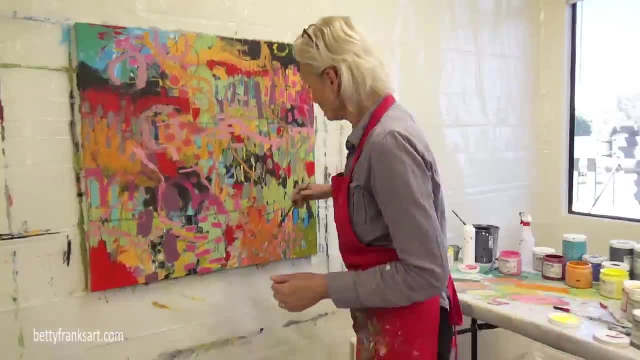 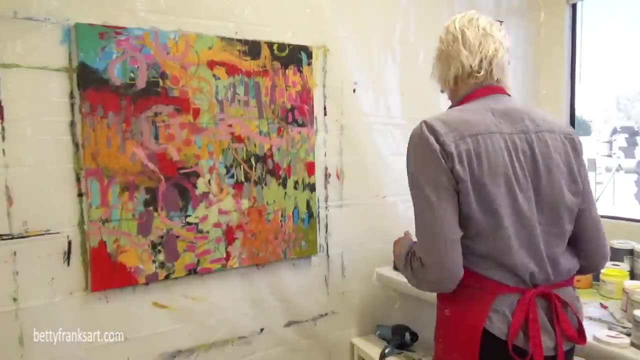 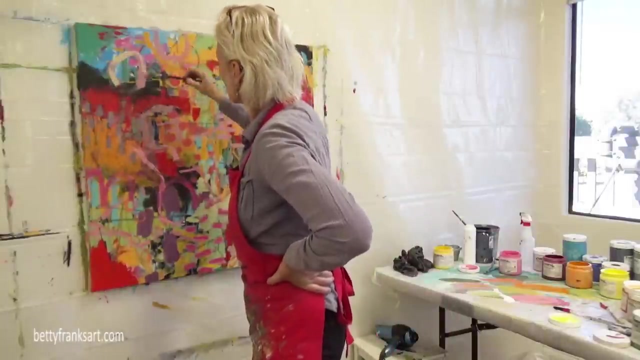 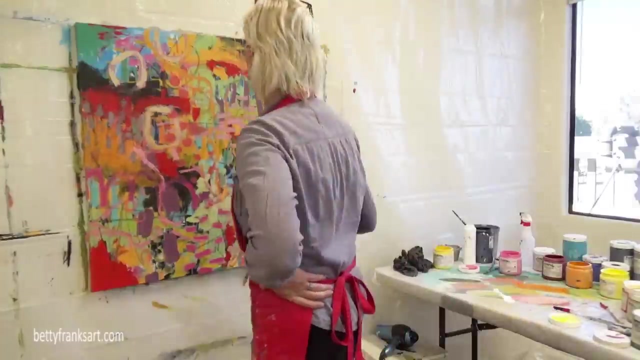 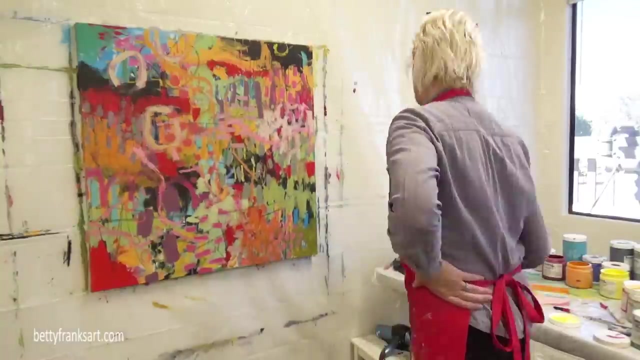 will be kind of crazy, but a more tamed crazy is the way I'd like to describe it, And so you know I just love each journey, Each journey that each one takes. It's just very fascinating to me. These are some of my- what I'm considering- larger elements of circles that I just did. 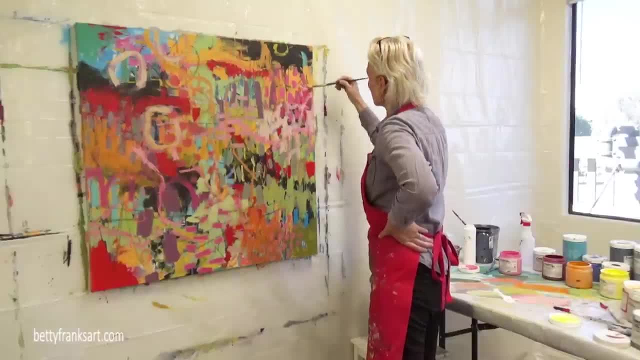 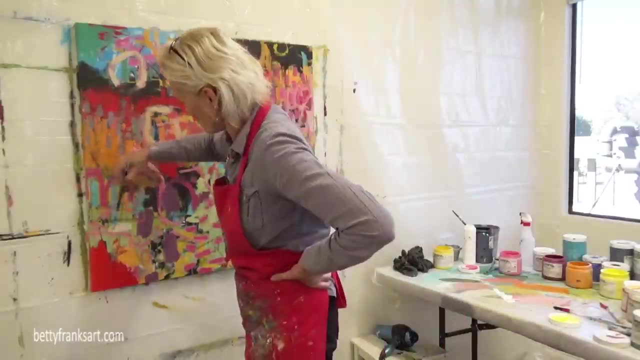 Sometimes when I look at my paintings and I can't figure out what's going on with them or what's going wrong with them, Then I tend to look at some of my older paintings, Some of my older pieces, And in my other studio I had a whole bunch taped up on the walls and I haven't done that. 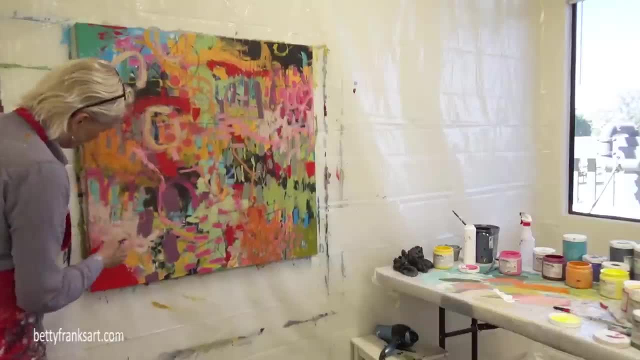 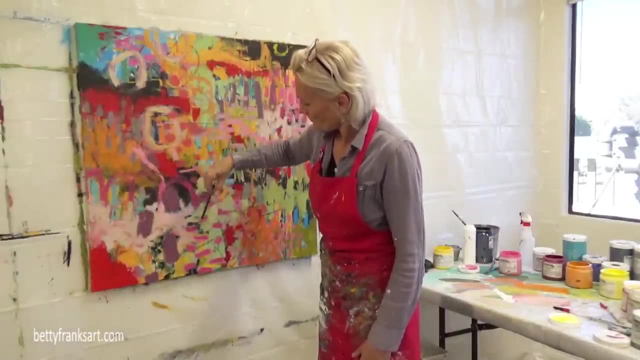 here, yet I don't know if I will. Sometimes I feel like they're distracting to me, But other times, especially if I'm working on something that I want to use as an inspiration, I do like bringing it in so that I can reference it. 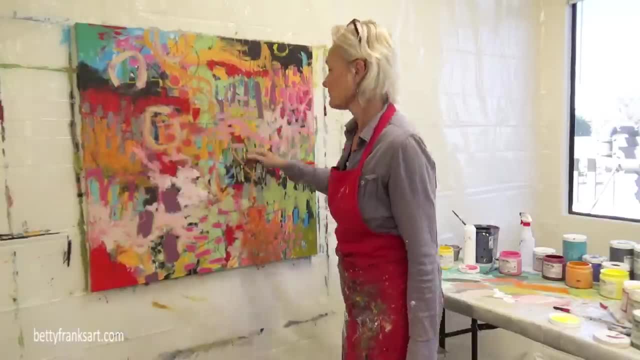 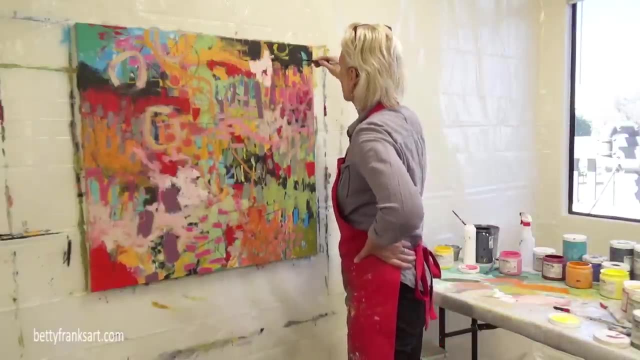 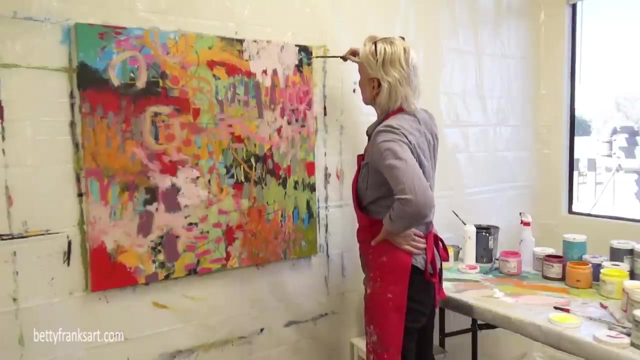 But when I, when I'm feeling stuck, it usually is because something's not working about that piece, And oftentimes it'll be because I don't have maybe some larger elements in it or maybe I don't have a good balance of, you know, color in it or shapes or the sizes of those. 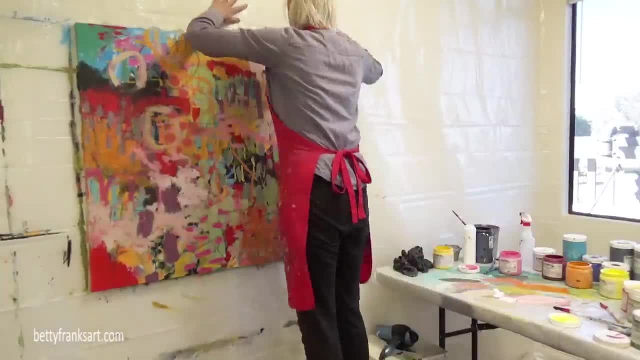 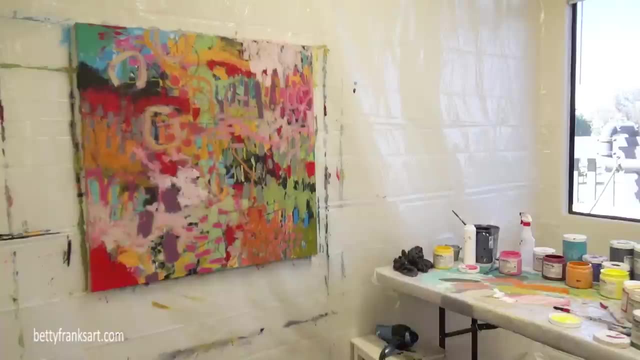 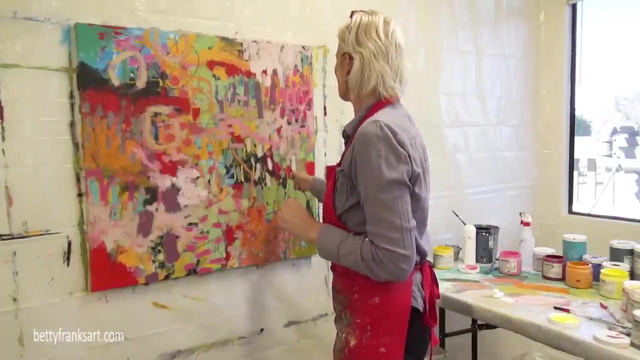 shapes or values. you know, right now I'm working on my lighter values, So bringing in light values. So it's it's all about problem solving. it's, for me, it's trying to figure out, you know, why isn't this working. 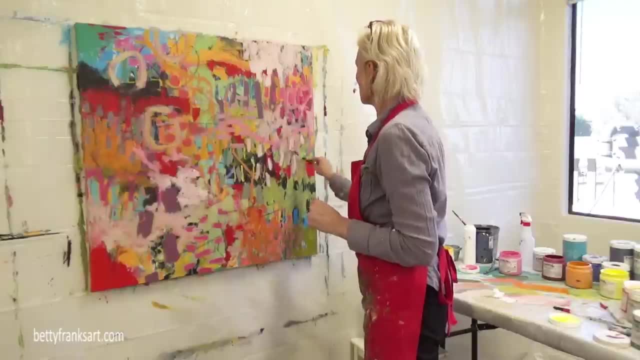 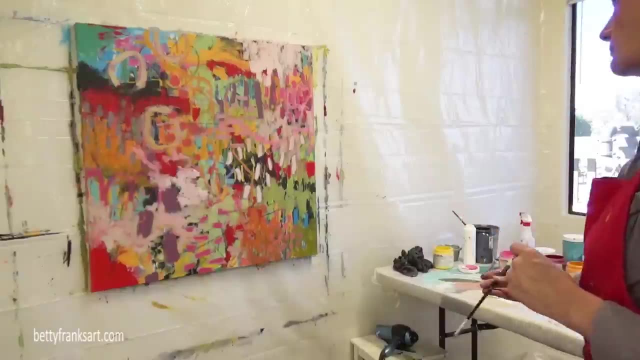 What can I do? What can I do to make it work? What kind of marks can I put down? What kind of color can I put down? And you have to remember that each mark, each color you put down informs the next one. 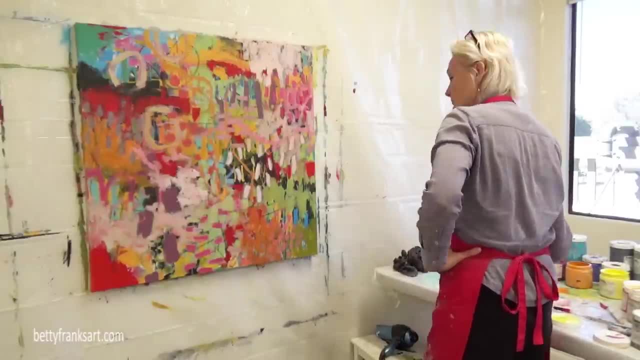 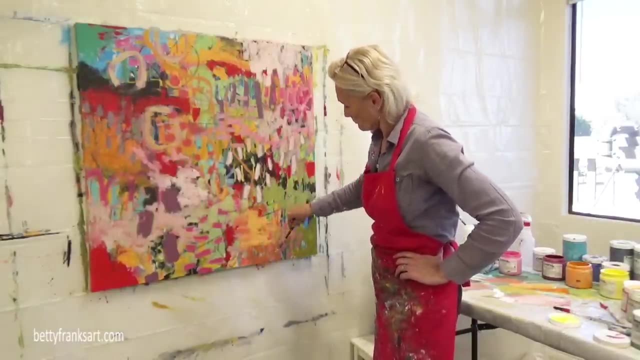 And when you put down a mark and a color, it may not work with what you had already done. So that means redoing some areas, And so it's that constant push and pull throughout this entire process for me. You know okay. 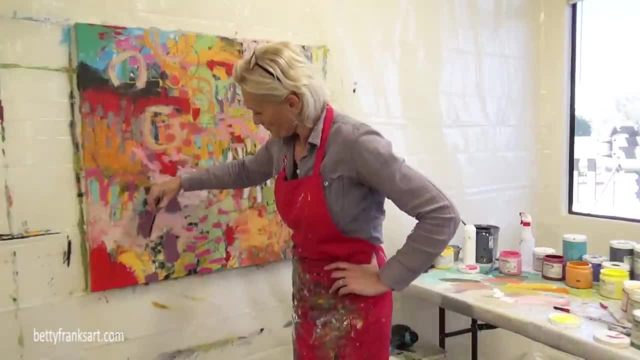 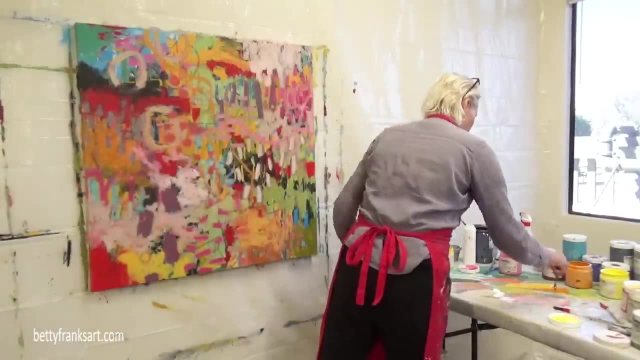 I'm going to put down these marks. Okay. How does that work with the other marks that I already put down? Or how does that work with the colors I've already put down? It's a dance. It's going back and forth throughout the piece until I get to a point where I say okay. 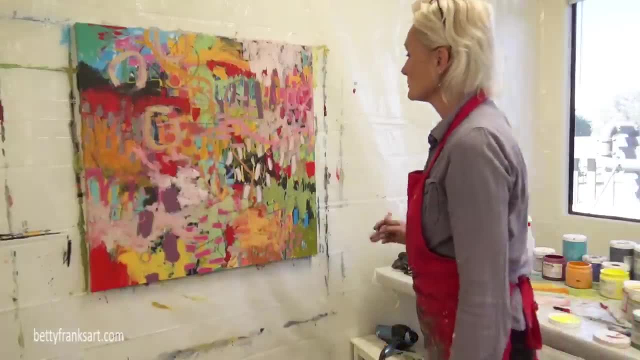 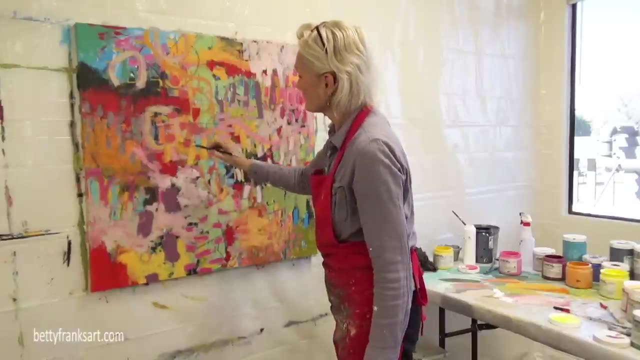 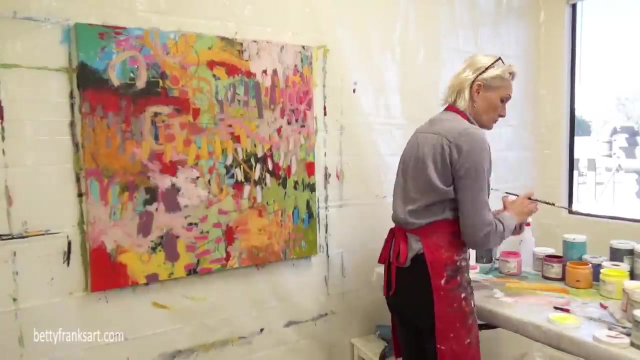 I don't know what else I could possibly do that will make me happy, And so that's when I know that I'm done with the piece. Okay, I'm going to put down these marks, Okay, And then, Looking at it right now, at this stage, you know there's my eye is going all over the 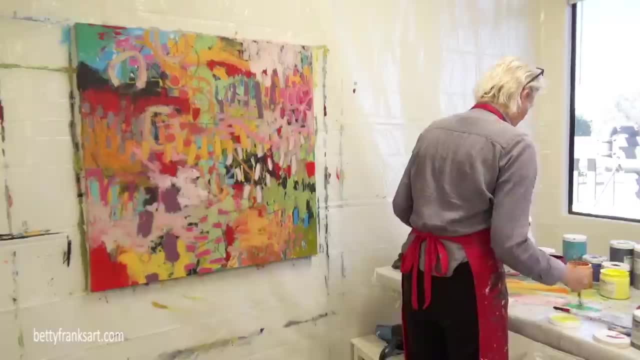 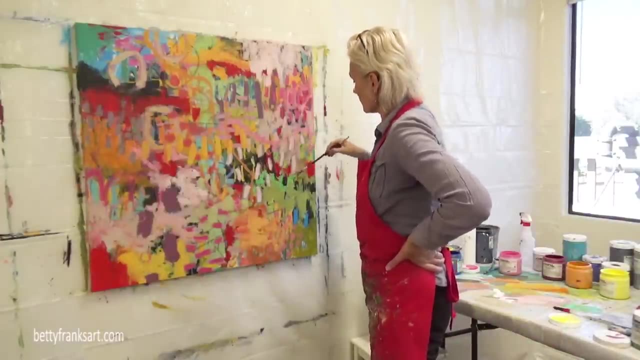 place And it's landing all over the place In the areas where I know it needs work. And that's usually what I'm looking for, and not so much what I like about it, but what is not working about it, so that I can continue to solve that problem. 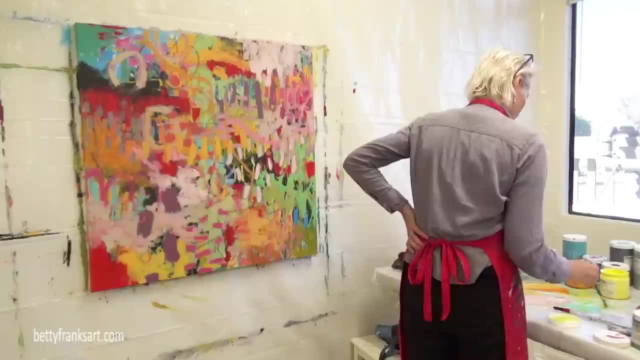 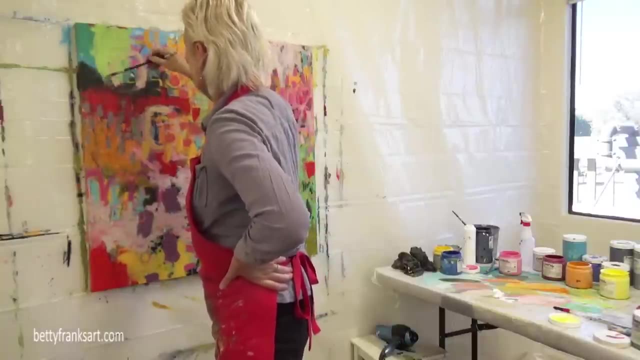 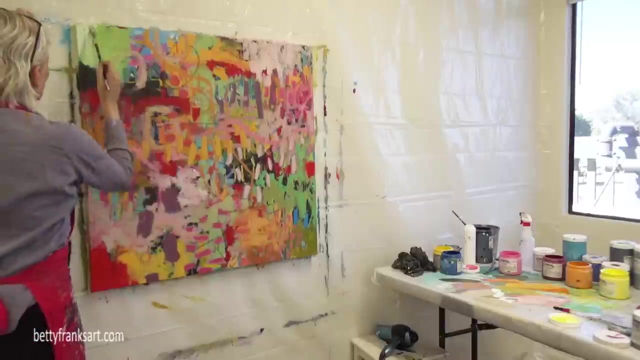 And in life in general. I tend to be a problem solver. if there's an issue, it's like: okay, okay, let me research, Let me figure something out, Let me think about it, Let me, you know, come up with some plans, And when I'm creating my art, that tends to be a shorter window. I don't. 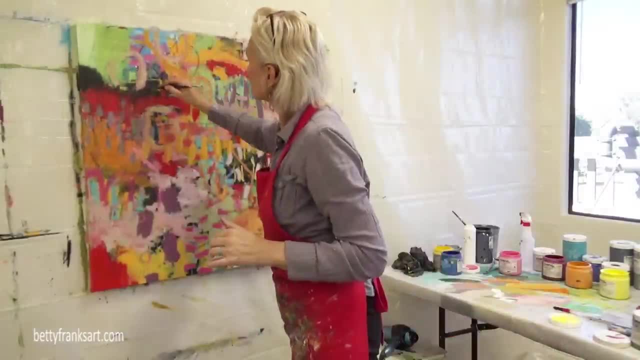 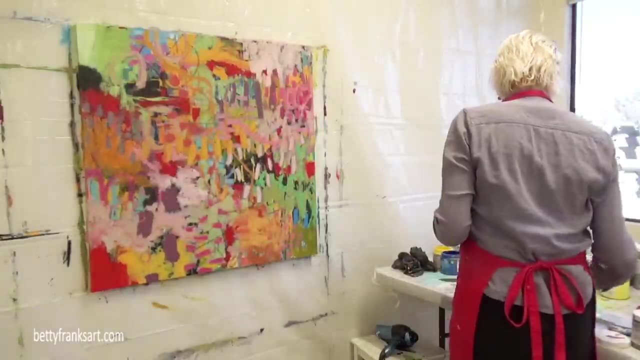 go off and research, And I'm not one to sit back and stare at it for too long and figure out: well, what's my next move? I you know, as you can tell, here, I just keep going and going until I'm happy. 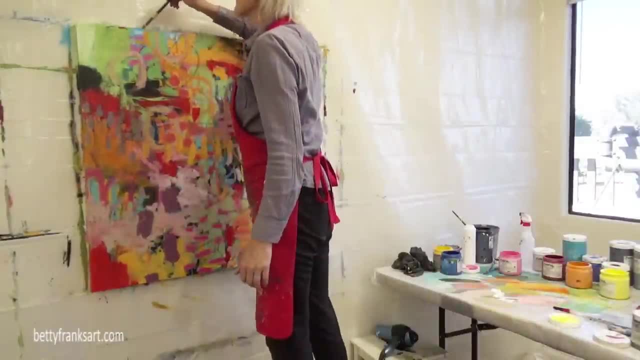 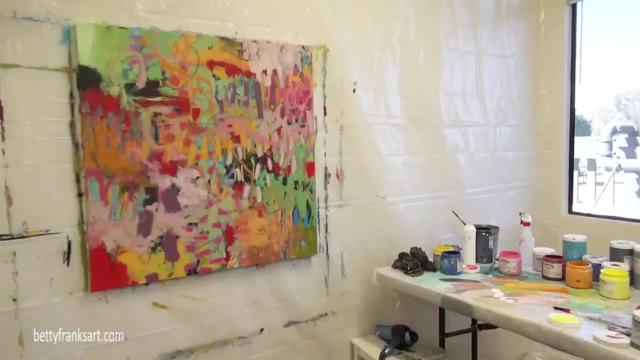 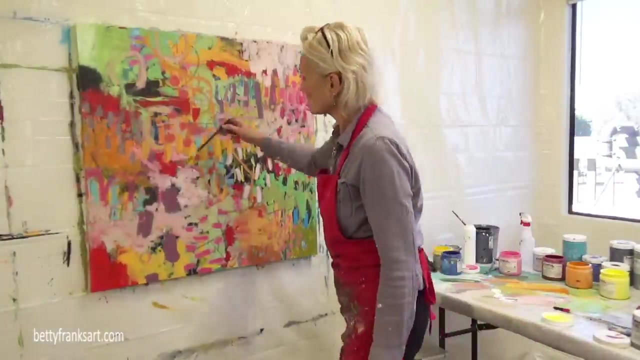 and I'm done with it. I know there are some artists, you know, because of the type of art that they create, they do look at it for a long period of time to decide. you know where it should go next. It's different for everybody. I think one thing I've really learned, as you know, as 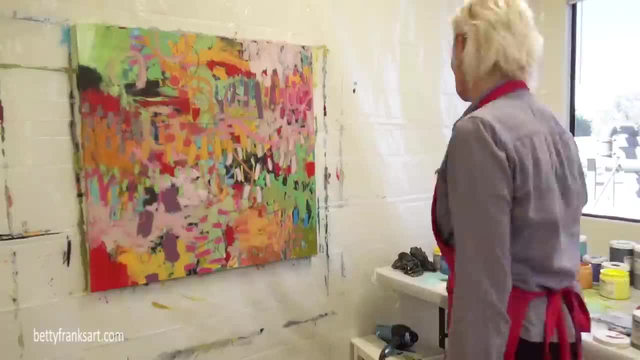 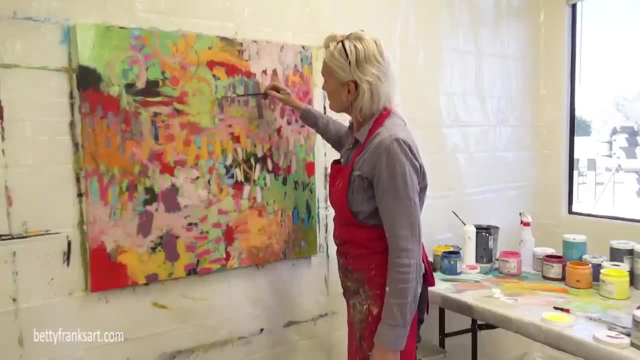 the years go by of creating art, is that we are all so different and so unique, And not only in the art that we create, but in the way that we approach it, in the way that we select our colors, in the way that we put. 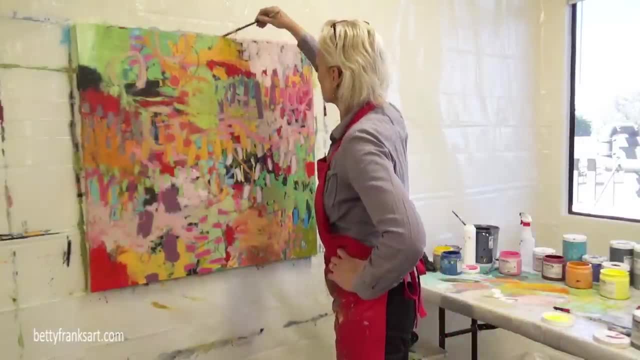 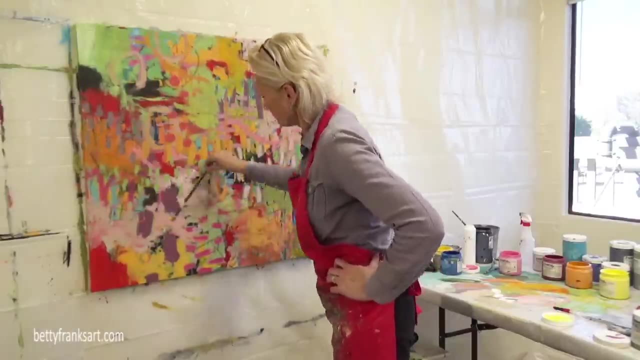 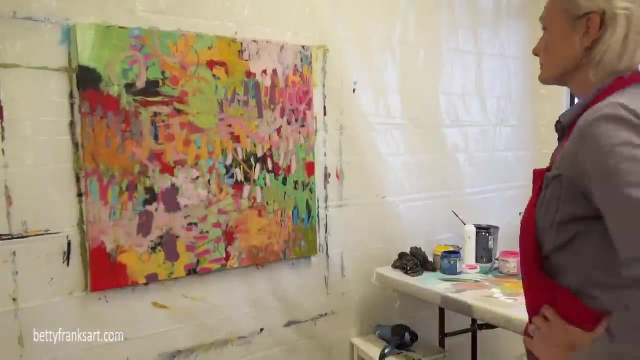 our compositions together, And it's just so fascinating to me because there are so many different ways that you can be an artist and so many different ways that you can express yourself as an artist, And we are all so unique in that regard- you know, as unique as a flower is. 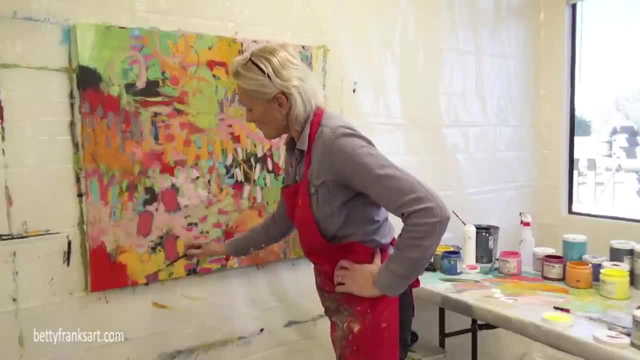 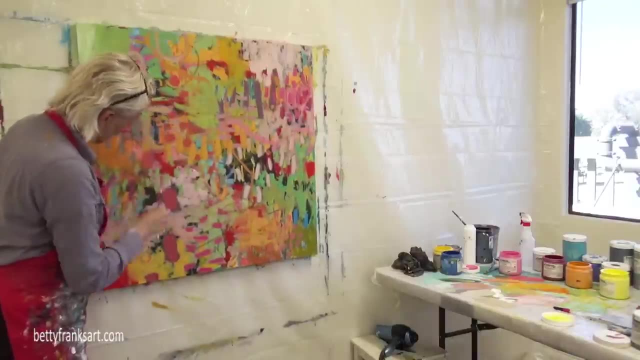 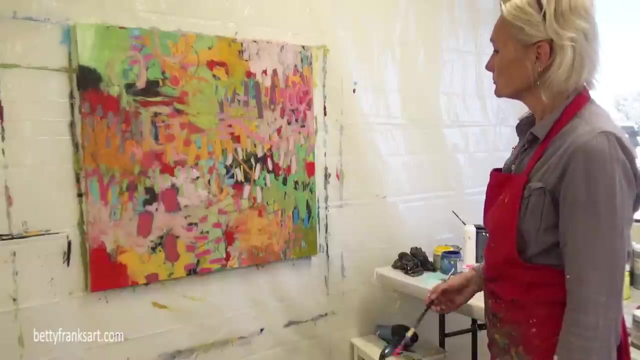 And so you know, I guess I just want to encourage you to keep creating, even if you are questioning yourself or you're unsure about yourself, just keep on doing it. So here you know. when I get to this stage, I start to slow down a little bit. 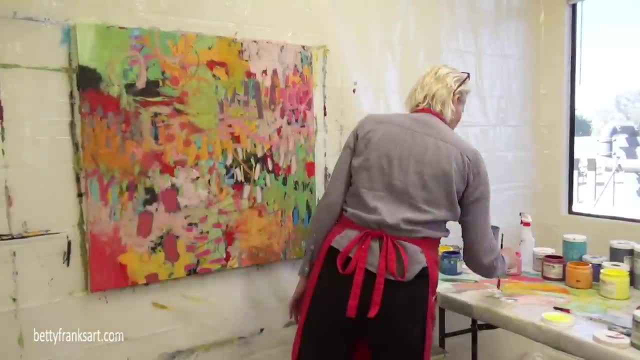 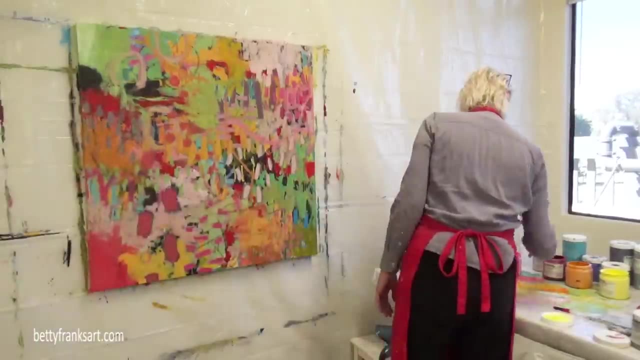 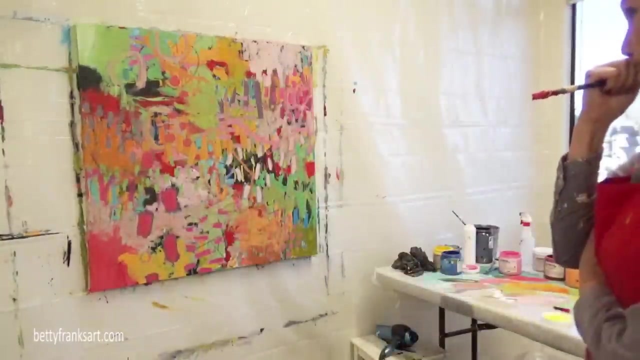 because I'm thinking more. I'm trying to- again going back to that, you know, solving problems, So I'm looking at it overall and then I'm narrowing down. okay, where you know, what should I work on next? What's the next area that's standing out to me that needs addressing? 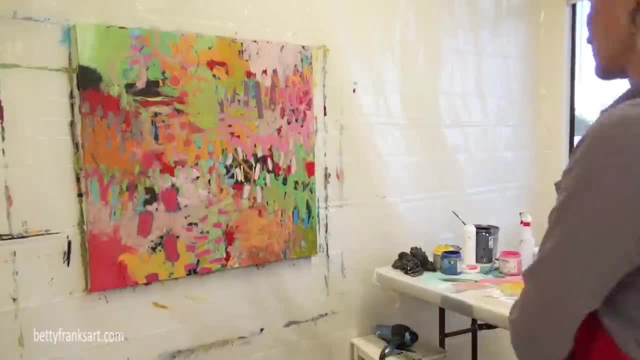 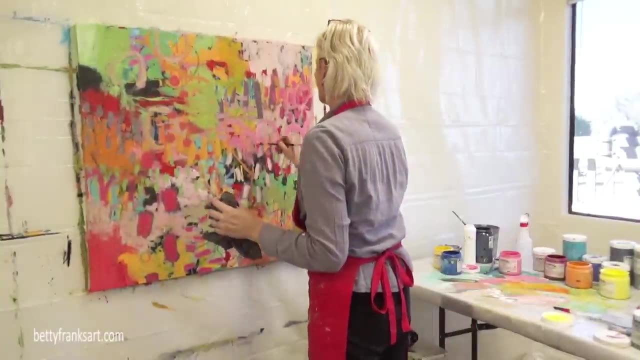 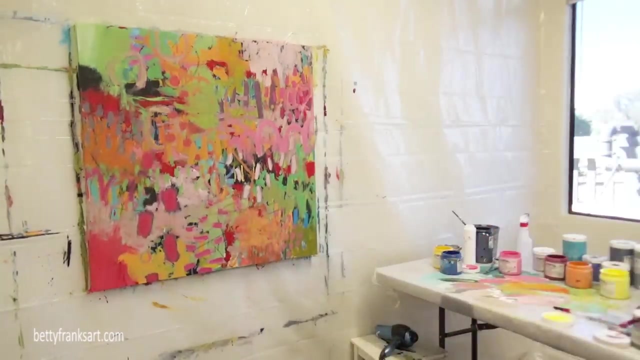 I love these loop loop-de-loops that I call and they remind me of of little white picket fences in the neighborhood walks And that one. I didn't like it And so I rearranged it a little bit And I had done that over on the left side, but that ended up. 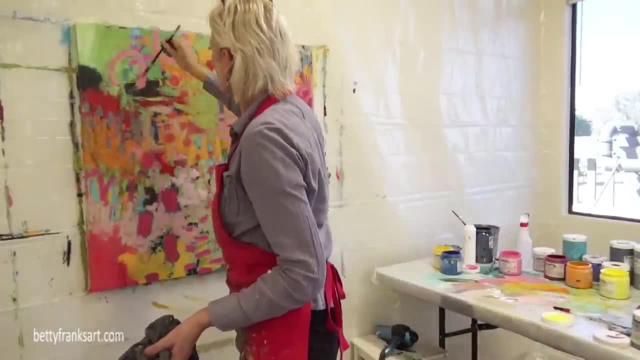 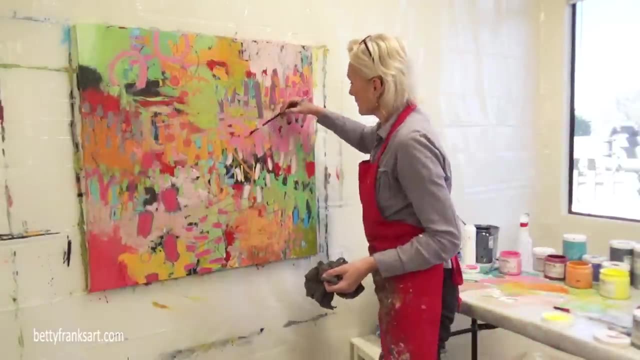 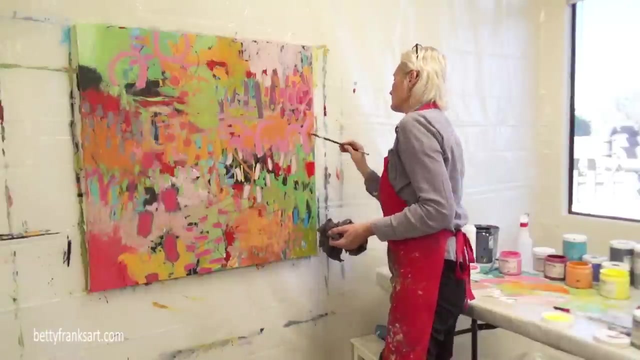 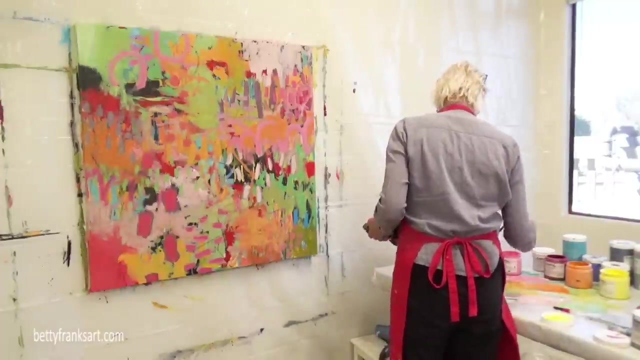 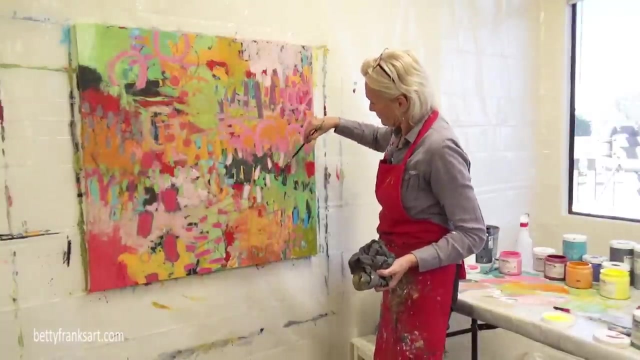 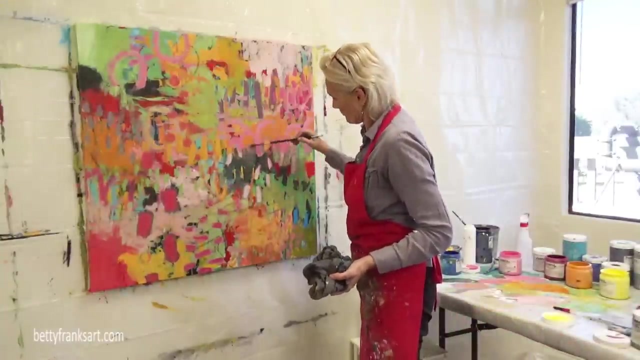 getting covered up a bit And I think it works better on the right side This painting ended up being at going to a gallery. I joined a new gallery in Morgan Hill, California, which is just south of San Jose- It's the next city south And they are called Calibri Gallery And I'll have their information. 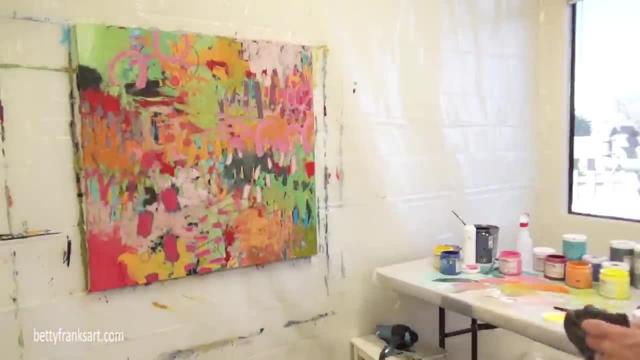 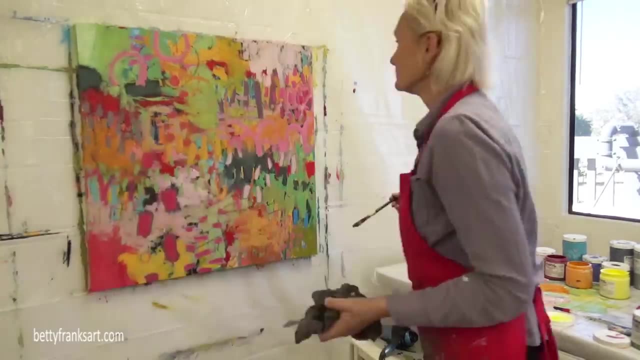 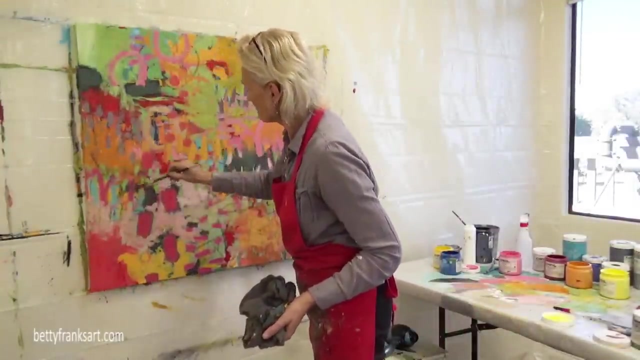 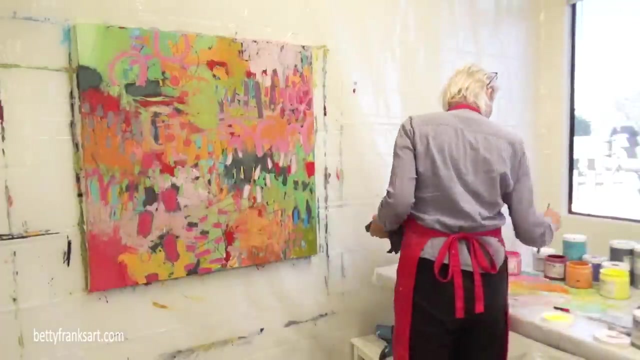 in my show notes down below. But it's so wonderful to to join up with another gallery I'm also with Curated by the Sea in Santa Cruz. So this piece and another one the same size and then two smaller ones are at Calibri and Morgan Hill. 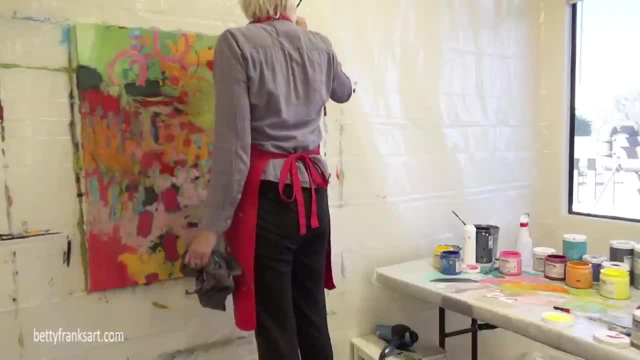 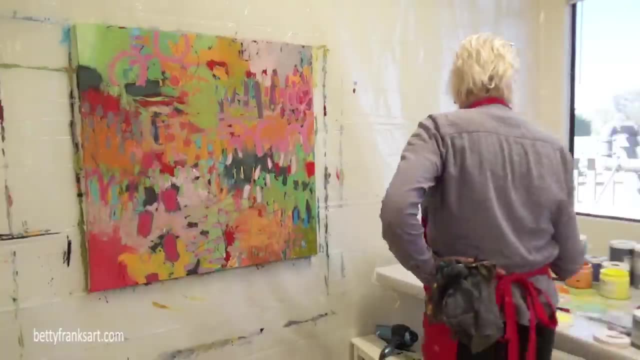 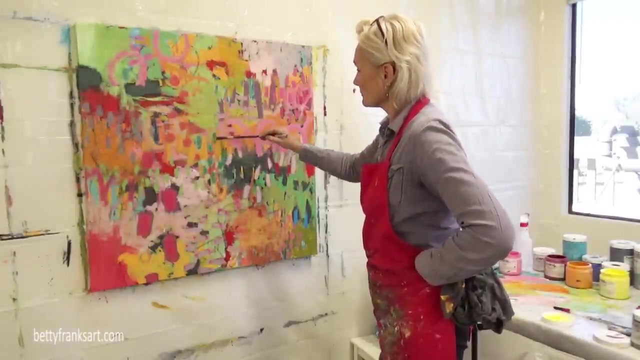 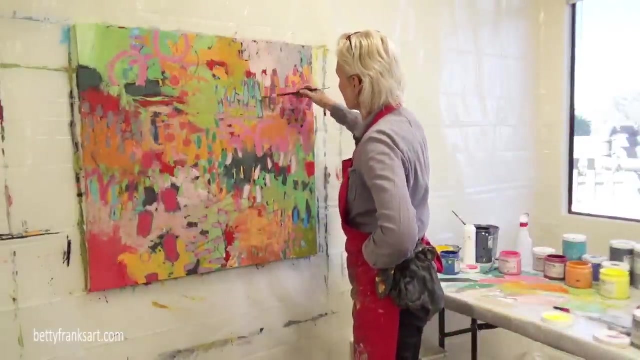 All right, moving right along here And as I was chatting before, so some of those really dark areas, I did come in with a darker gray, green-gray color. I think works better with the overall as opposed to the black. I think was a little bit too jarring. 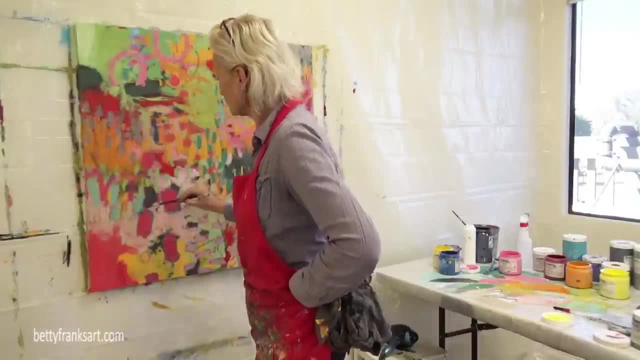 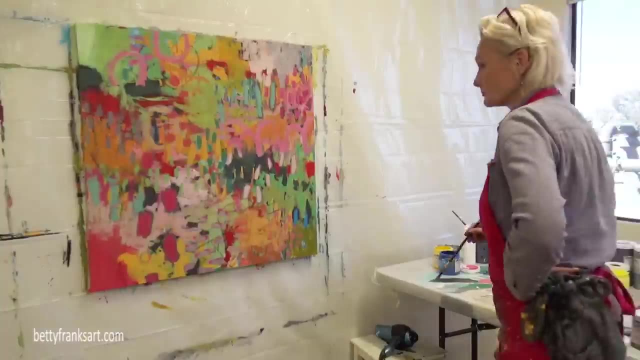 I do love that teal I just put down. But I'm looking at my final piece and I ended up covering the teal at the top there, Not sure why I kind of like it. I probably had a good reason for it. 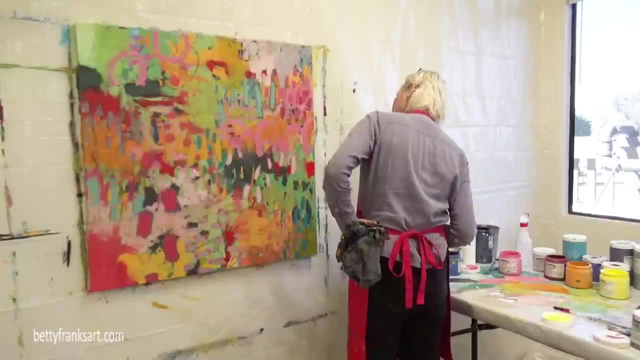 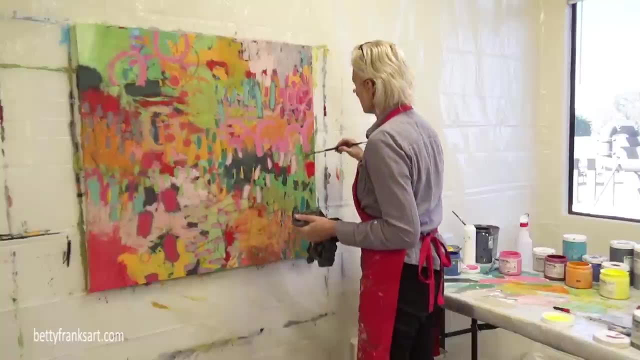 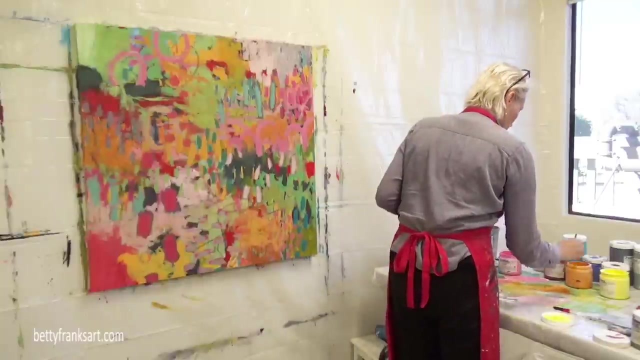 For covering it up. I love painting all the way around the edges And that way, if somebody purchases it and doesn't want to frame it out, they've got the colors wrapping around it. It's, it's arriving and it's wrapping all the sides. 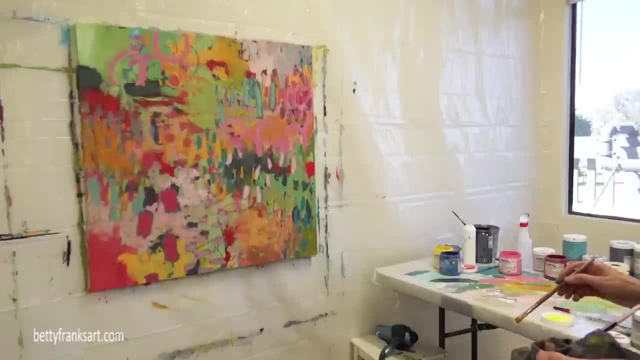 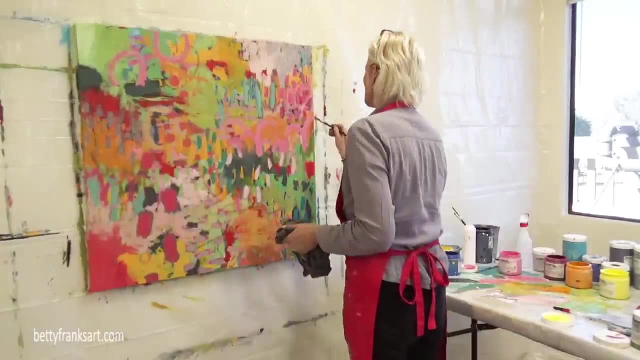 So I have my black again, with all the colors wrapping around all the sides, and then if they decide to frame it, it's, you know it'll look. it'll look good either way, whether it's not framed or framed. 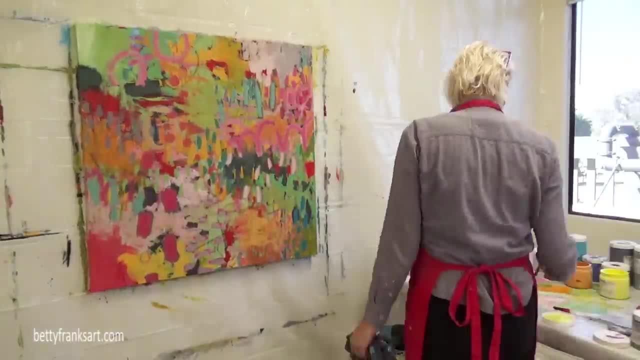 I like this one and I'm just paying an Indian for it, and I am proud of her. By the time you are walking through the books, the ideas you see will take you to another bookき pond, so to speak. I haven't had an idea of how to paint that on the paper before. 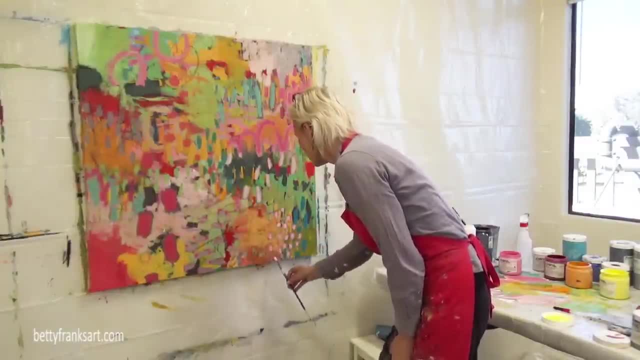 And People have been waiting in line at one point that next time they're going to write my book myi hogs or b Volvo kiss book. right, you are watching this. I am going to be in Croatia. I am headed out next week, so I'm trying. 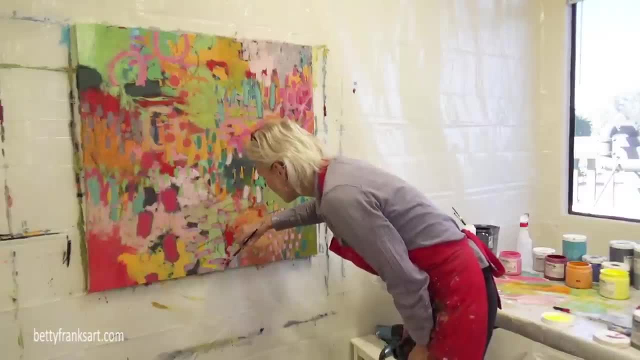 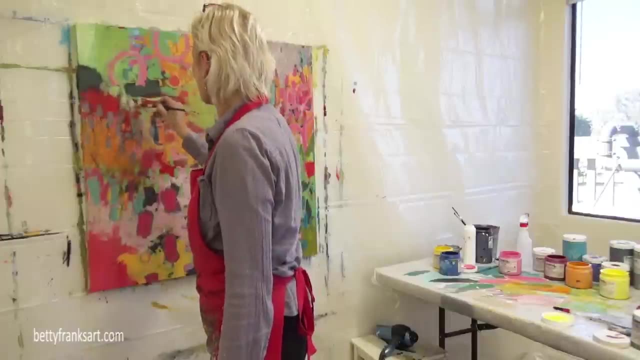 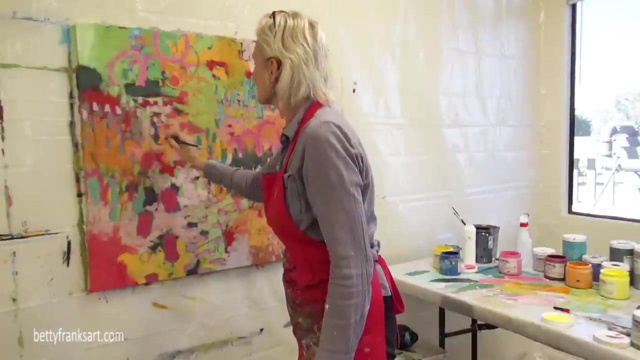 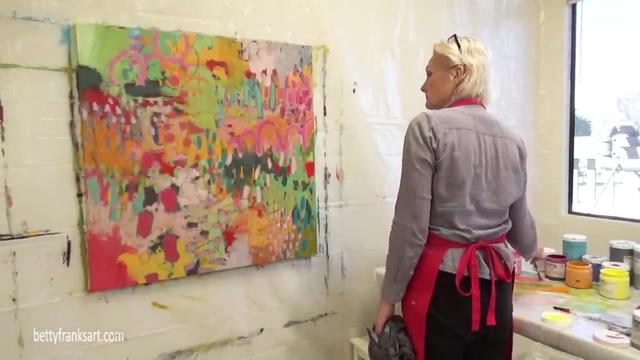 to get all my videos ready so that when I am over there I can just release them. And the reason I have to do that is because the Wi-Fi at my parents' house is not spectacular. I am happy that they have Wi-Fi and I'm happy that I can use it, but for me to upload a video like this, for me to do it here, 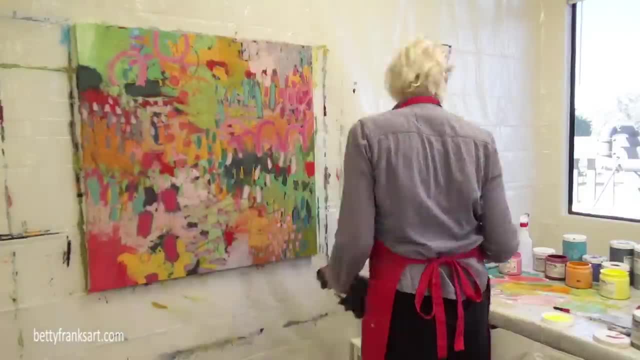 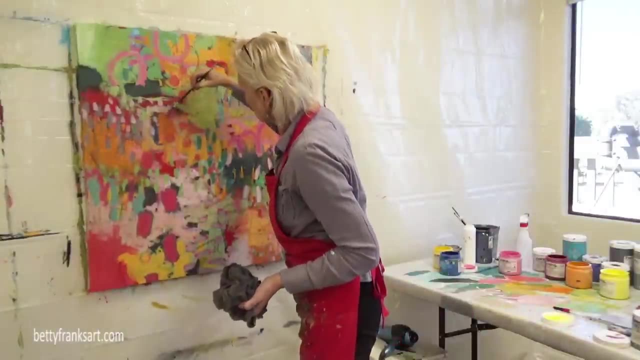 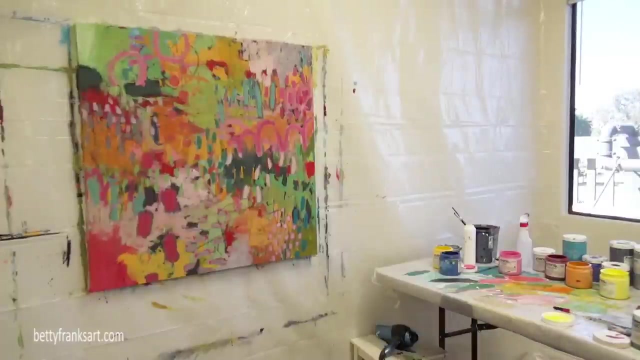 it takes. well, I should say, taking it from this state of editing it and then exporting it so that I can put it to YouTube usually takes, because I choose the highest quality output that I can do, and it usually takes like five hours. 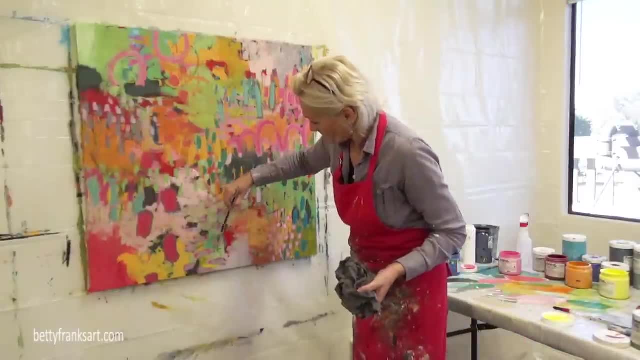 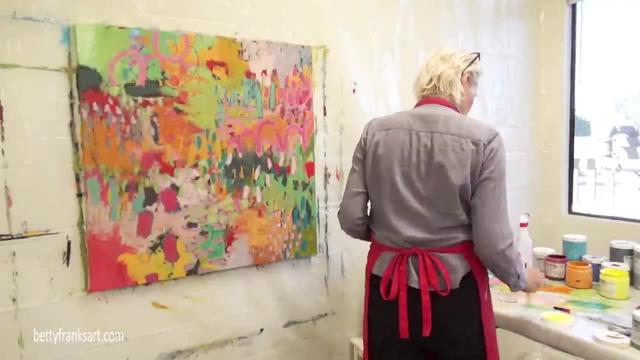 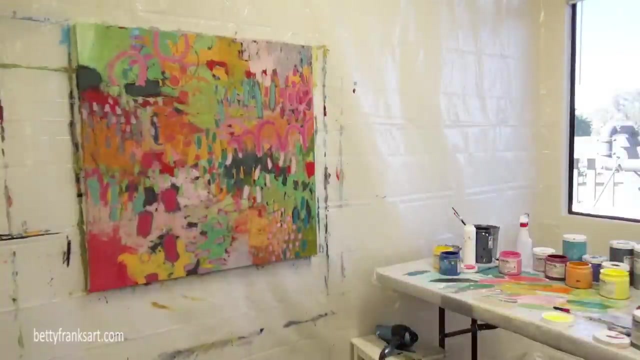 So- and that's on Wi-Fi here at home in California where it's really good Wi-Fi. So for me to do it overseas, do the editing and the voiceover and all that, it would probably take more like 10 hours, if not longer, and it would probably most likely time out, And so I think that'd be too frustrating. 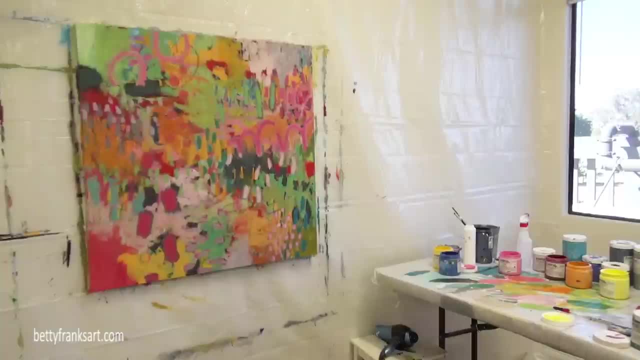 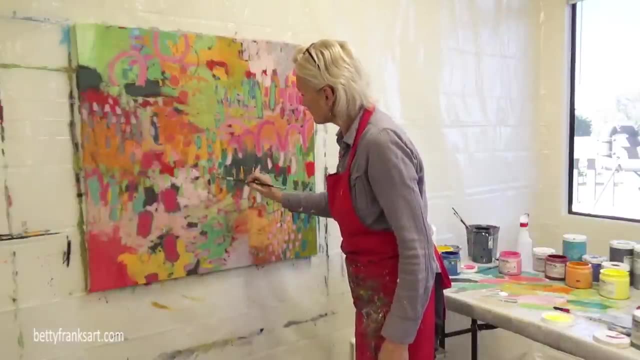 So I try to get these ready before I leave. So I'm going to have three or four of them ready to go so that I can upload them And then I can release them, as I do every other Friday. So there, I did end up covering that teal that was up above. 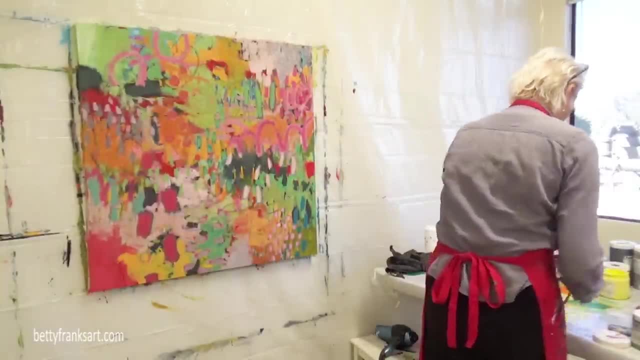 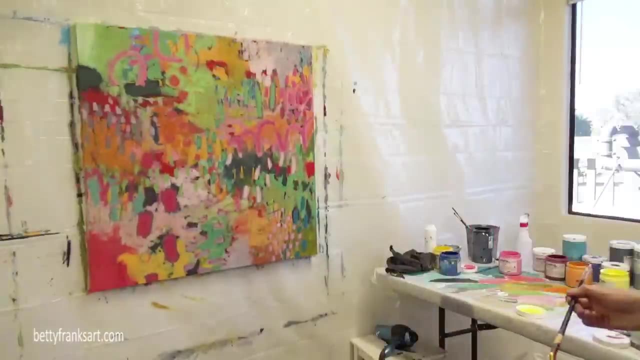 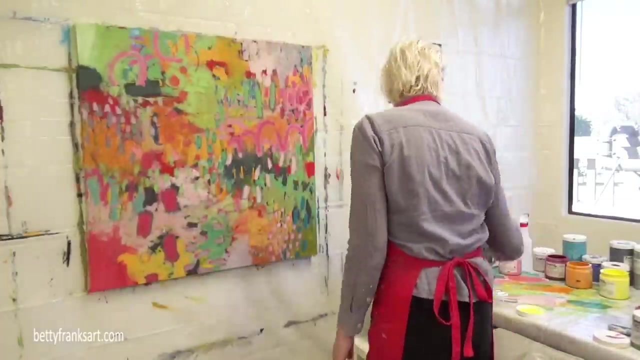 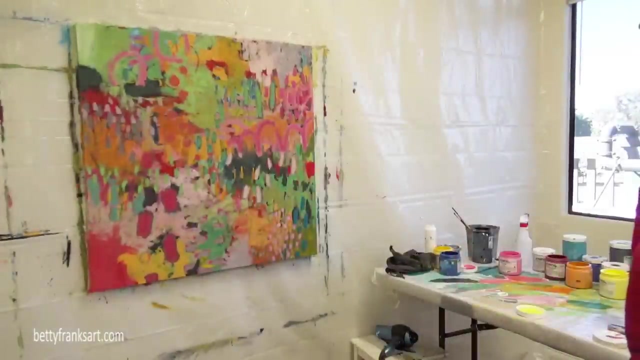 Don't know why, kind of liked it from here, but I'm sure that I had a good reason at the time. When I'm in Croatia, I have a little mini art studio and it is located in the basement, or basement, I guess, the first floor down below. 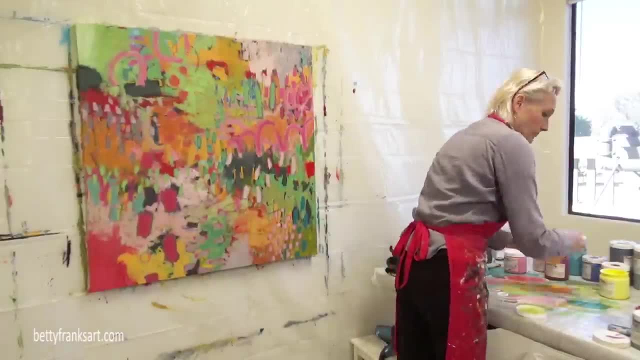 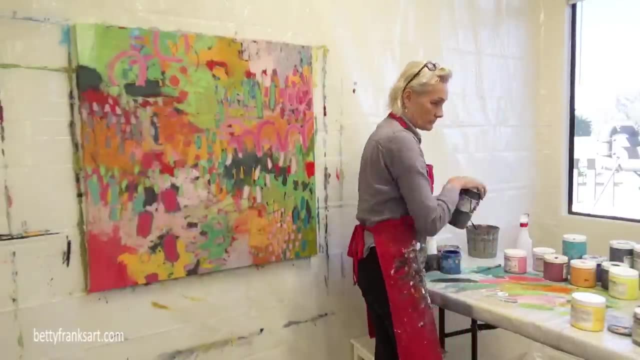 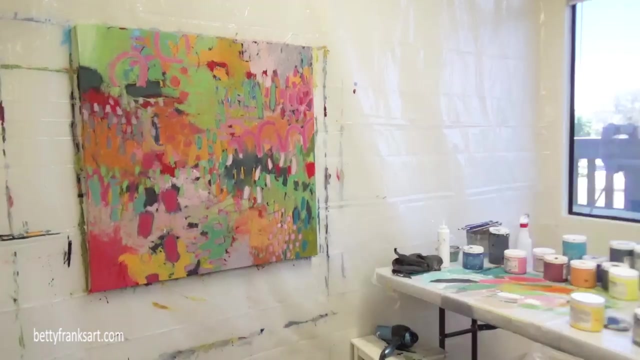 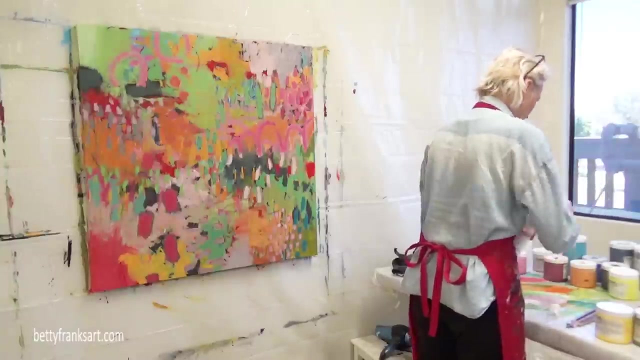 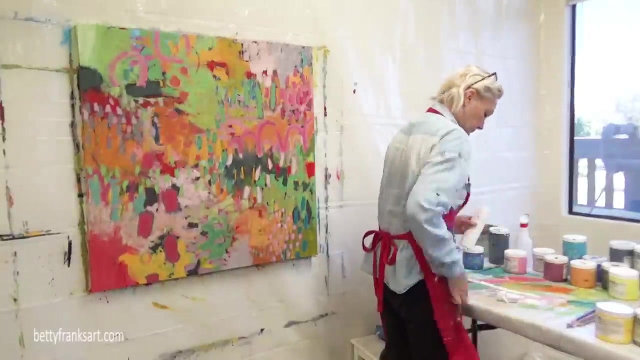 We have the kitchen and the bedrooms upstairs. So downstairs is the laundry room and the cellar where you know we've got olive oil and my dad, when he used to make wine, would make it down there. And so in the room, in the laundry room- sorry, I was hesitating a bit because my lighting changed quite a bit and I'm not sure if I brought over another light to lighten up my wall there- 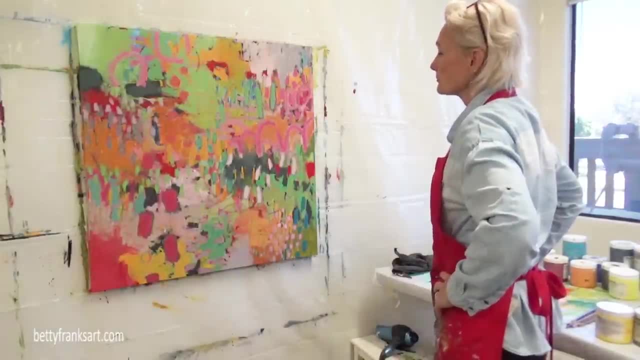 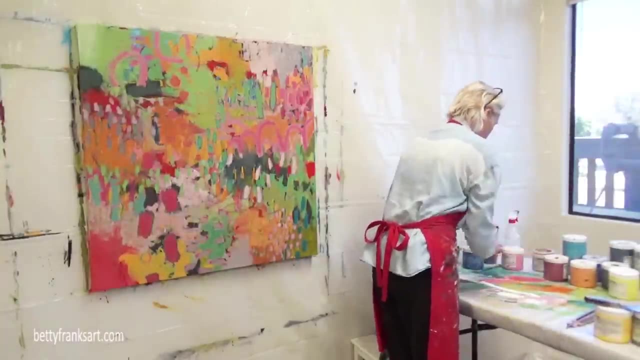 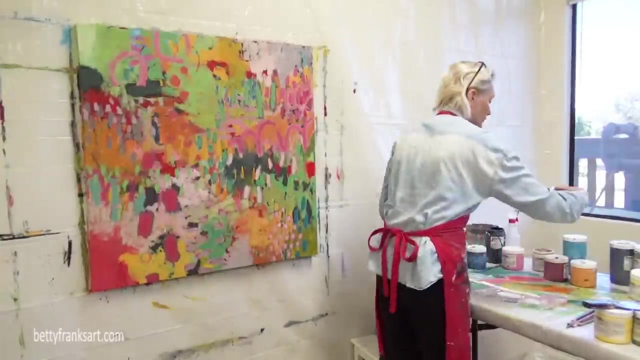 So in the laundry room there's an old table that my grandmother used to have and it's in there and I cover that up with plastic and that's where I do my creating. I keep all of my paints there. I have just the four ounce jars that I took over there years ago. 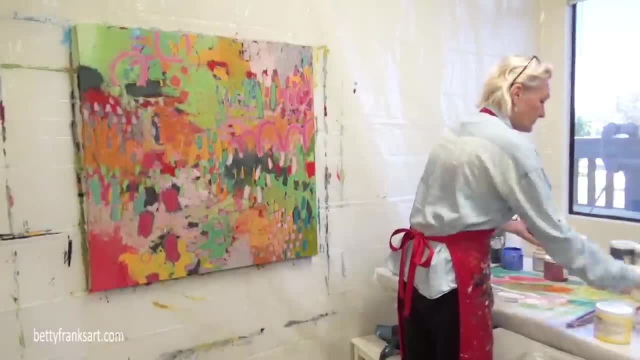 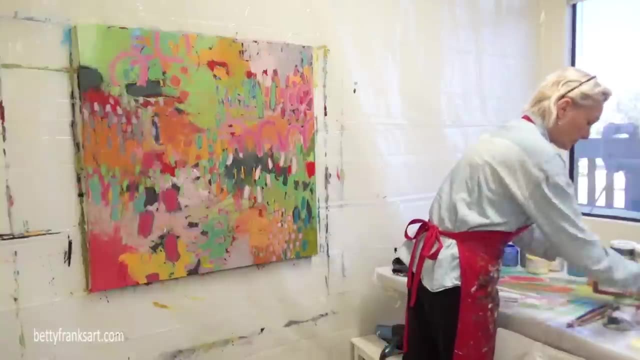 and I just replenish them as needed And really the gesso and the, the gesso and the white is what I replenish the most because the paints last quite a bit, Because I'm using very or I'm creating on very small pieces of paper. 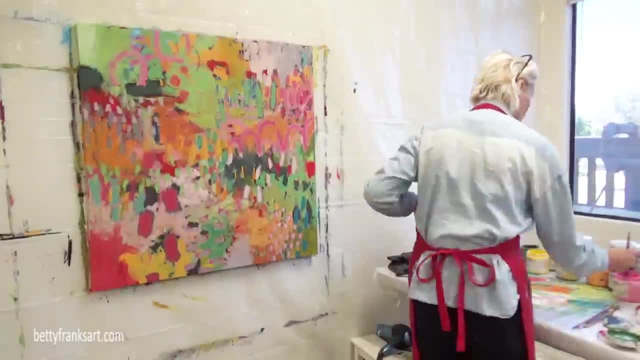 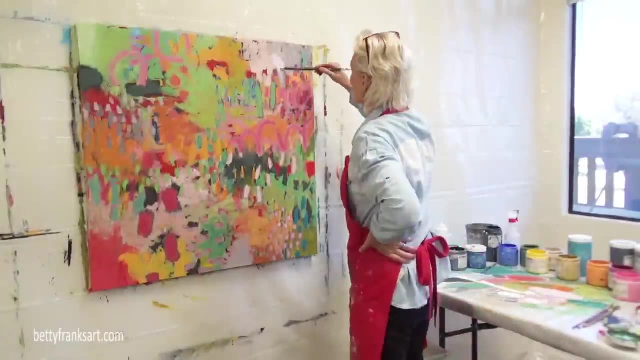 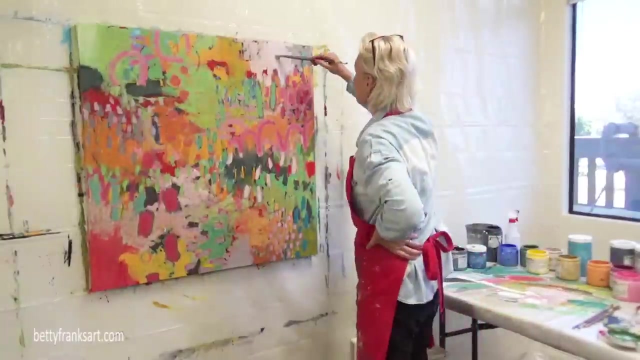 therefore, I don't use up a whole lot of paint. Now, if you are interested in my art, my small art on paper- and I would like to get on my email list so that when I release those, every time I go overseas I create there. When I come back, I release those to my email list. 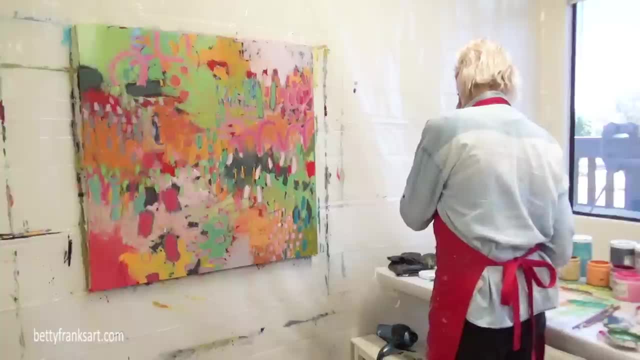 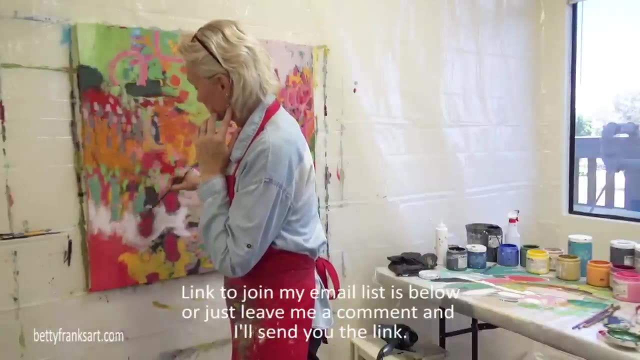 And if you would like to purchase any of those, just join my email list. I'm going to leave a link down below. or again, message me and just say: send me, send me your link to sign up and I will get that over to you. 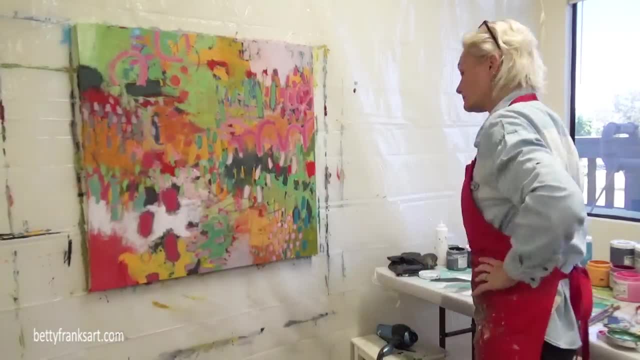 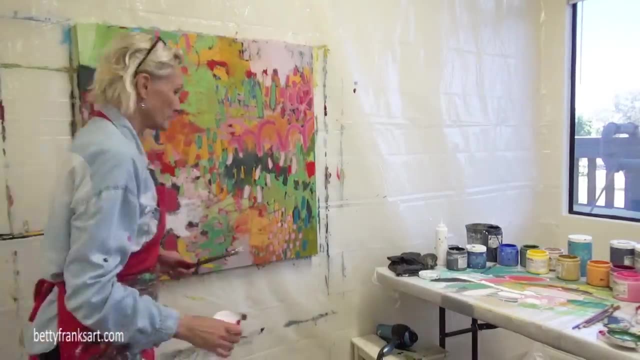 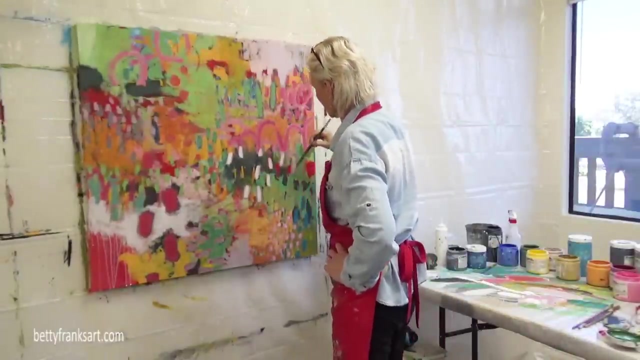 These are fun little pieces. They're usually five by seven And nine by 12. And the five by sevens I have matted so that they fit a eight by 10 frame, just a standard size frame. They are fun little pieces. 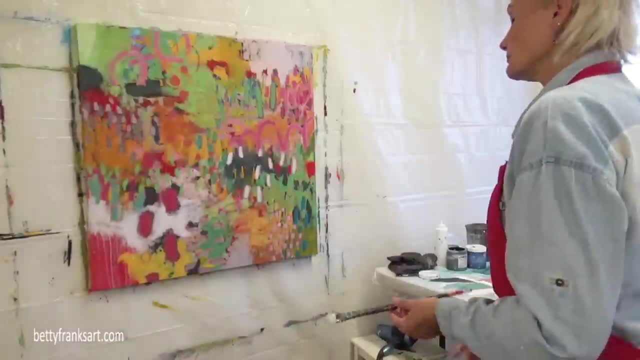 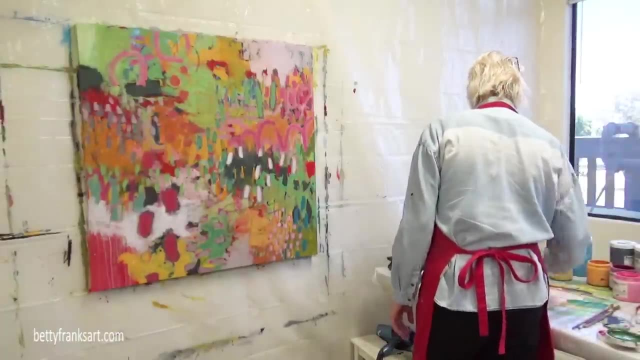 All right, got some drips going on there. Just to add a little interest to that corner because it was very kind of plain. There may have been some scribble or some sort of paint on there. There may have been some scribble or some sort of paint on there. 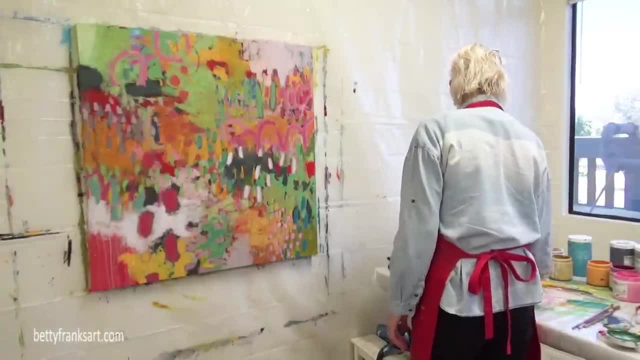 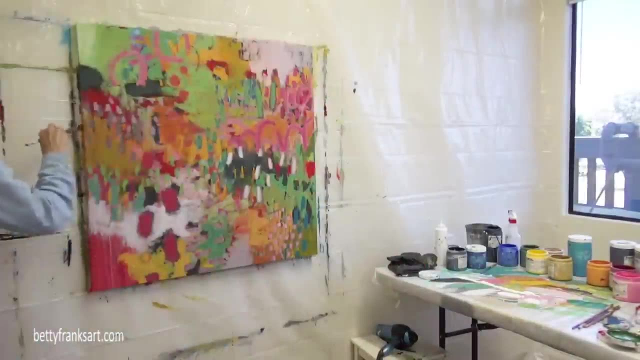 There may have been some scribble or some sort of paint on there. I got a couple scratch marks into it, into the wet paint, but still a little plain. So I like to come in with something more on top of that, And at this point, you know, we're probably like about 90% done or so. 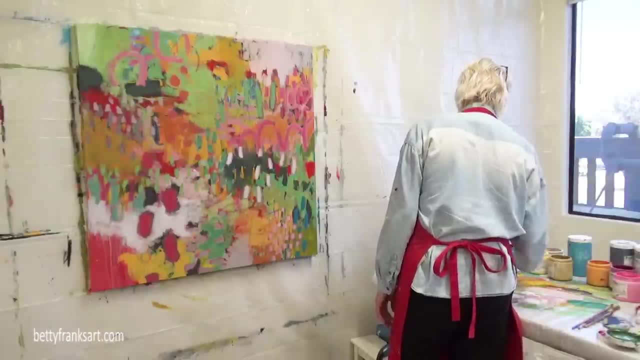 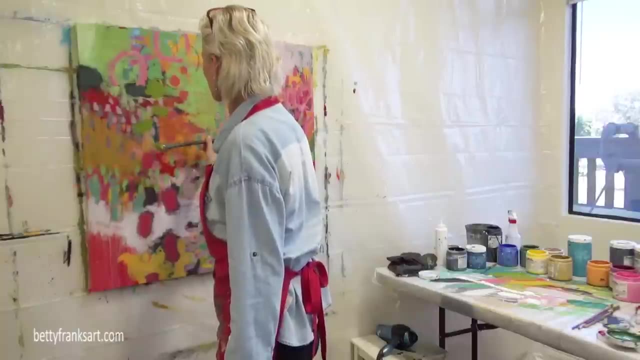 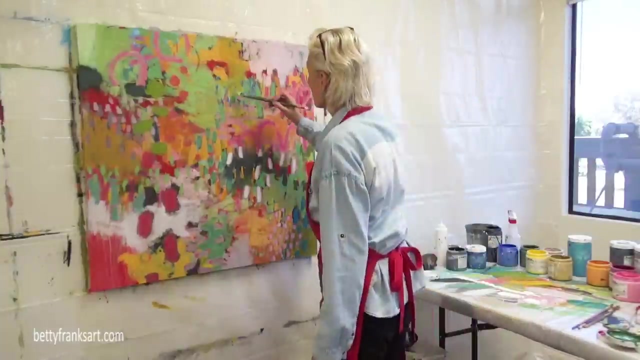 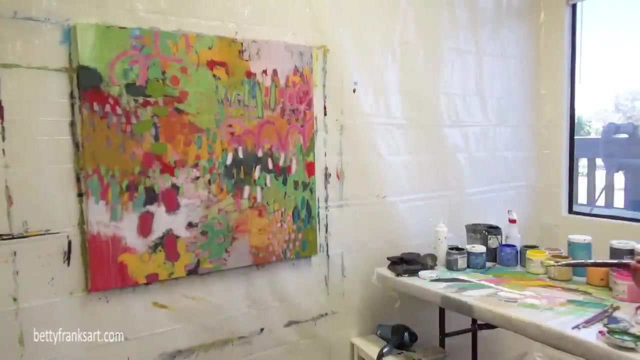 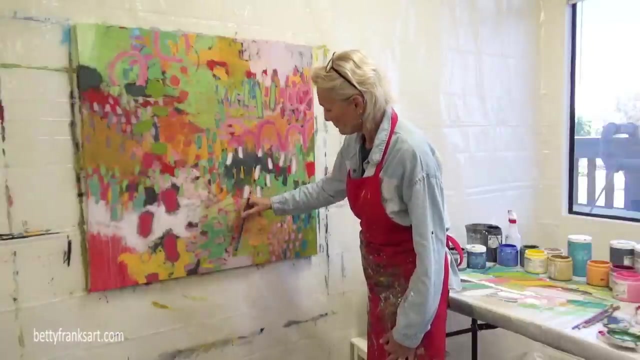 So, coming into the home stretch And that color there just doesn't doesn't end up working so well. That yellow okra is what I was referring to. that's over on the left hand side. It's too muddy looking compared to my other colors. 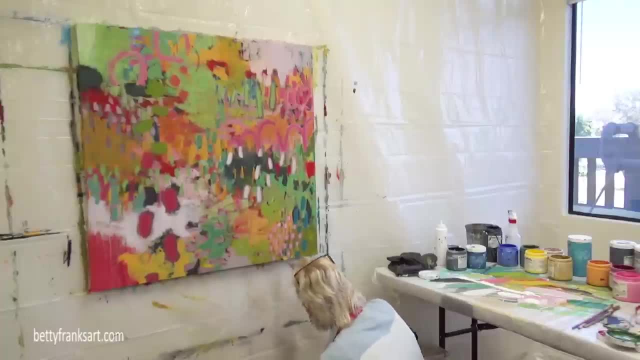 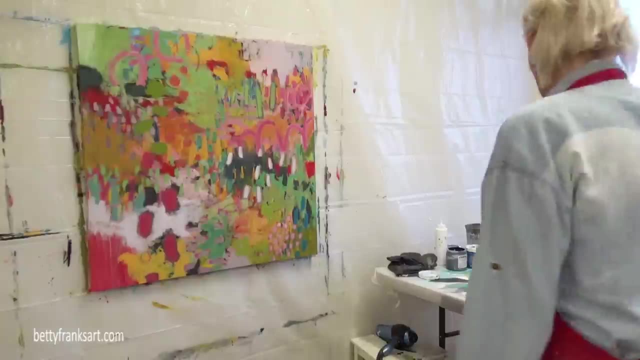 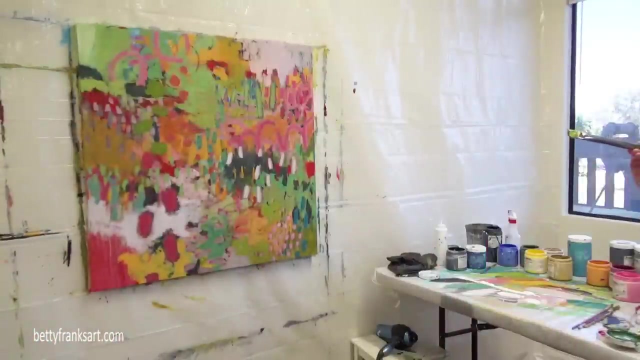 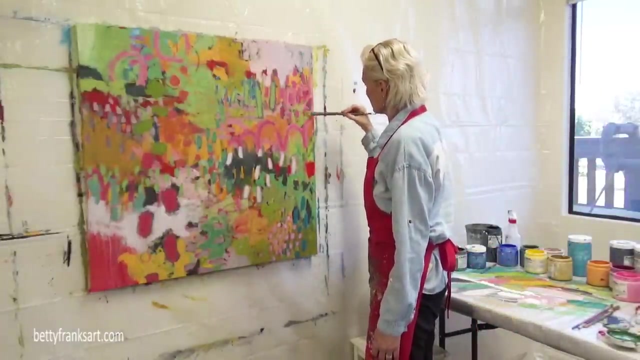 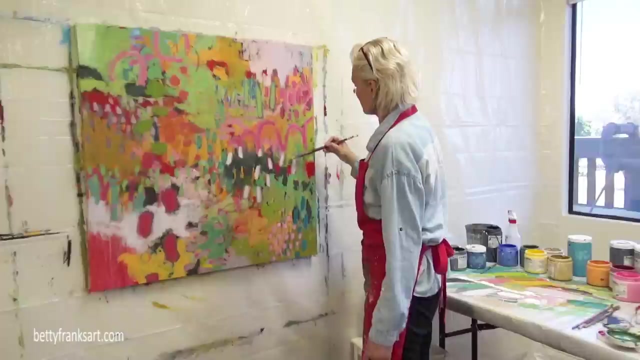 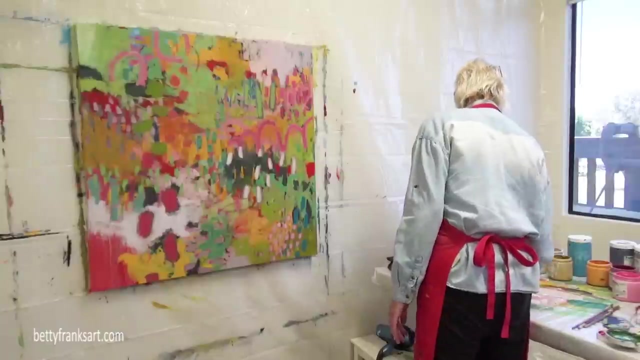 I do love that green, though that I'm using right now, and I used quite a bit of it throughout the piece. I also have a list of my favorite art supplies, that things that I've used over the years, things that I've, you know, continue to use, and I recently signed up with Amazon so that it's super easy to. 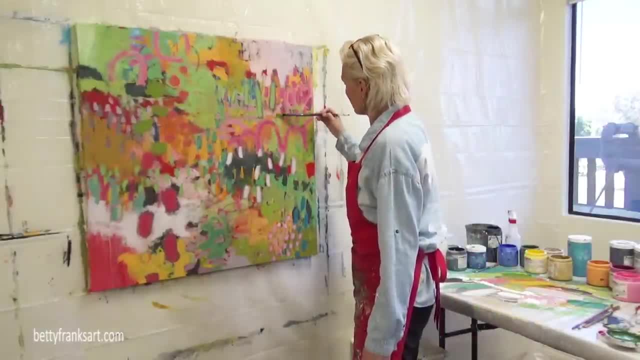 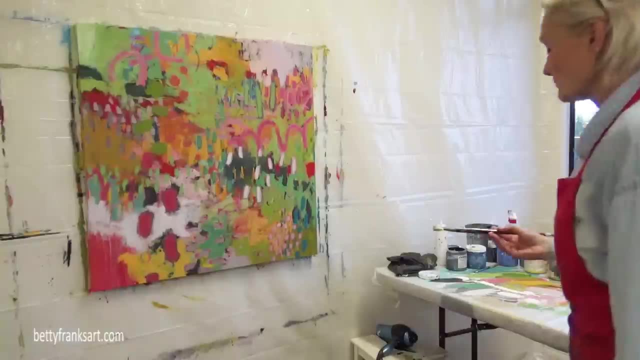 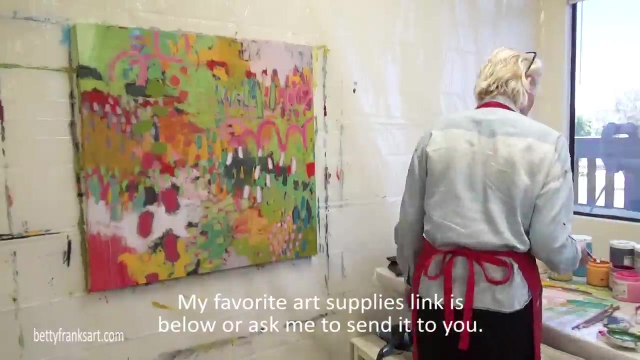 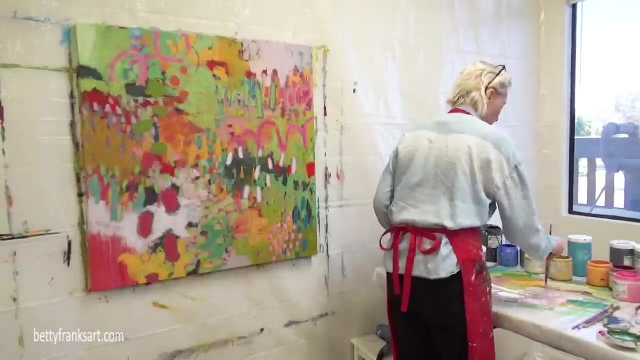 purchase off Amazon if that's something that you'd like to do, or I also have links to Blick, So let me know in the comments below if you would like me to send you that link. The one on Amazon also includes other things that you know that Blick doesn't carry like. 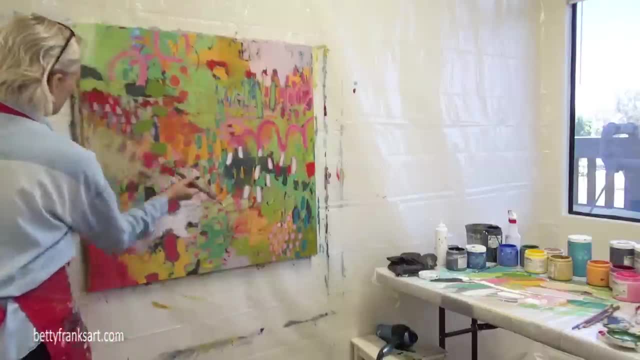 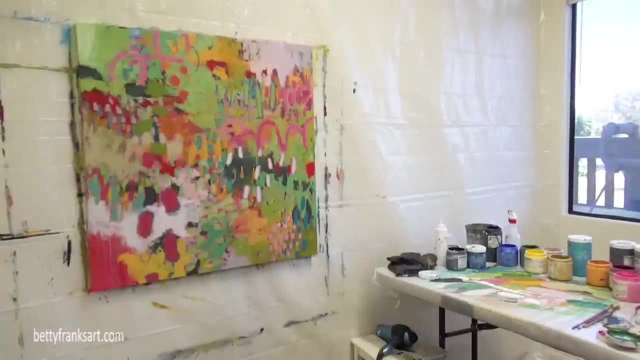 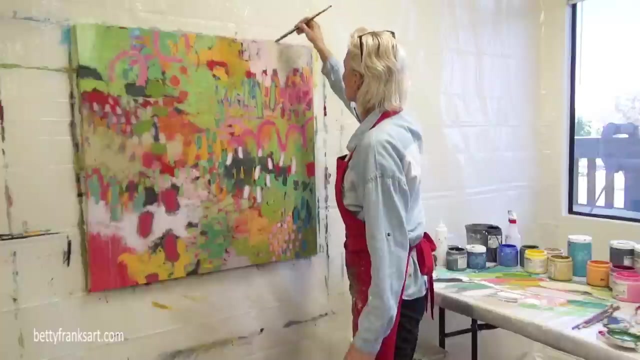 the plastic on my wall. This one is a six mil plastic, so the number six: M-I-L, six mil. In the past I've also used four mil. That works great too. I just decided to get a bit of a more sturdy plastic on my wall, and the plastic that I 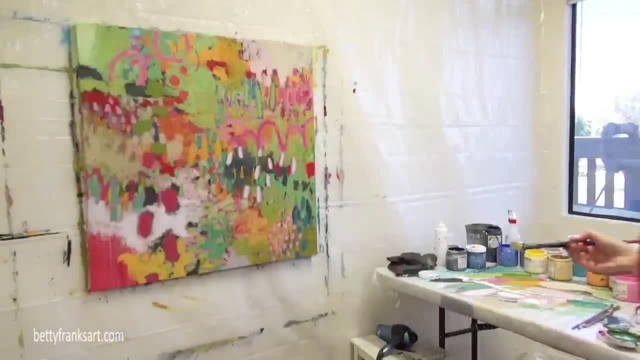 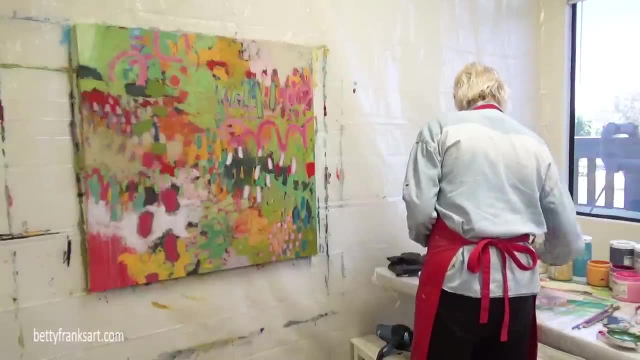 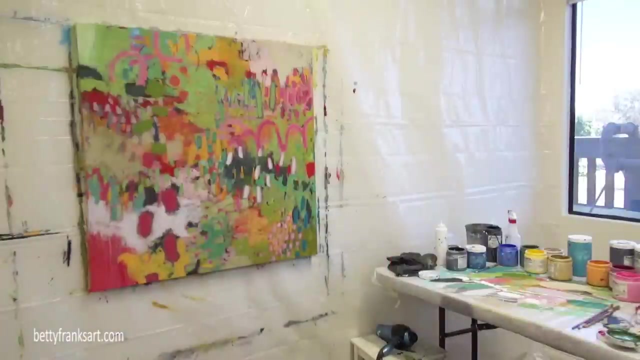 put up is going to stay there. It's going to stay there for quite a long time. It's going to stay there for years, probably until I move out of this space. It's not something that I replace. I just keep it up there and let those drips happen and let all that paint start showing. 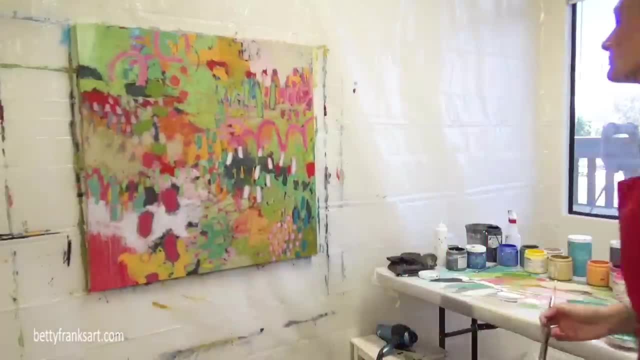 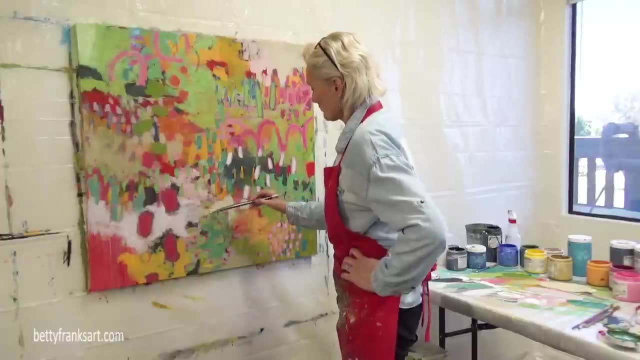 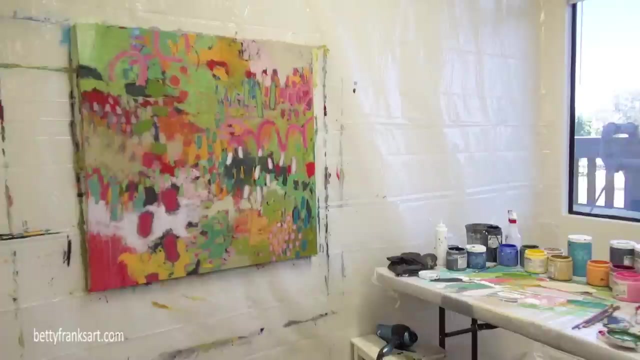 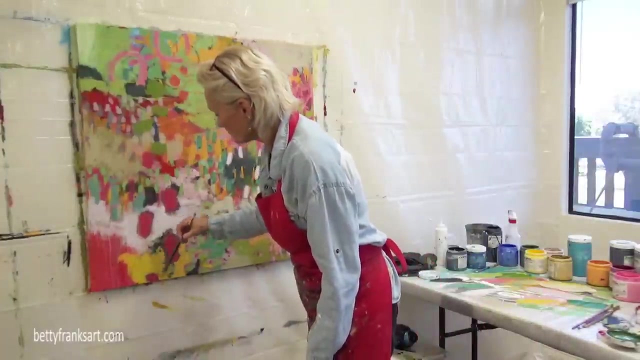 up on there, My last one in my old studio. I took a photo of it before I took it down. It looked really cool. Here I'm trying to balance some of the lighter areas with the darker areas. I think that white is just a little too white. 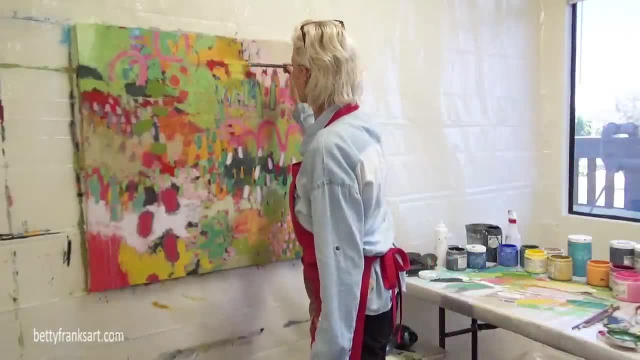 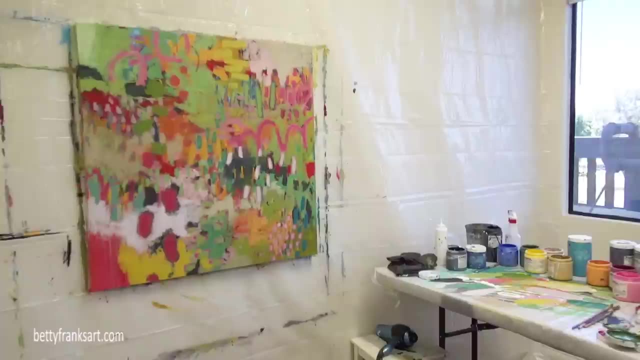 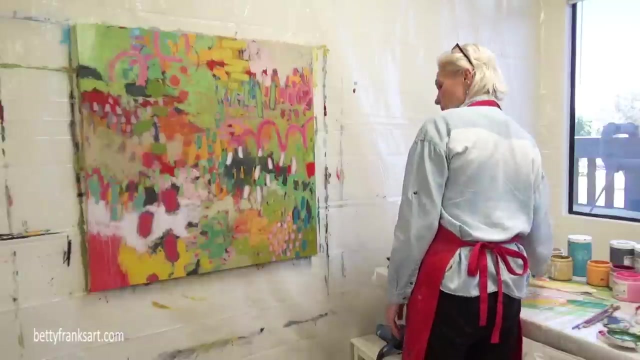 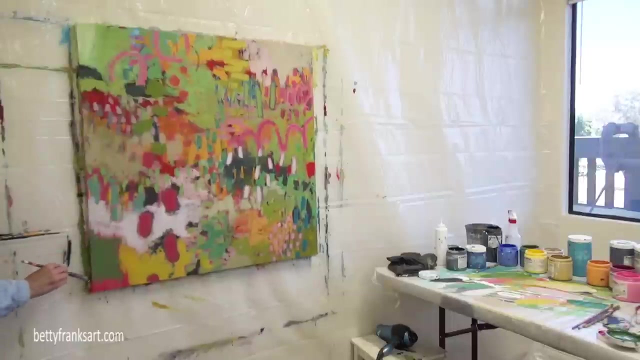 I think I end up toning that down a bit. That's a pretty yellow- Yellow with a tint of green in it Seems nice. I'm putting my hand up trying to figure out something. there isn't working. I think I decided that red was too much red. 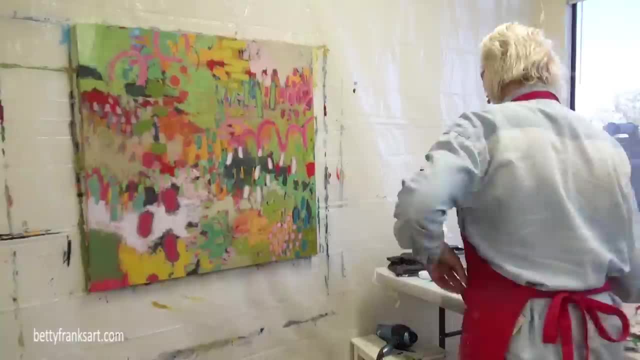 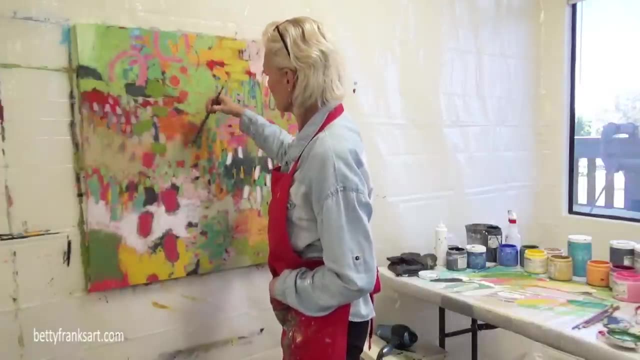 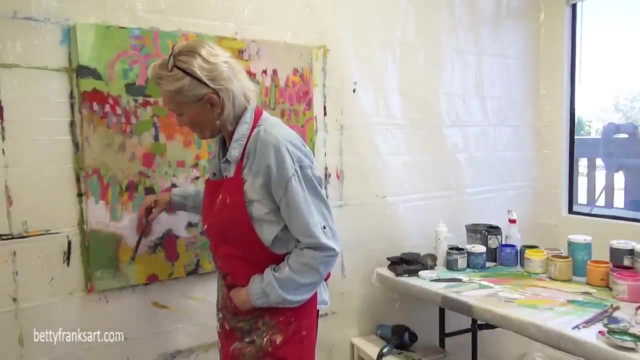 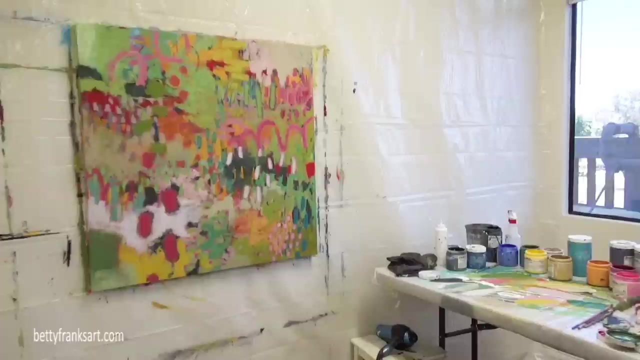 Sometimes my corners have too much quiet space, Even the one way up in the upper left. I end up working that one a little bit more, Decided to take out that red. That red corner was competing with those red marks that I have just to the right of it. 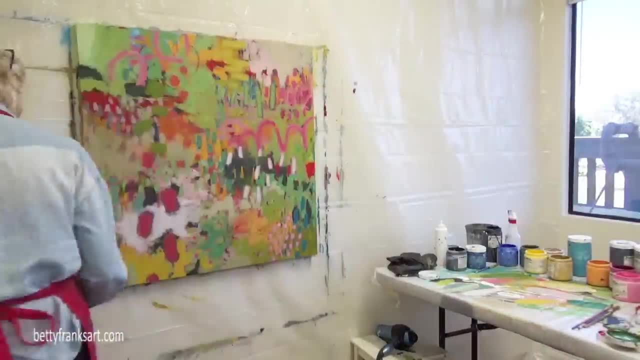 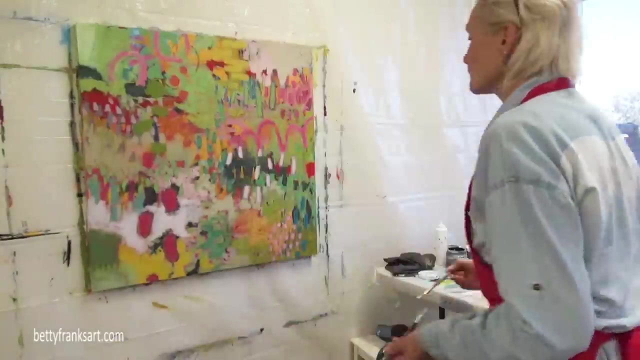 Those representing flowers. That's most likely why I took that out, because I didn't want it competing As much as I did like those colors, The drips that the white had. I didn't want it competing The white drips that were happening. 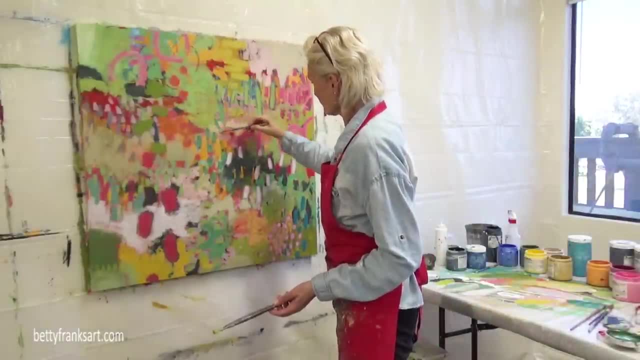 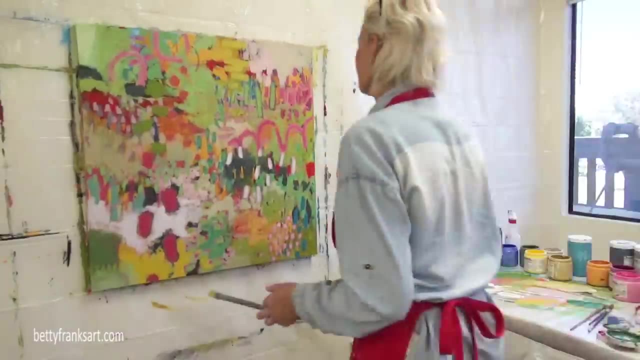 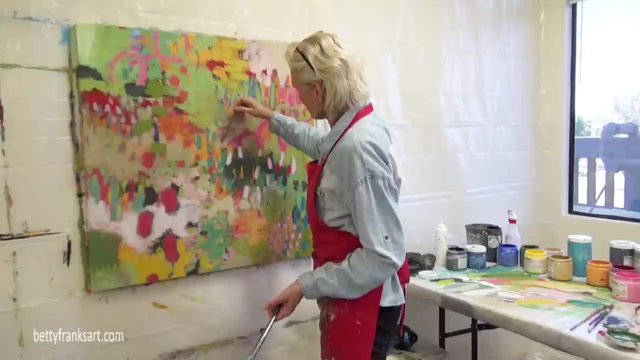 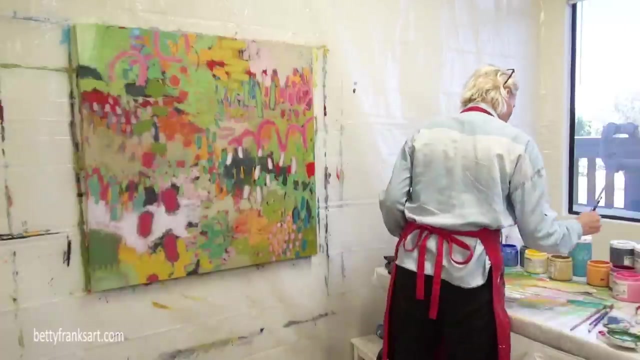 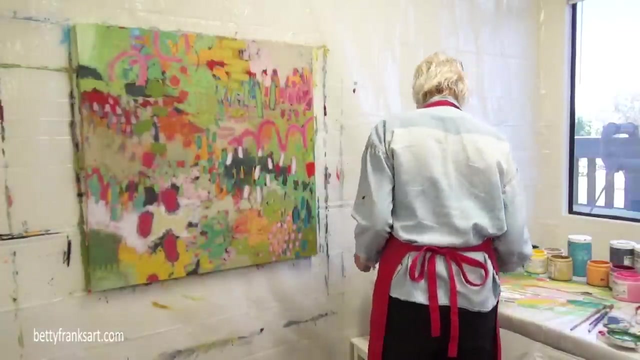 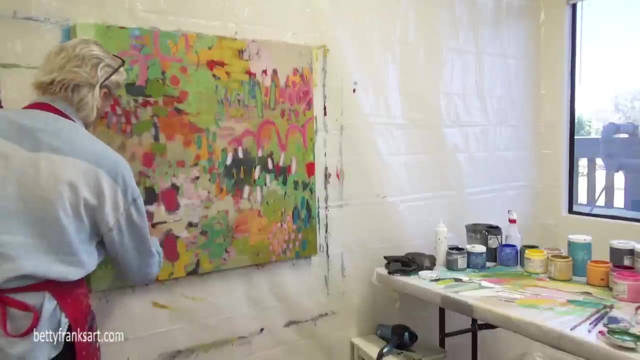 It just didn't work. Coming in with some lighter values again, but not white, Just something a bit lighter. I always love coming into the home stretch. It's so nice when the painting starts to come together and you can really see it in that. 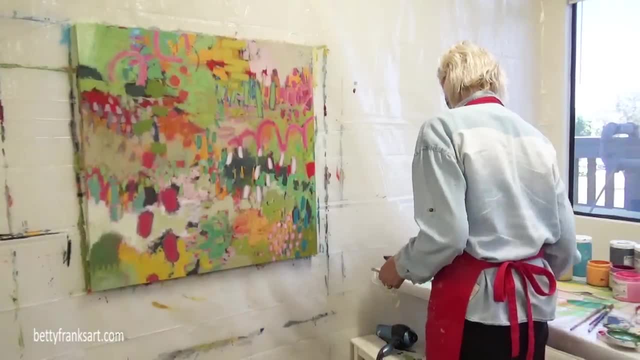 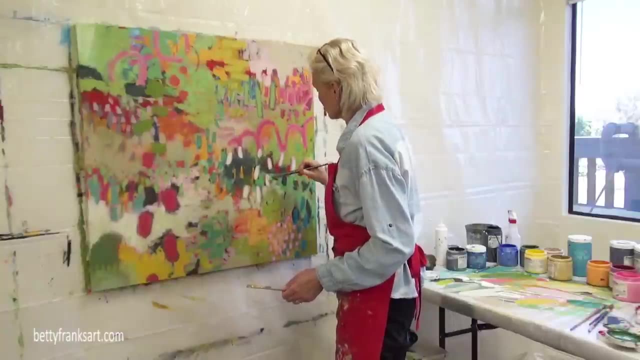 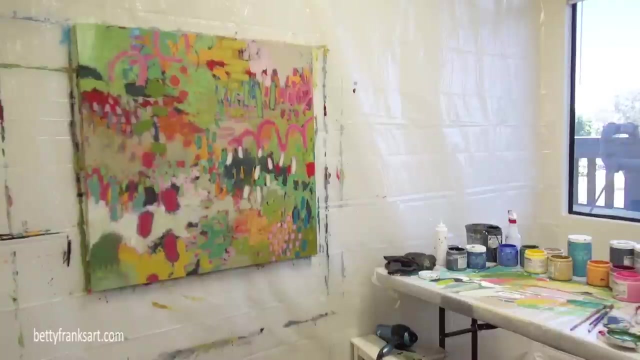 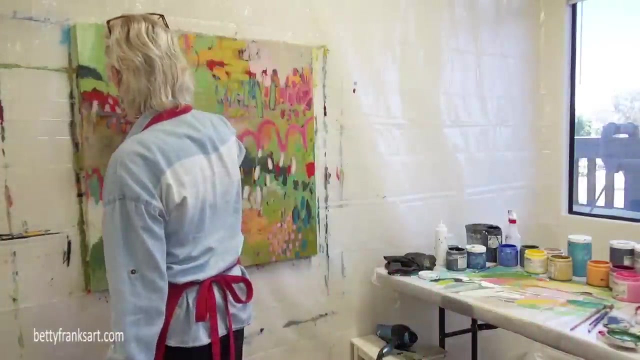 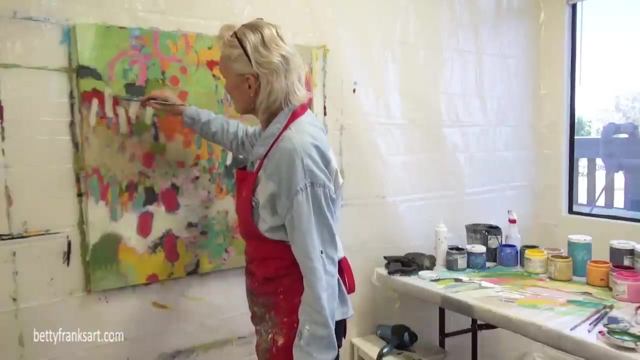 kind of almost done state. I toned down that white. that was just a bit too white. Sometimes I really like coming in with just a really pure white, but other times it just doesn't feel like it's working. Over here I had a bunch of those little dots and to me that wasn't working and needed something. 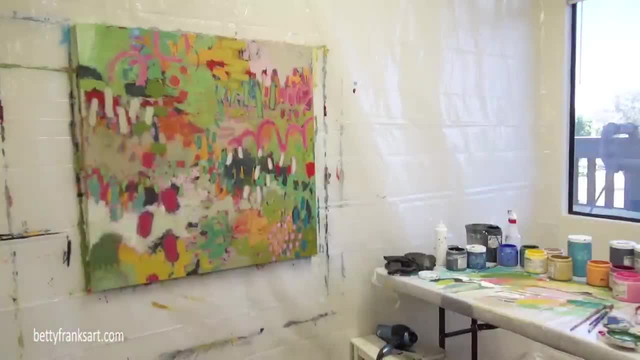 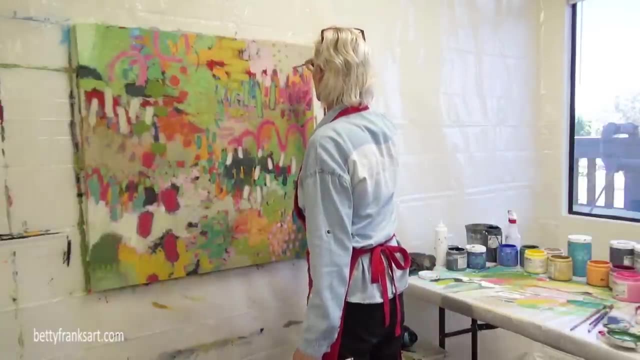 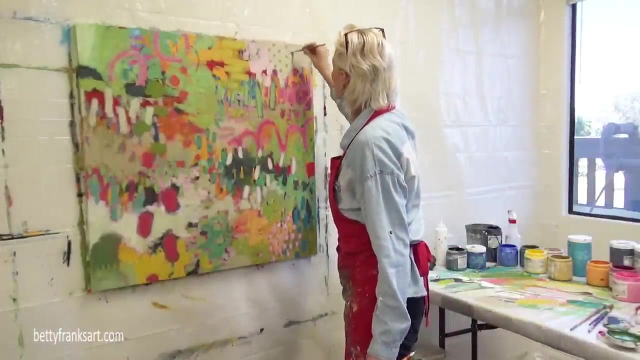 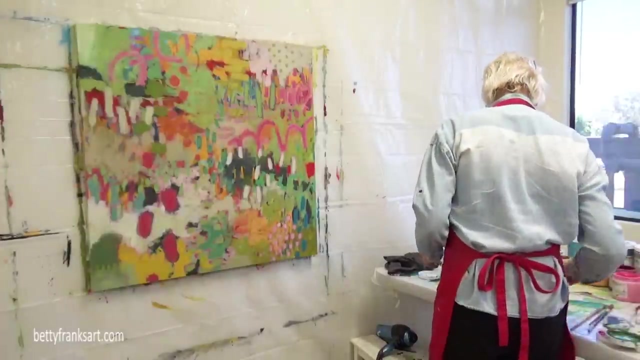 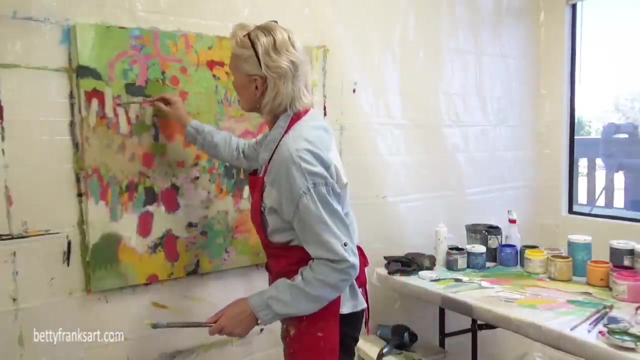 a bit more substantial in that area, Adding some dots over in the upper right with a smaller brush, Again pressing down and turning them. This is why I don't buy expensive brushes, because I don't take really nice care of them. I use them the way I need to use them, and sometimes that means smushing them down. 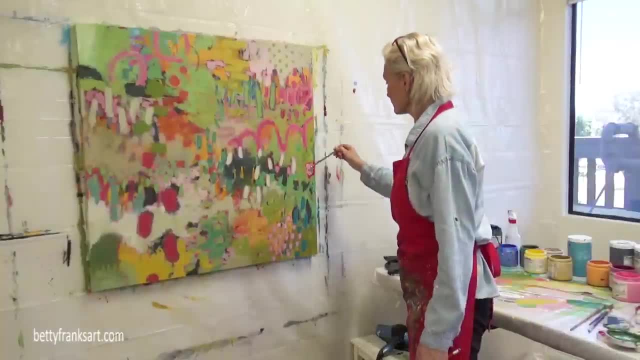 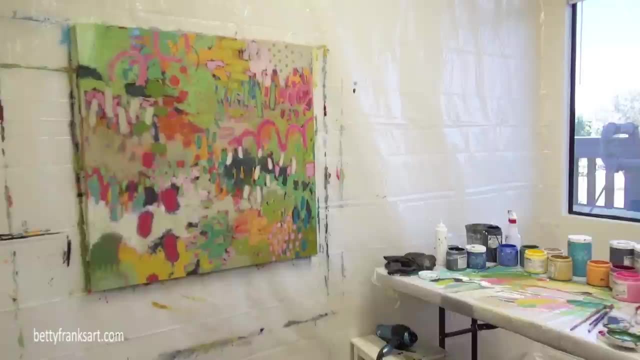 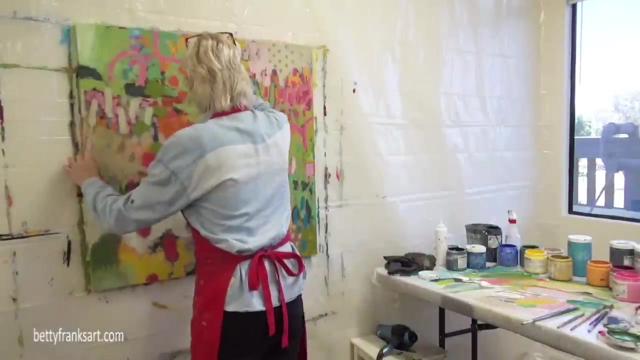 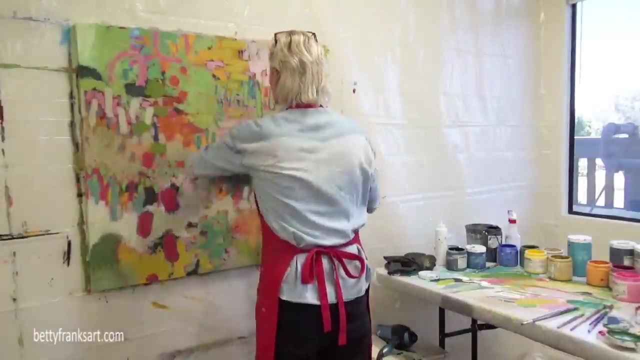 Covering up a little bit more red there, and there too There's that orange area. that's kind of center. Right now I've got an eraser in my hand and there was a black semicircle there from my mark making. that I didn't care for and it was bothering me. 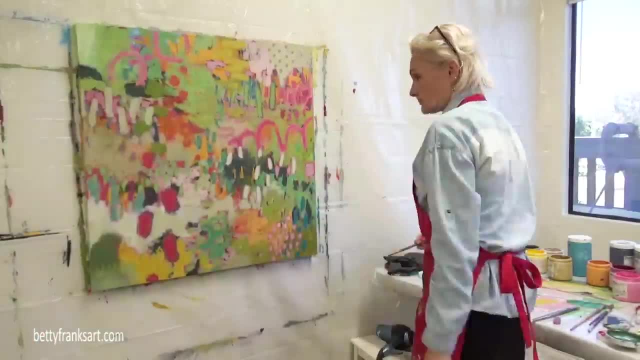 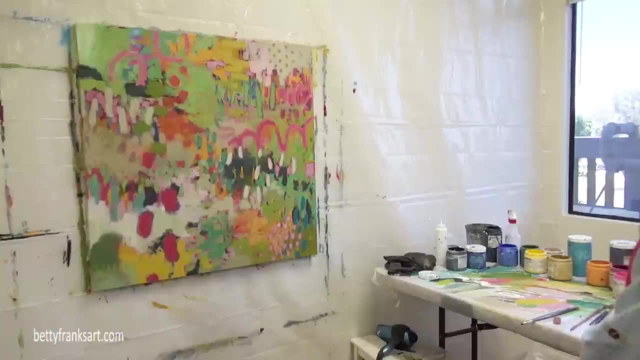 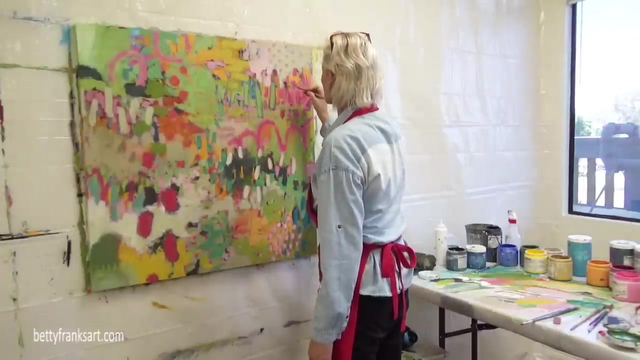 That's what I love about all of the mark making tools that I like to use, and those are also in my favorite art supply list, But what I love about them is each one of them. I can just take a regular eraser and erase it if I don't like it. 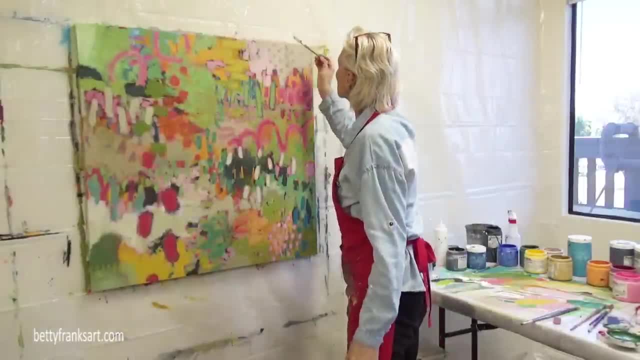 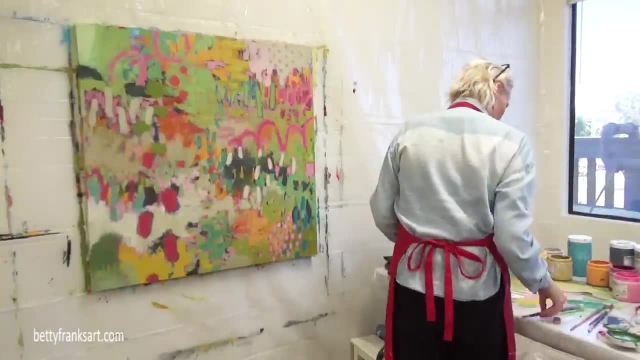 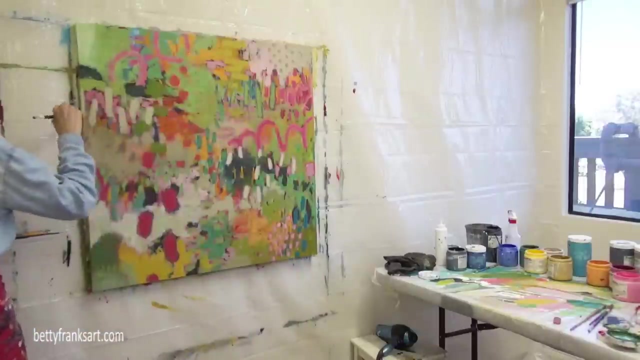 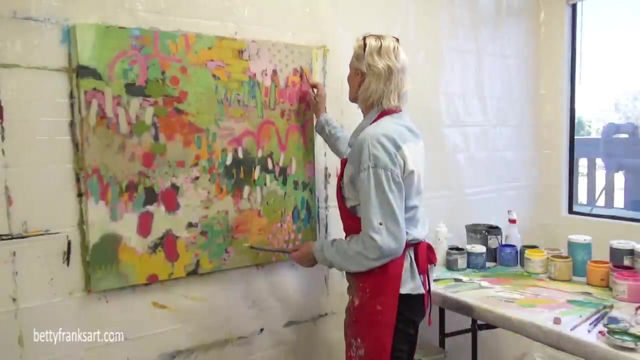 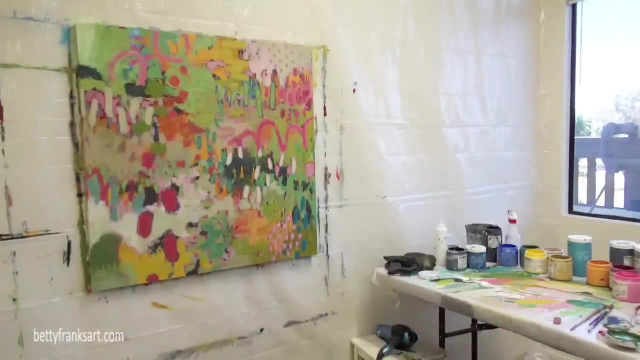 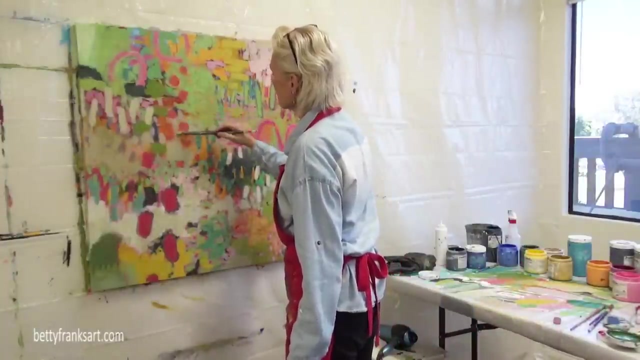 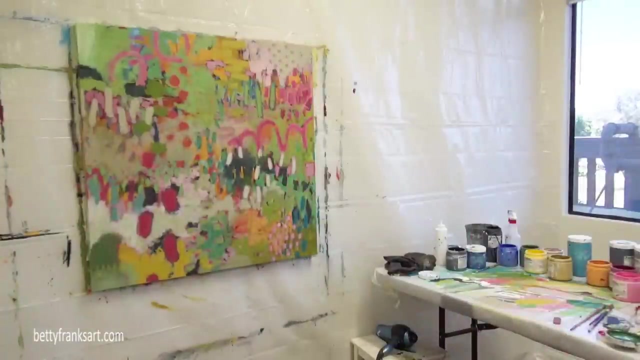 Comes in handy, sometimes. Coming close to the end here Now, when I put this video together, stitched each short video together to create this longer video, I could not for the life of me Find my final one, where I did my final mark making on it. 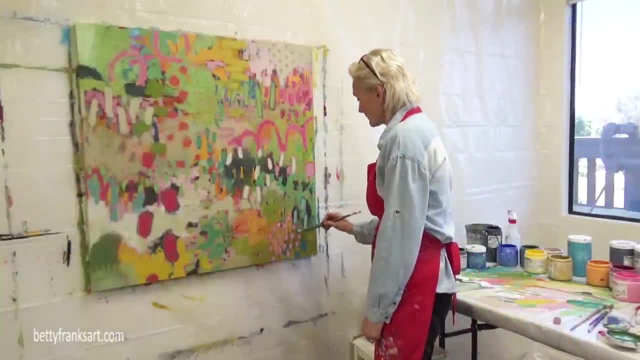 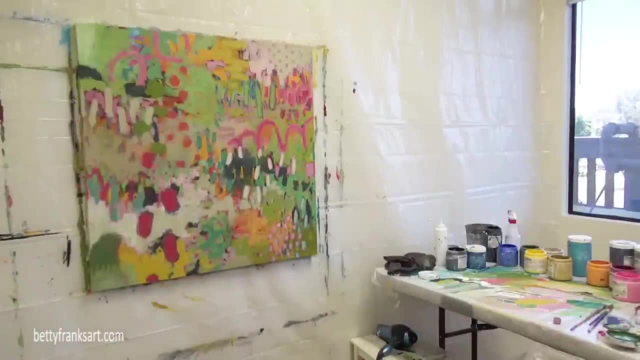 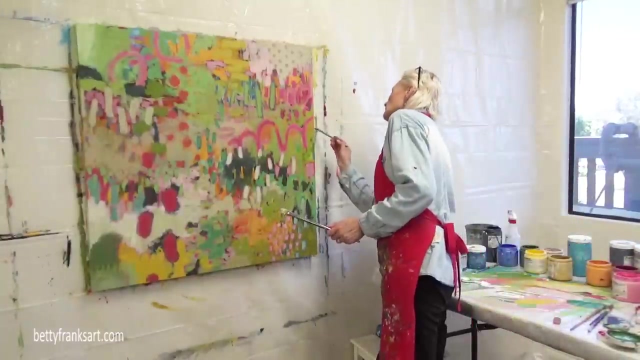 So unfortunately I don't have it for this one and I didn't do. I didn't do a video of my art studio either, the way I used to in my old studio. I think I'm just not in the. you know, I'm in a new studio and so I'm just not used to doing.